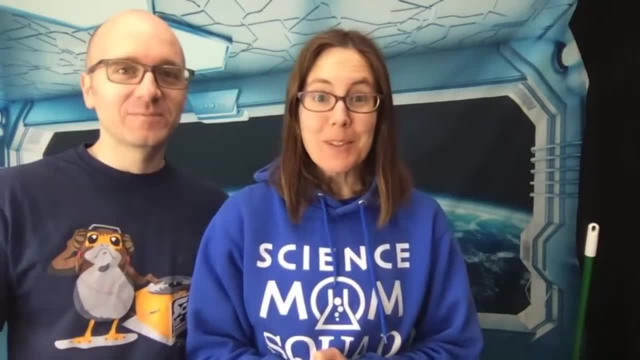 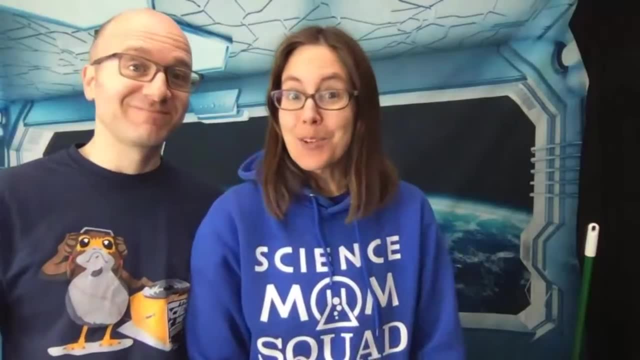 Welcome to Quarantine. In today's episode, we're going to be learning all about simple machines and about degrees and angles. I'm Science Mom. this is Math Dad. Special welcome to you if you're watching the replay And hello to Space Apollo. Joanna Queen Donut. Alyssa Nathan. 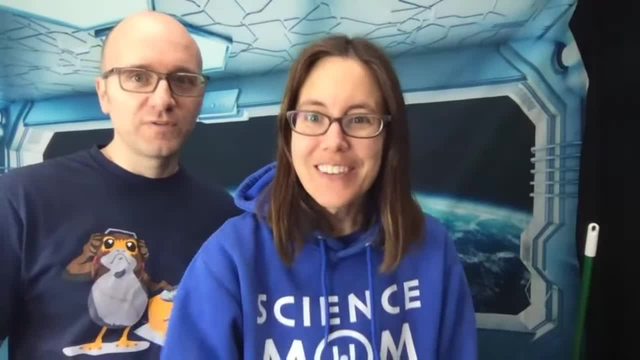 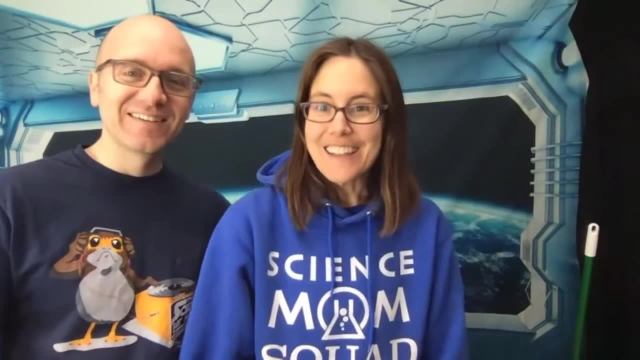 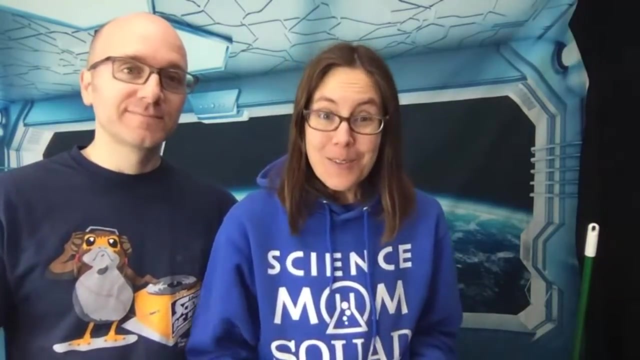 and Grace Gaming Wolf. Esther Ember Wolf, Girl 24. Science Mom Amber: Hey, it's Corgi. Science Girl Claire, Thank you for joining us today, And I see Emily said that she enjoyed yesterday's lesson about fungi. I had a lot of fun yesterday sharing with you amazing facts. 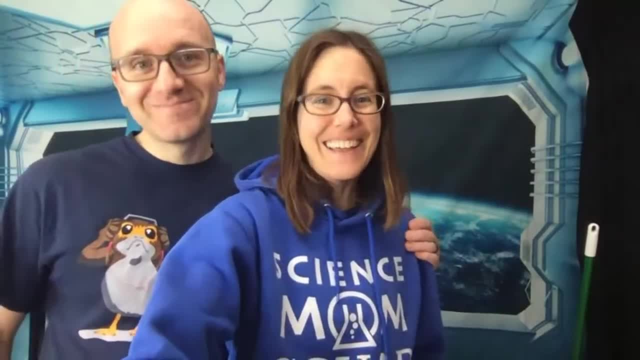 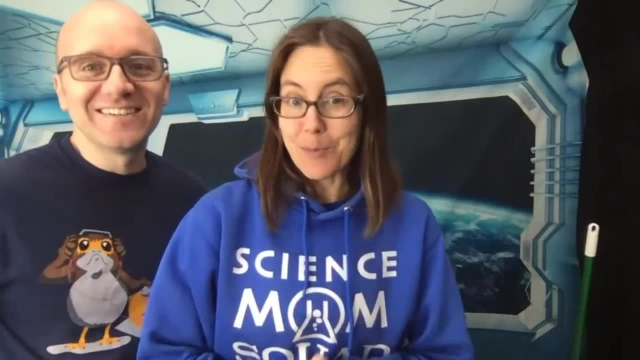 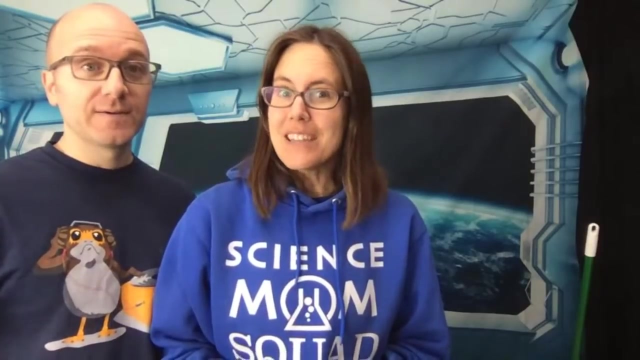 about the world of fungi as well. You're kind of a fun gal. That was a terrible pun. Now, today we're going to be talking about simple machines, And these are things that we use every single day. It's a super important part of physics And what we need to. 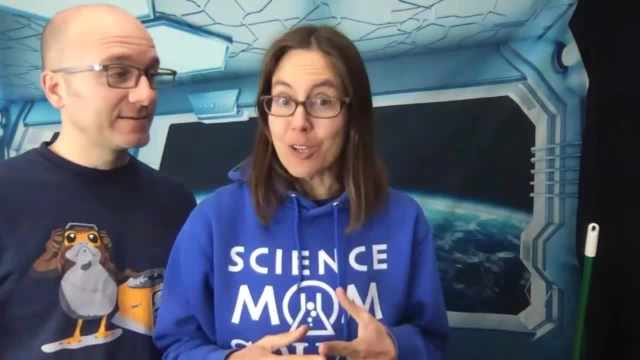 understand is that we need to be able to use simple machines And we need to be able to use simple machines, And we need to be able to use simple machines And we need to be able to understand is force and leverage. Those are two things that we're going to be talking about, and 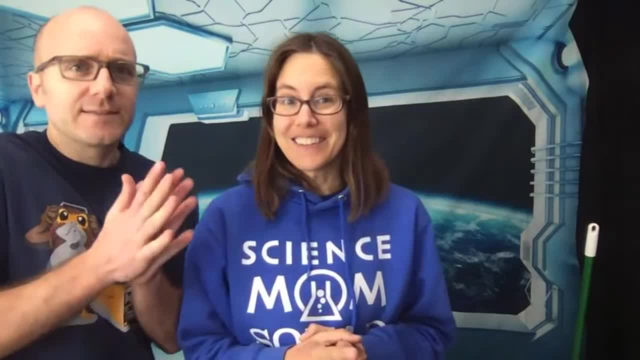 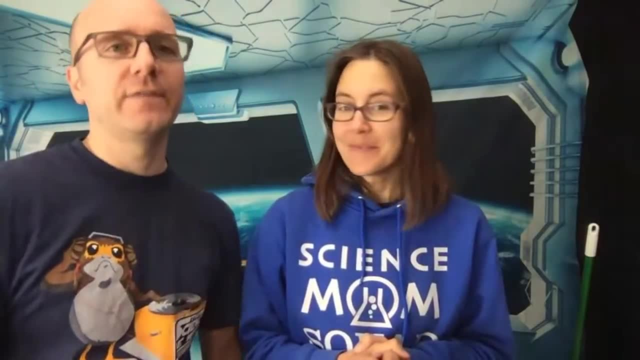 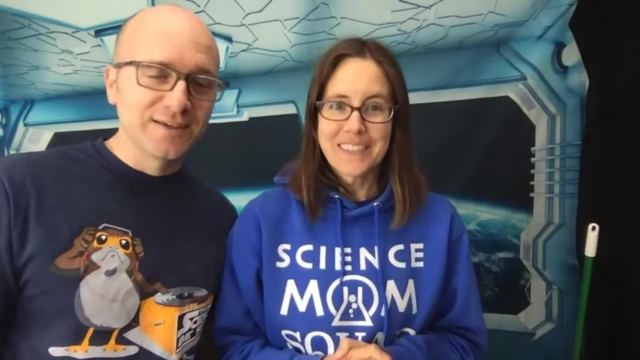 exploring today. I mean, let me just actually start off with a little story. We are building a wall in our backyard using these big landscaping bricks, And they're actually heavy enough that I'm the only one in the family that can reliably lift them and move them. So I bet you can guess who is. 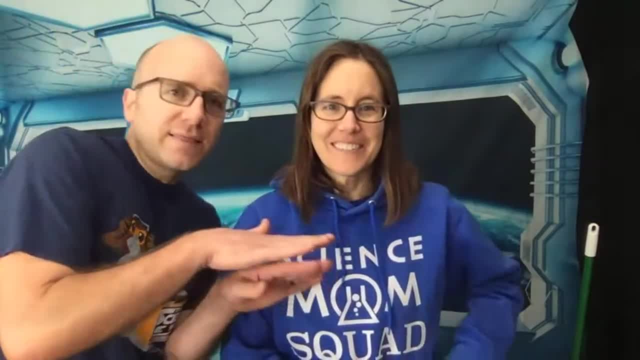 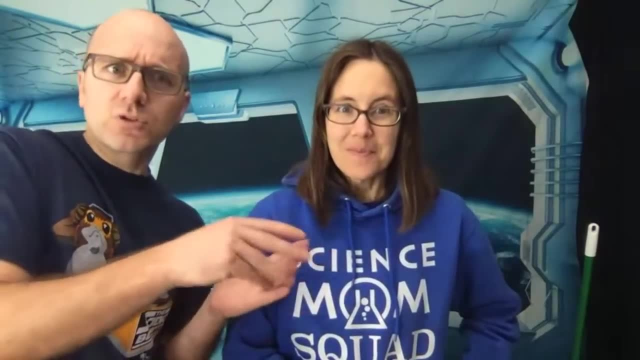 doing the bulk of the work here, But we had to get the bottom level- all sorry bottom layer- all level so that we could be able to stack on top of it. So that's the most work is trying to get that bottom layer level. I messed up Somehow. maybe it settled after I'd put it down, Or maybe 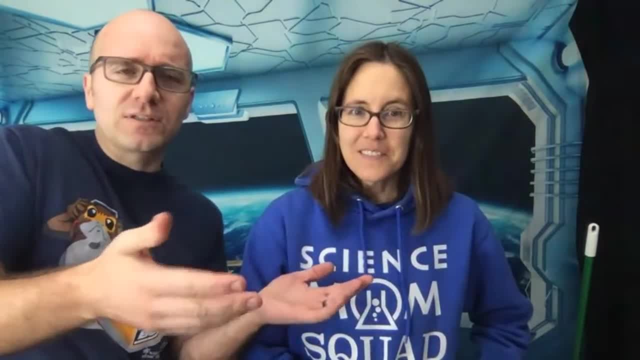 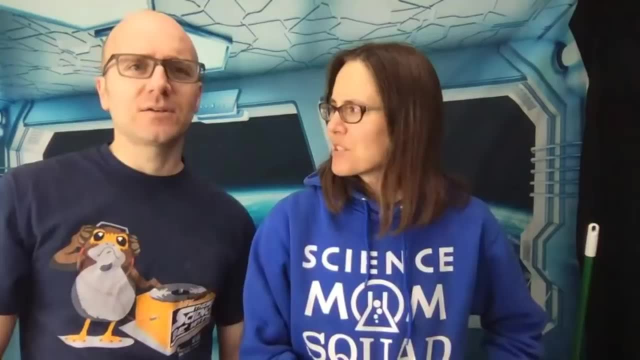 I just hadn't gotten a level in the first place. But when I went to do the second layer, there was too much tilt between them. And well, these are big, heavy blocks. How much do you think they weigh? Oh, I don't know. They're 50 pounds. 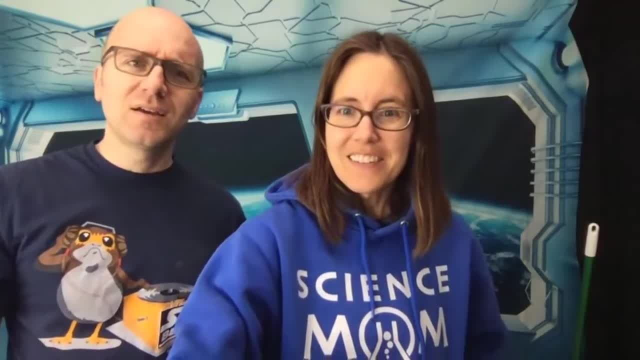 50 pounds. They're pretty heavy, Kind of awkward. It could be 70 pounds. Yeah, I don't know. I don't know They're they're. they're heavy, heavy enough that you guys weren't lifting them. 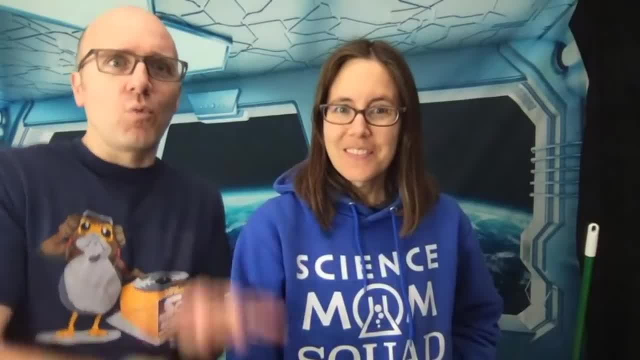 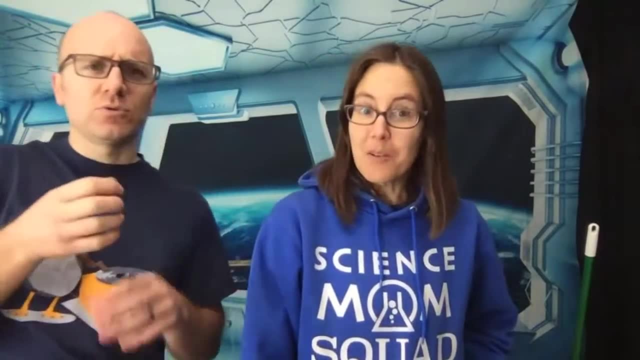 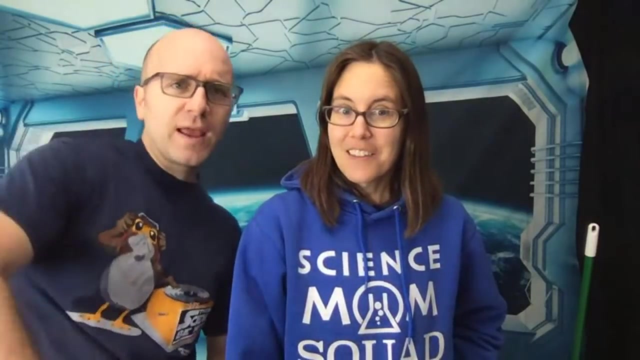 And anyway. well, I can't lift more than one. They're all stacked together. But we have this big, long rock bar. It's actually taller than me And made out of metal a couple inches thick. Well, we got this rock bar, wedged it underneath And just with one hand it's going to lift it up. 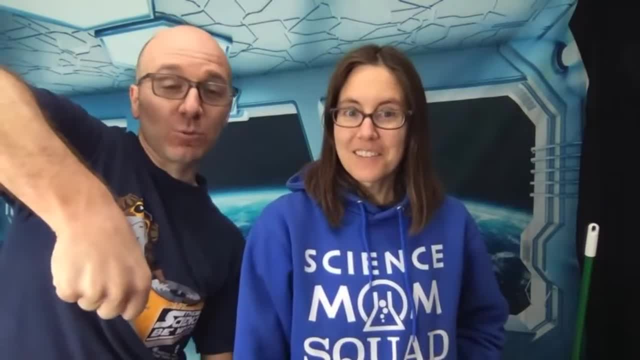 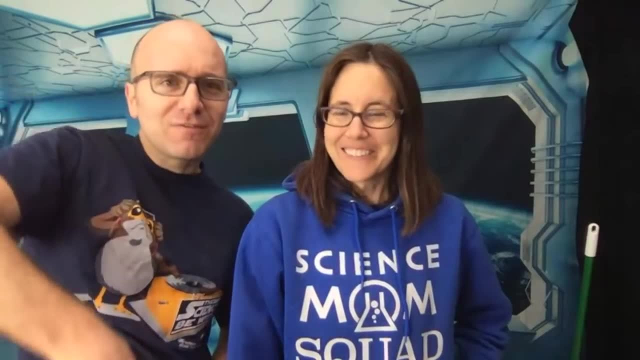 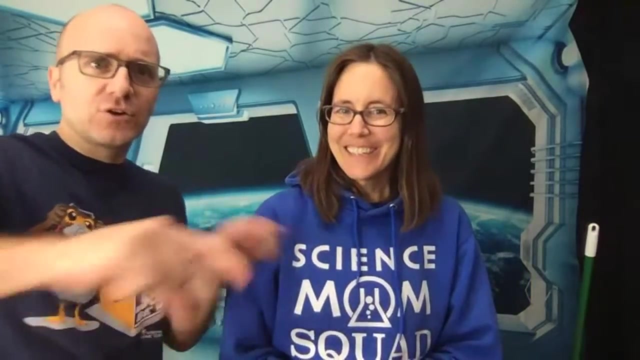 And the whole wall lifted. we were able to shove some gravel under there and took a little bit of adjusting, But somehow with one hand here I was able to lift this rock bar and lift this entire brick. And well, the walls, they were stacked and they were intertwined with each other. 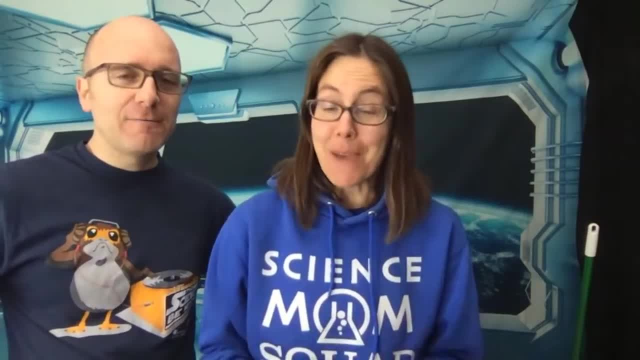 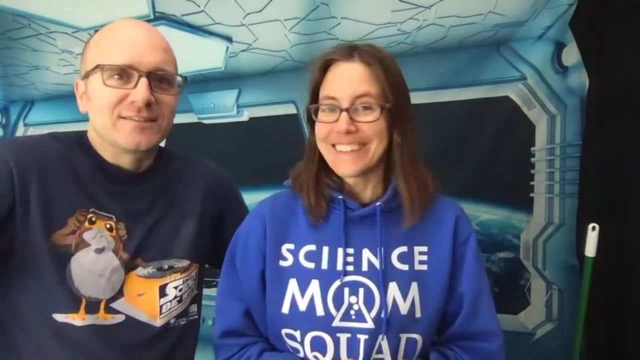 If you don't understand the physics of simple machines, they seem like magic, like legitimate magic. It's incredible what you can do just by adjusting your leverage. They're better than magic because you don't have to spend any time learning it or casting spells or incantations. It was just insert and leave. 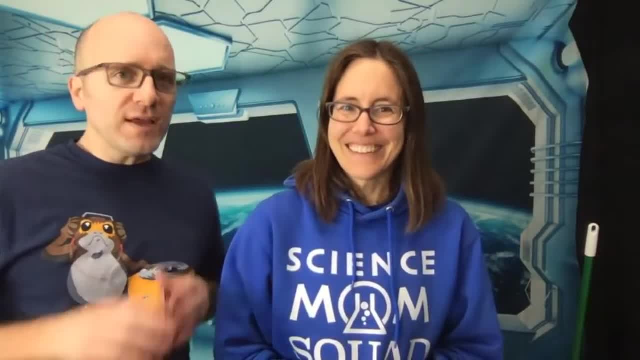 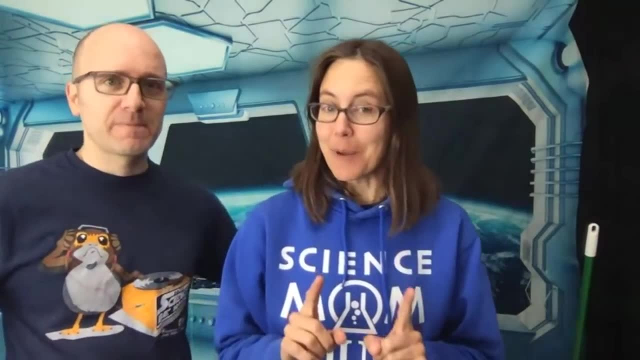 Yes, Yeah, And it's kind of crazy how prevalent these are. So that's an example of a lever, But before we get into types of lever, let's talk about teeter-totters. Okay, And I'm going to. So, Math Dad, if you can move our view around. 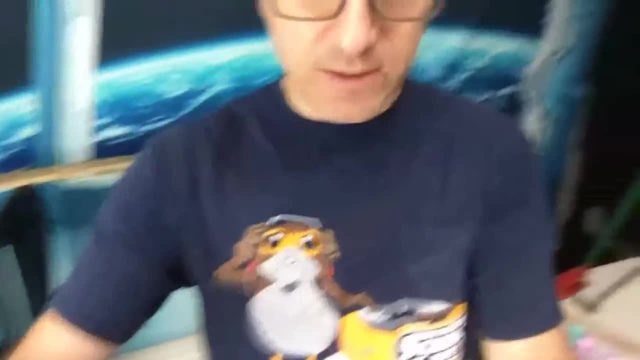 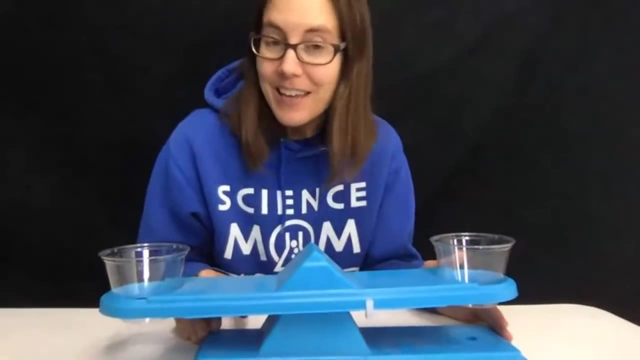 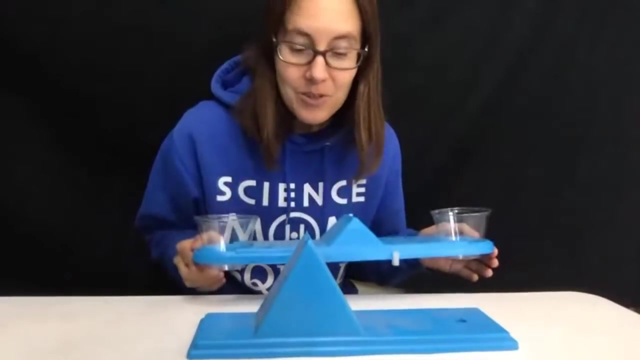 Oh, you have something set up for us here. Yes, I do So. one of the best ways to learn about levers and to understand how levers work is to start off with a simple teeter-totter. So I have a teeter-totter here and you can see that there is just a fulcrum. 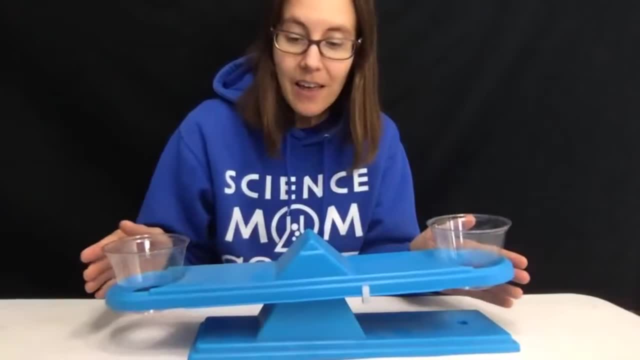 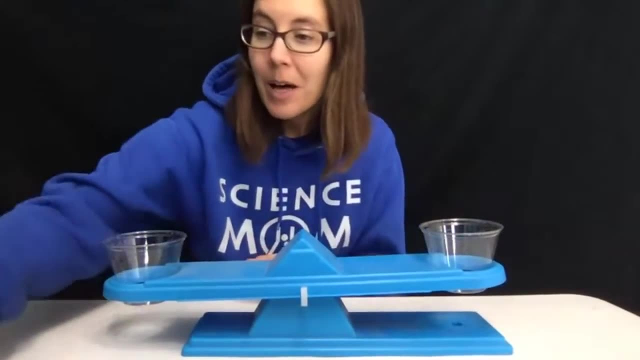 a point where this top bar can balance And right now move that little gauge there. Right now it's balanced. I've got two cups that weigh the same, But what happens if we start to add some friends? I made some little eggs that have a little bit of. 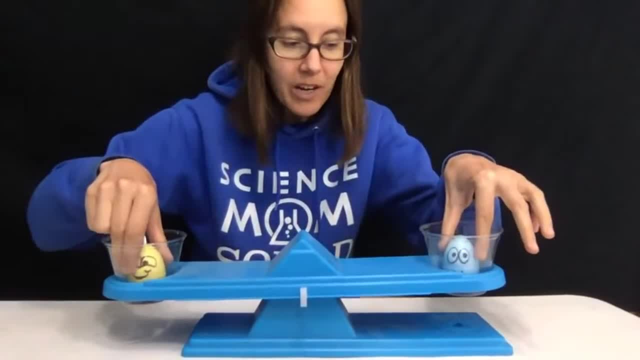 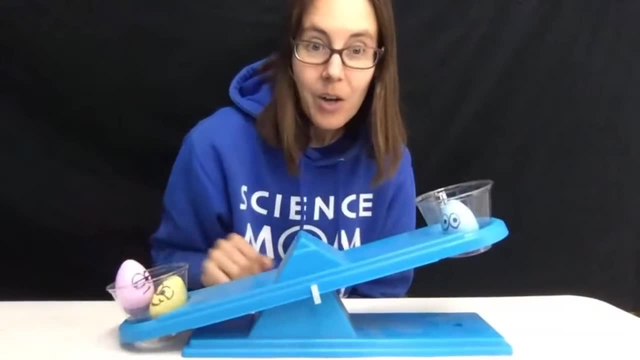 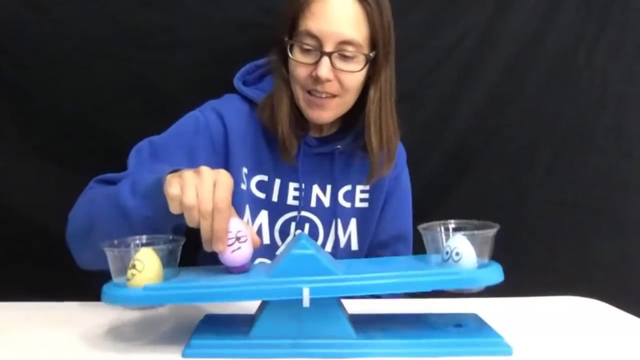 clay inside. And if I put two eggs in here, one on each side, it stays pretty balanced. But if I add a third Grumpy egg over on this side, now we're not balanced anymore. We have more weight over on here. But what happens if, instead of adding the egg at the end, I add the egg in the middle? 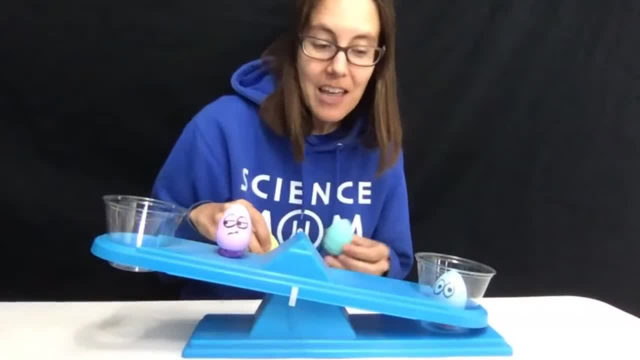 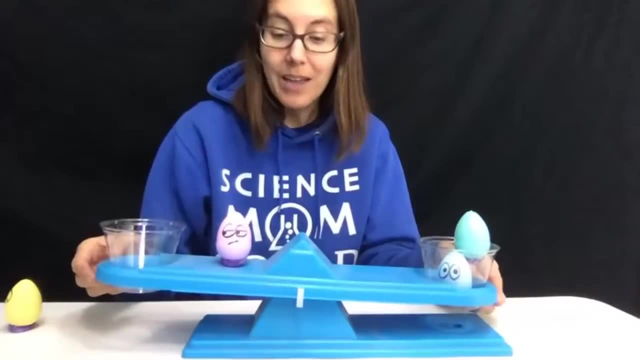 Can I get my lever to balance? if I have an egg in the middle versus over here, Well, that looks way too heavy on one end. It is too heavy on one end, It's lopsided. But if I'm able to move it, and with this one, 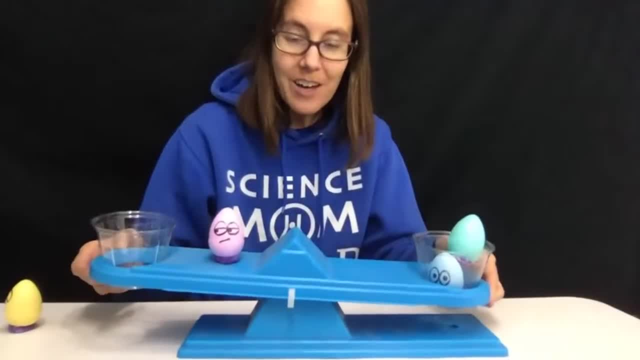 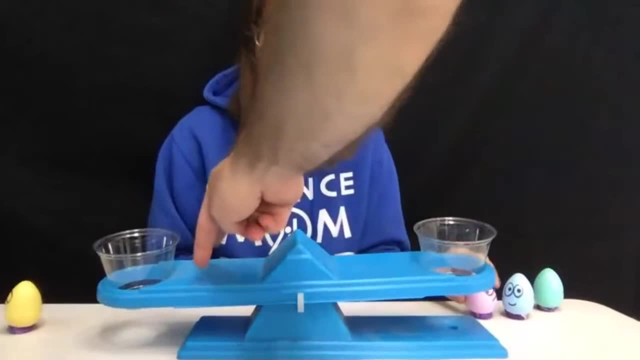 it's a little hard to move it because I've got the, I've got this nice big triangle in the middle And if I offset it all then it will throw things out of balance. So let me show you, Well, what if you had one here and two here? 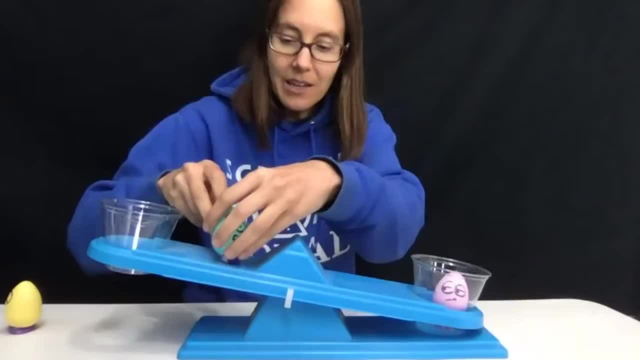 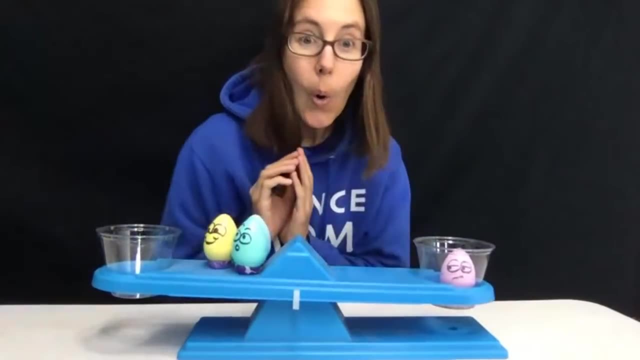 One here and two over here, That might work. Let's see if we can get it to balance again. Two's not enough. What if we add a third? Oh, we're so close, We're so close. Oh, look at that, We have three right here, closer to our fulcrum. 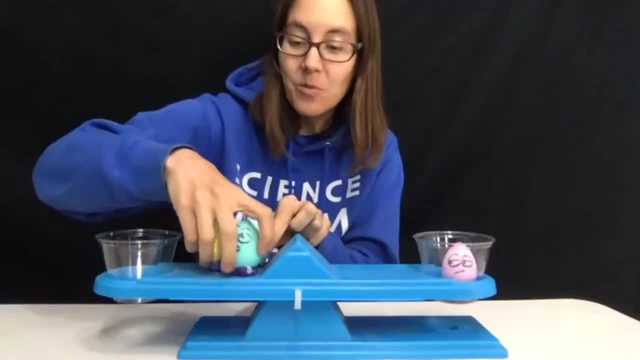 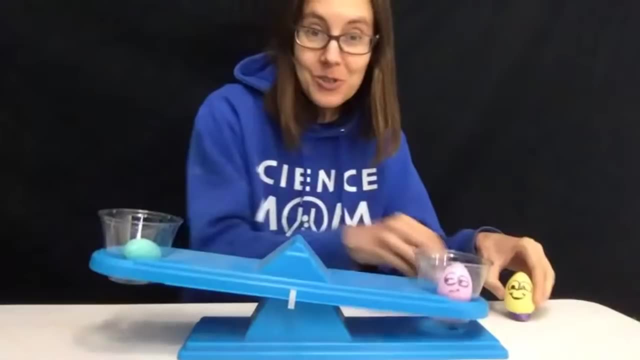 and one over here and we got it to balance. But of course, if we put these three out here in the main cup, then it will fall. Now you can make your own teeter-totter. Just look around your house, see what kind of supplies you have, and as long as you have something that they can. 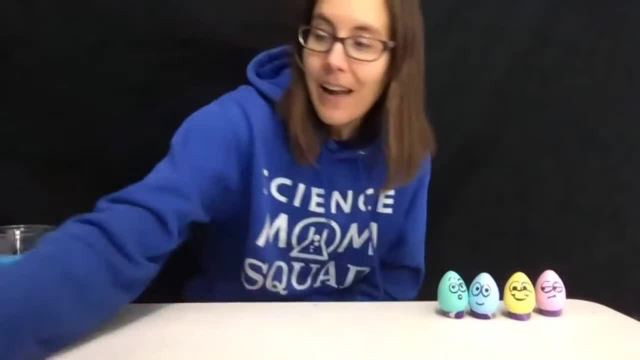 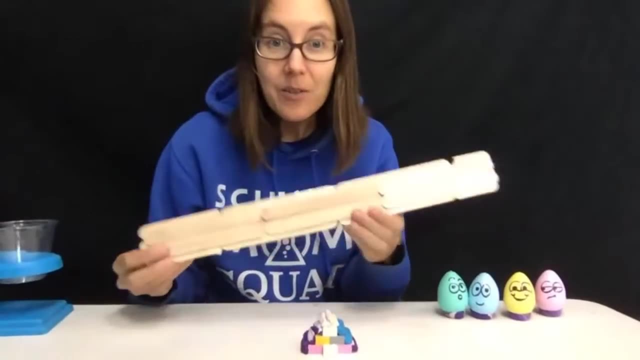 balance on. So I'm going to show you my homemade version now, And I made this out of Legos and clay. I just put some Legos together and kind of put some clay on the top to make it a triangle, And then I glued together some popsicle sticks to make my beam And right now it's balanced. 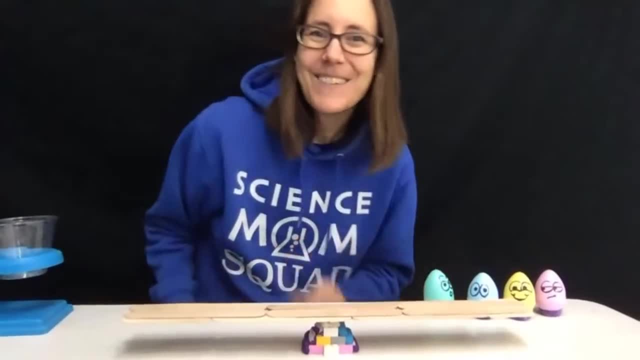 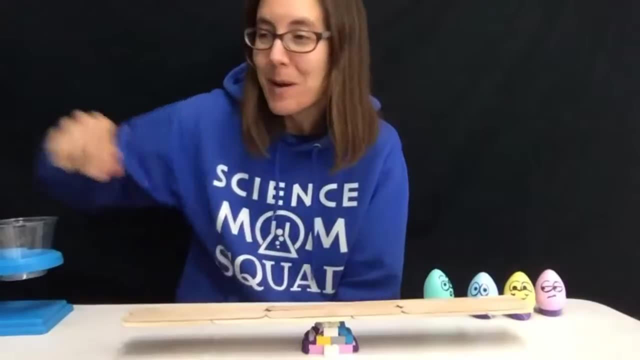 Don't tell her that we have actual boards we could have used. My dad said: don't tell her, we have actual boards that we could have used. I could have used some boards, but it was kind of fun to glue together my popsicle sticks. All right, Now let's put. 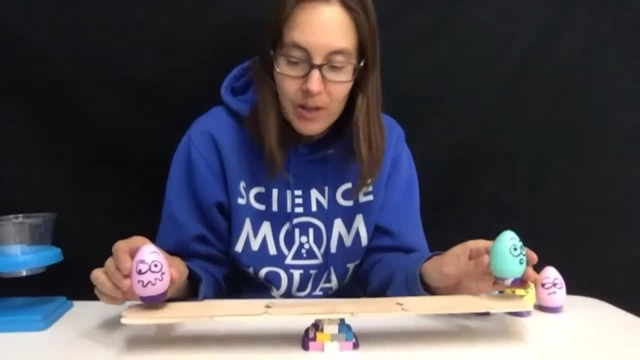 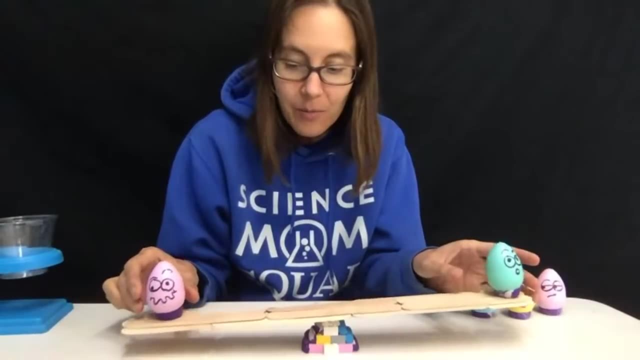 some eggs on and see what happens. So, just like before, if we put equal weights on either side, then I have to adjust them in and out a little bit. There we go. We're pretty well balanced. So now we have a teeter-totter where just a little bit of force on one end. 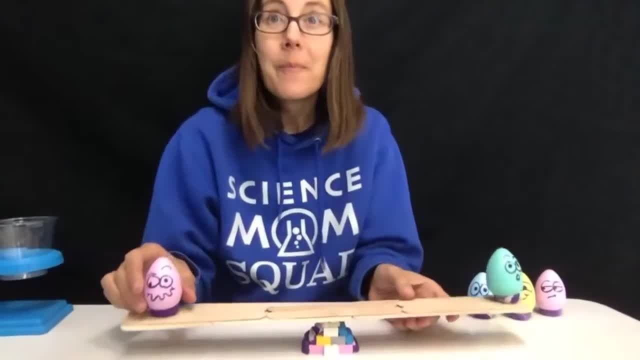 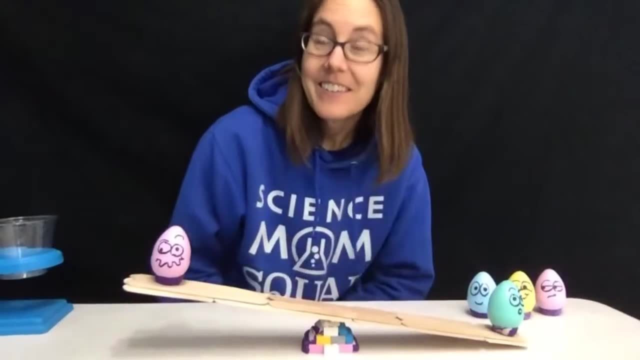 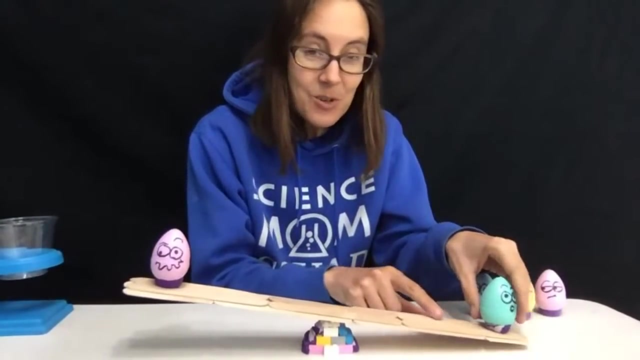 will cause the weight to shift. Well, if you're actually on a teeter-totter and you lean back further, you may have noticed that that's often enough to get it to go in your direction. Or if you lean forward, that can have the opposite effect. So you can experiment with. 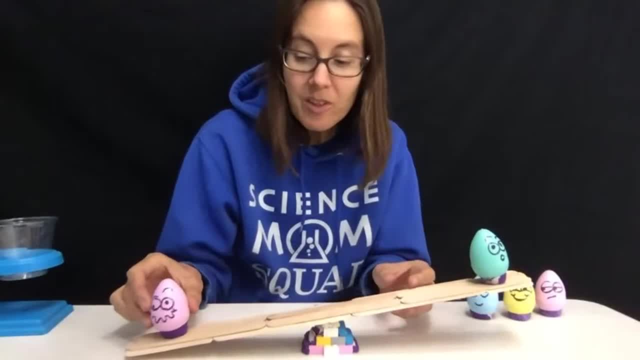 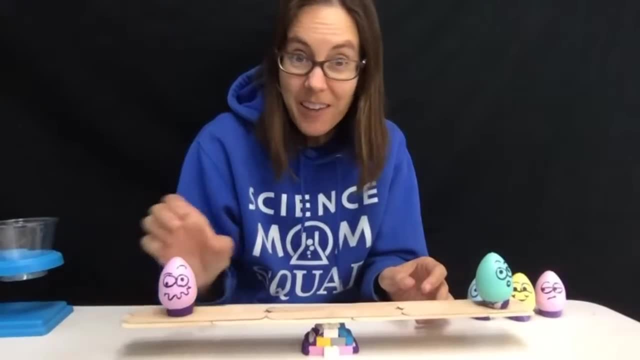 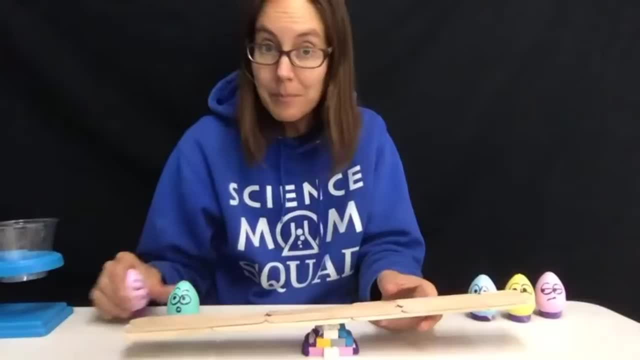 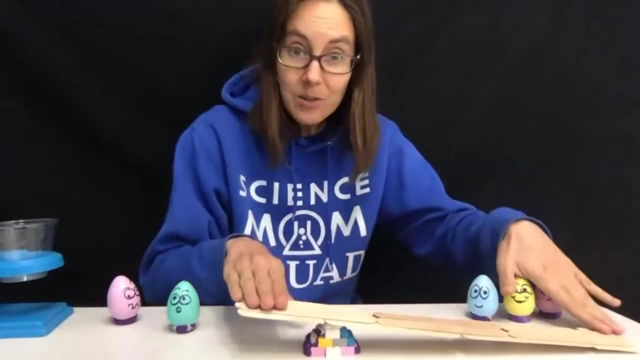 fine-tuning. But what happens if our fulcrum is not in the middle? So the fulcrum is the balance point. And then here, what if we do something like this? So now our teeter-totter is not balanced. 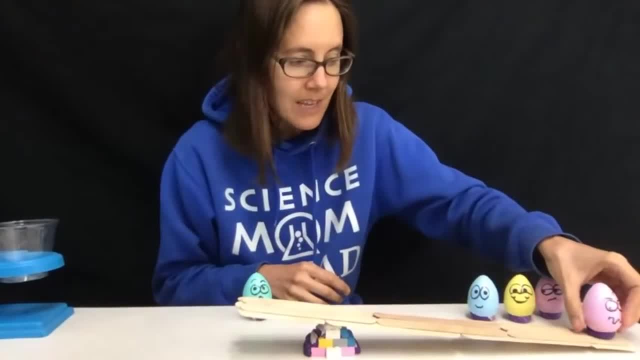 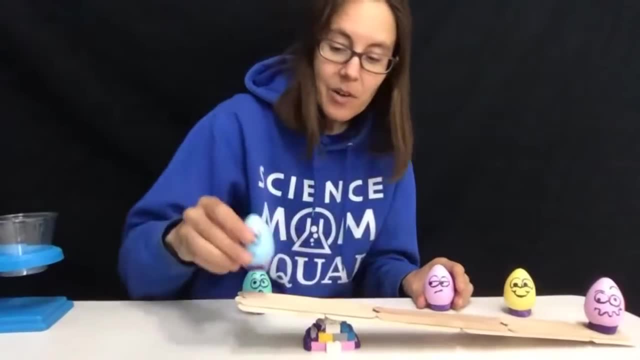 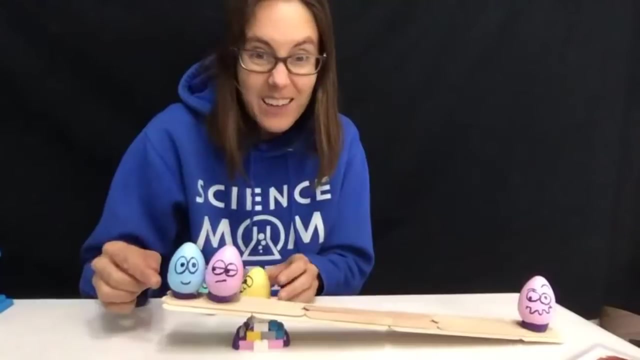 And let's put our grumpy-faced egg over here. The grumpy-faced egg, let's say, is kind of stuck and needs to be lifted up, just like those heavy bricks that Math Dad was lifting. Well, if we put some weight over on this side and apply a force downward- and this with the eggs- it's going to. 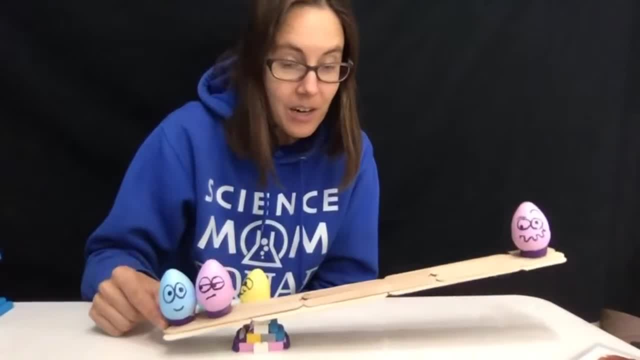 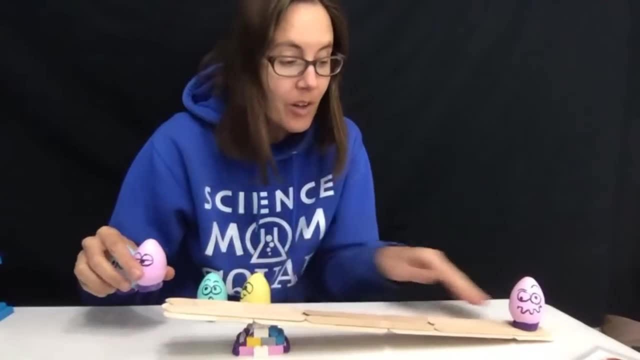 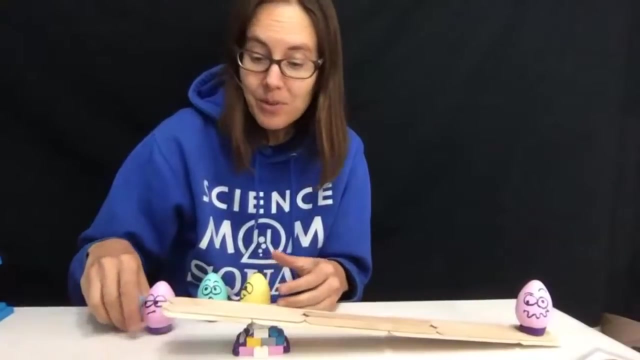 take more eggs than I have space for. But by applying a force downward here you can lift something up, And this is a lever. If you have a force over here, the fulcrum in the middle, and then you push down, your weight will go up And this is a class one lever, the simplest type. 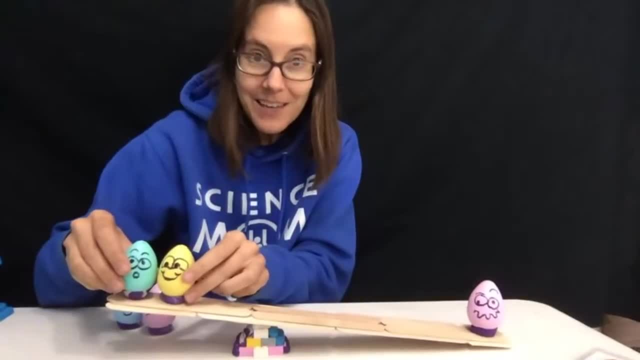 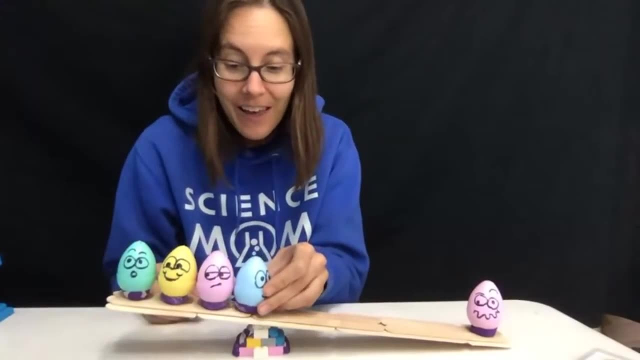 of lever And I have to say when I was making these little eggs I was having a lot of fun just experimenting and playing with them. You can learn a lot about levers and about force Just by experimenting with some simple machines. 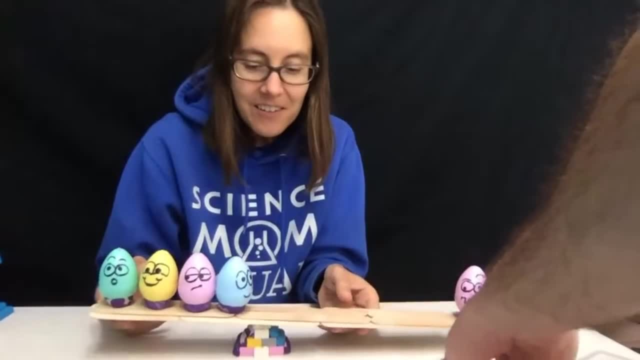 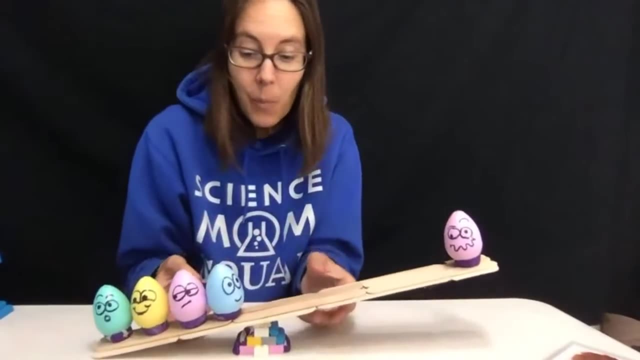 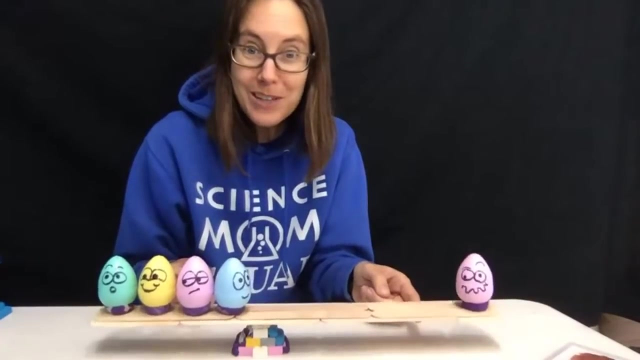 Well, it's crazy that you can think of it. this egg is enough to lift up four different eggs by placing the fulcrum close to them. Yeah, So look at this. Oh, I was so close to being balanced. There we go. We're really close to being balanced now, And if I scoot this guy in just a little bit, 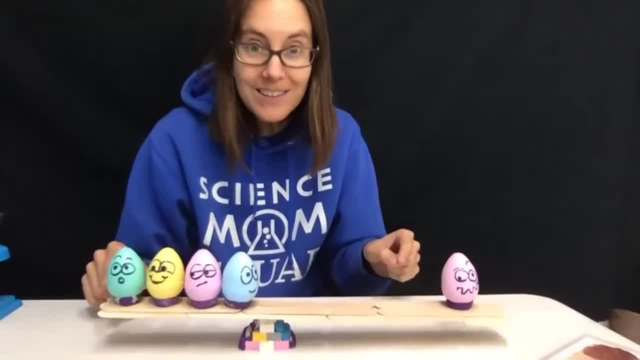 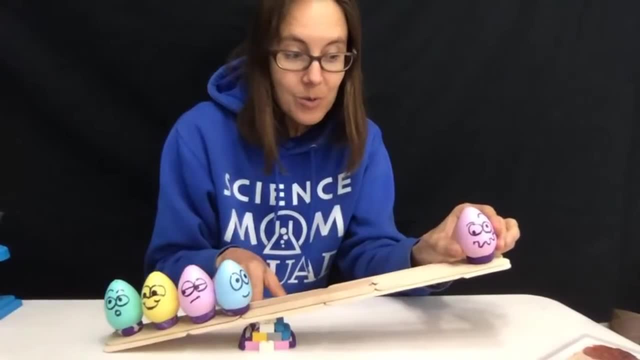 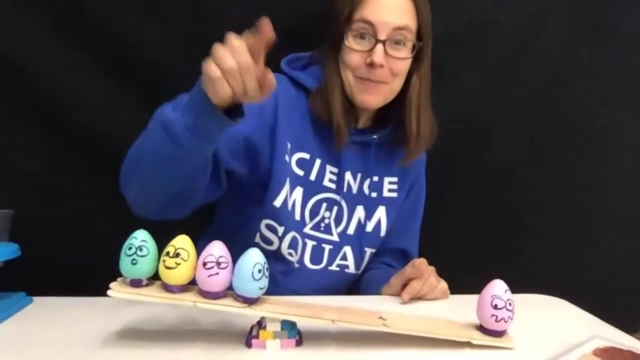 Oh, come on. come on, There we go. We're balanced. This one egg is able to counterweight all four of these because our fulcrum is closer to them. So if I set him out on the side, lots of fun. Now let's bring the view back up top And we'll 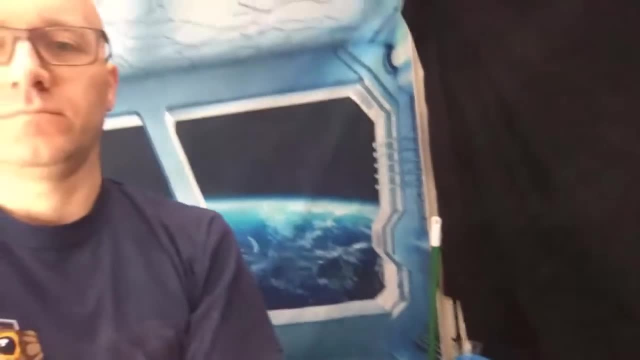 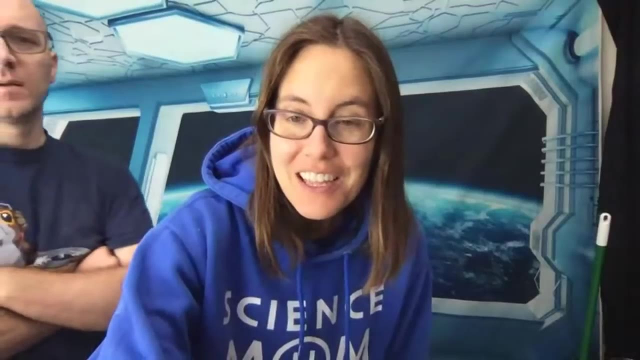 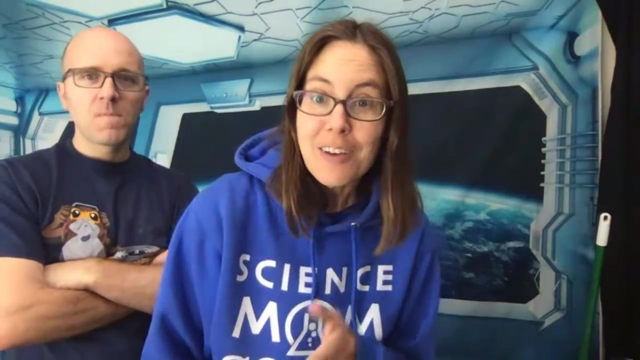 talk a little bit more about types of levers And I want to give a quick thank you to our moderators in the chat. So we have: On Facebook we have Science Mom, Krista, And on YouTube we have Liza and Blanca and Amber, and 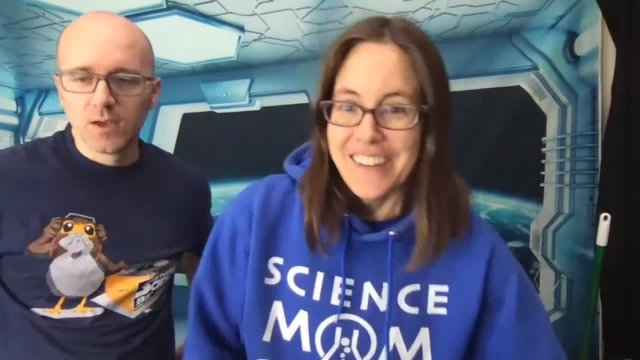 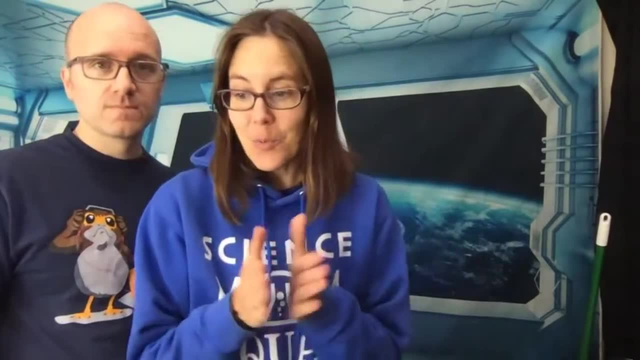 Jamie, Thank you for moderating for us. So let's talk about types of levers, because we use these all the time. You just might not realize it. So a class one lever when we've got our fulcrum in the middle, and then the weight on the force on one side and the weight on the other side. 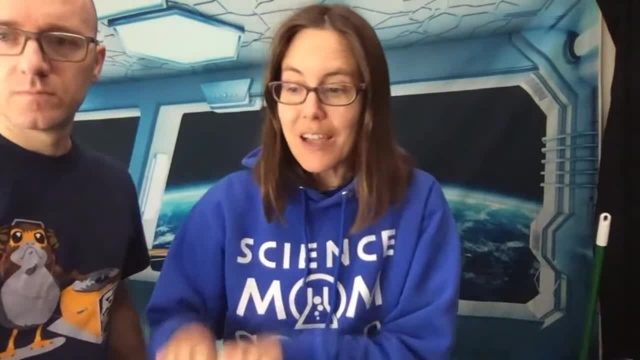 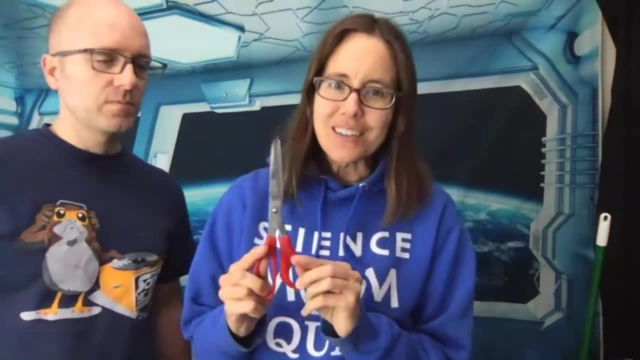 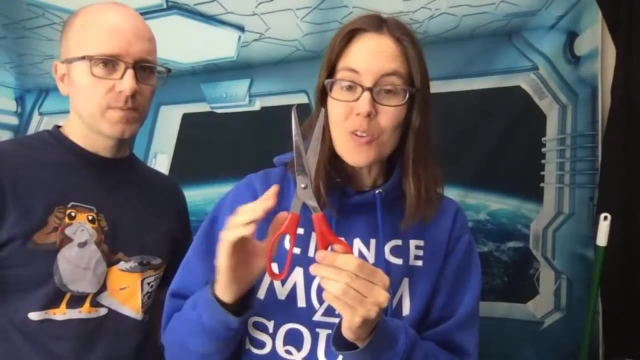 One example of that is like a pry bar, like pushing down to pry something up. But another example: oh, do we have? We do have some here. Another example is scissors. This is actually a double lever because we've got a fulcrum right here in the middle where you have that part where it can. 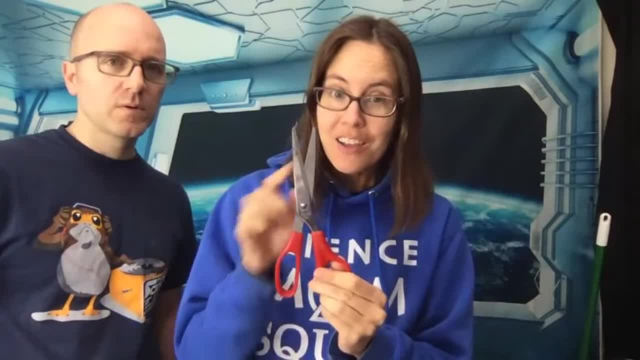 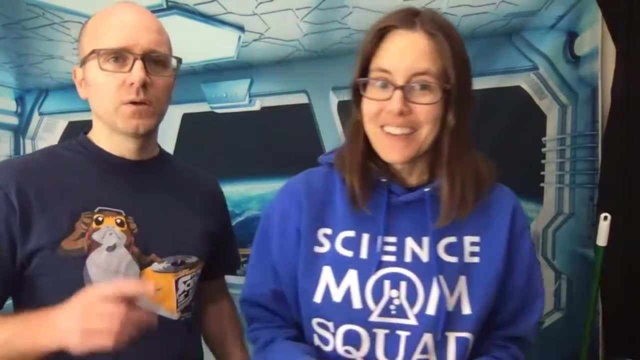 shift its weight And then when you apply force here, it moves the opposite direction And you actually have two levers working together. That's essentially what a pair of scissors is. So a class one lever. you're saying the fulcrum is in the middle. 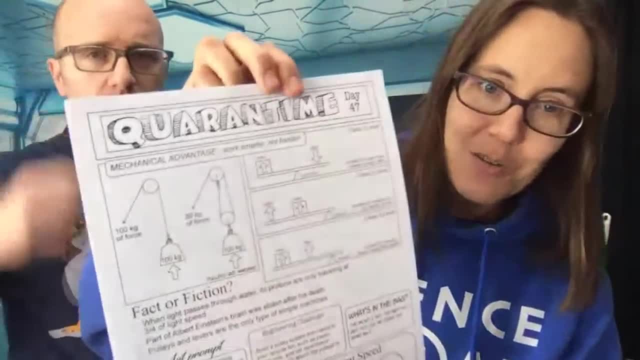 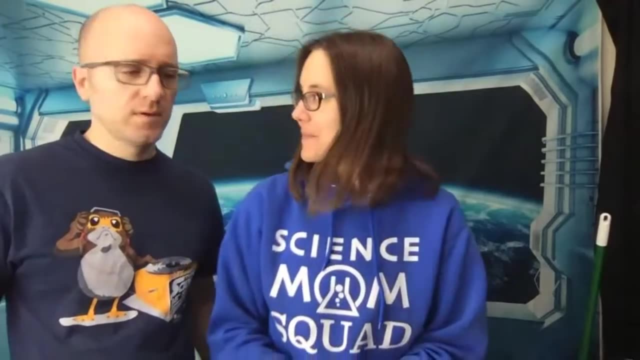 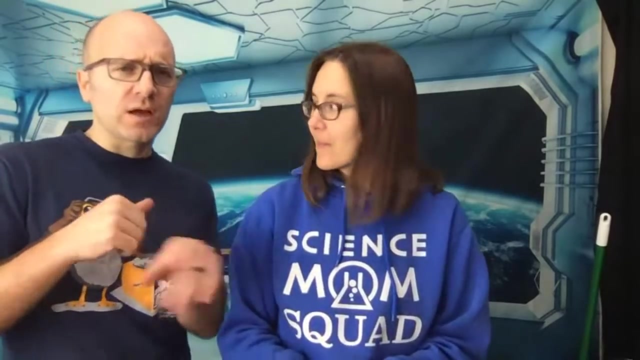 Yes, Fulcrum. Fulcrum is in the middle And on our little handout that you can download for free from Patreon, we have a nice little some reach heart there of the different types of levers. So those ones are kind of neutral in the sense that both sides are balanced And we'll talk. 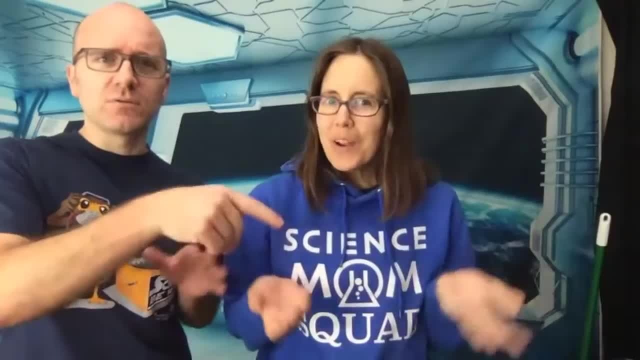 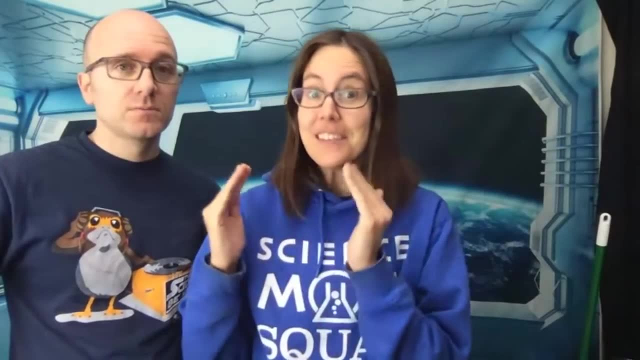 about some of the math behind it in a couple of minutes. But what if the sides aren't balanced? What if your fulcrum is not in the middle? What if it is off to the side? And it turns out that this is a type of lever that we use as well? 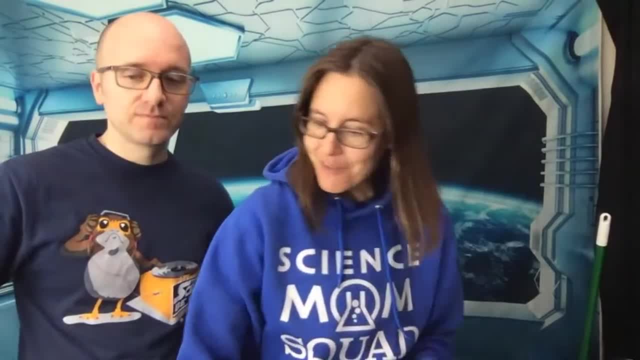 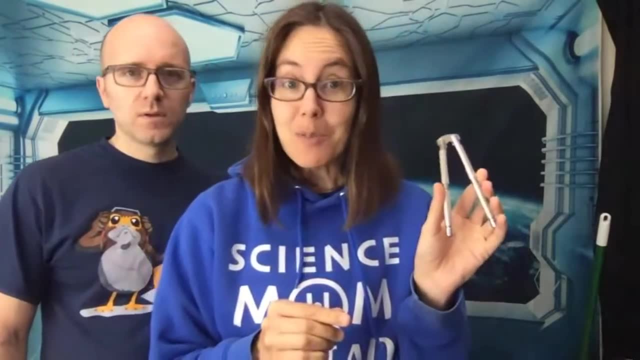 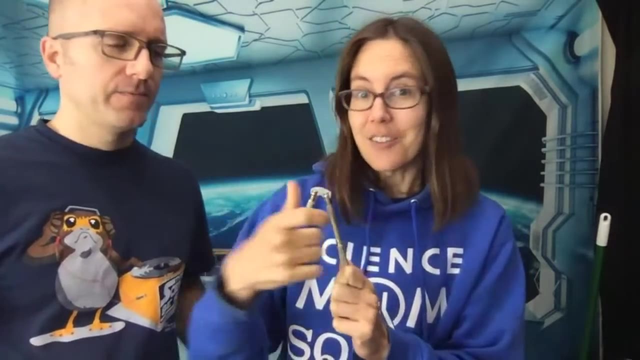 Maybe not quite as often as the other ones, But in fact let's pull up a little example here. So a nutcracker? A nutcracker is like a type two lever, where you are applying your force down here, Your fulcrum is up at the top, And then the weight, the thing that you're hoping to change. 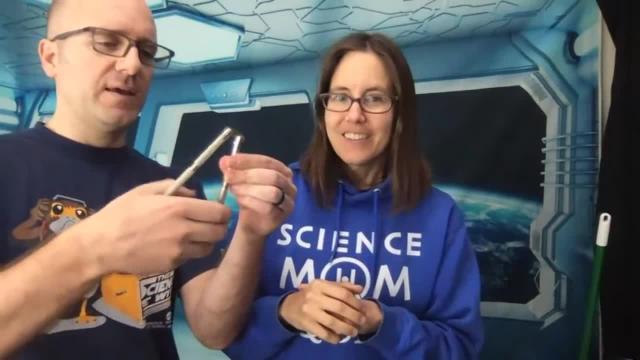 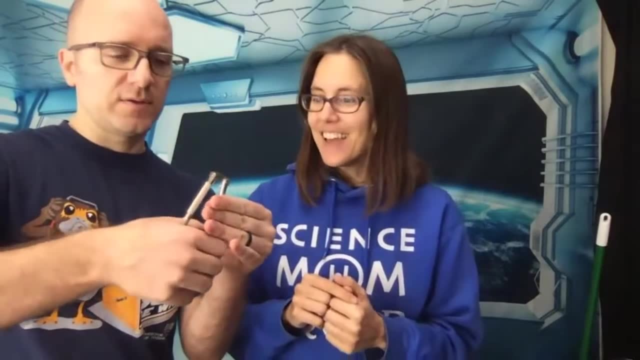 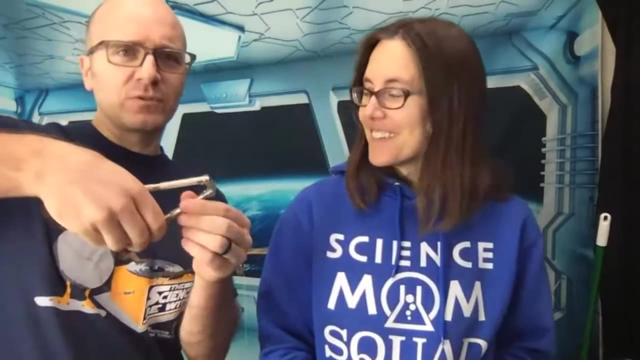 is in between the two. Okay, So in that case, by exerting force at the end, I'm getting extra force in between. Extra force in between, Yes, Yeah, The longer it is, the more that force increases. Yeah, Yeah, I've definitely seen some of those before, but yeah. 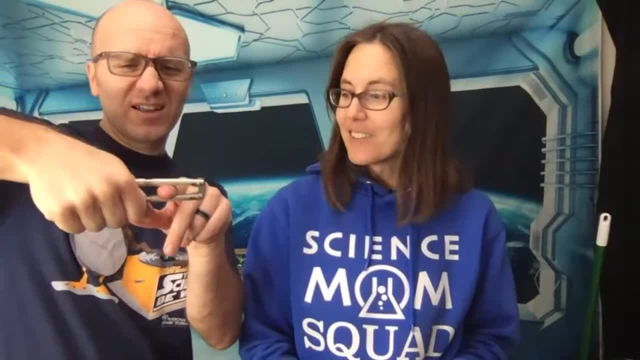 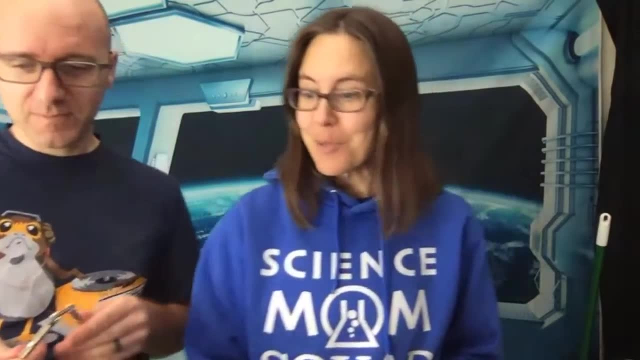 it's amazing how much pressure you can do. I mean- Don't pinch your fingers with nutcrackers, This isn't that long, but boy, oh boy, can you apply a lot of pressure. You can apply a ton of pressure. And then another fun example of a class three lever. 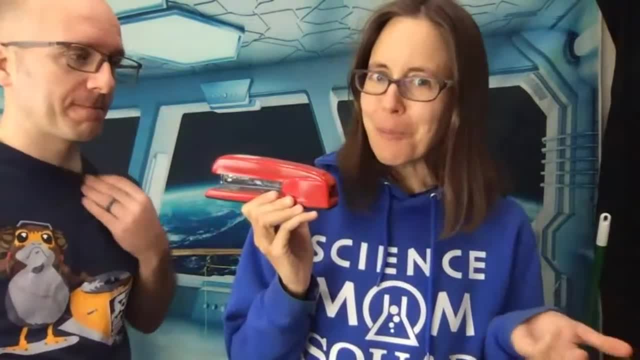 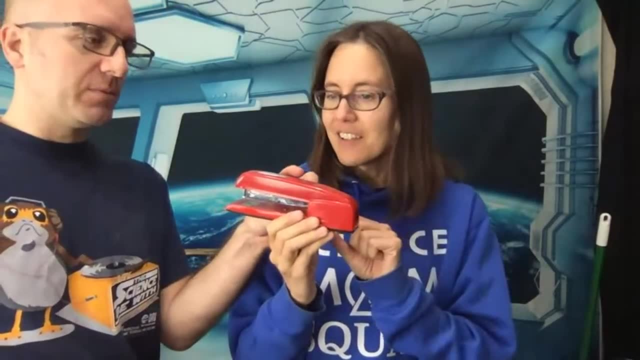 is a stapler. We don't think of this as being a lever, but it actually is So. class- Three. So the fulcrum is at one end, but you're pushing in between, You're pushing in between And at the end-. 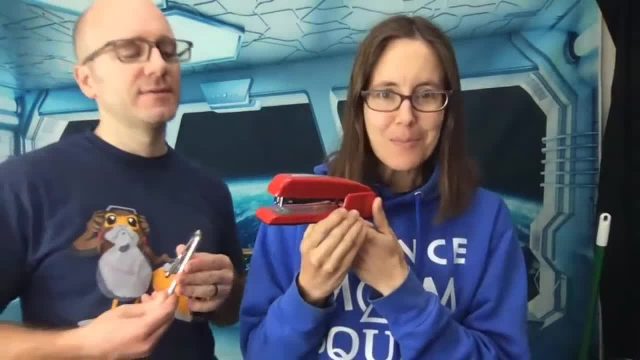 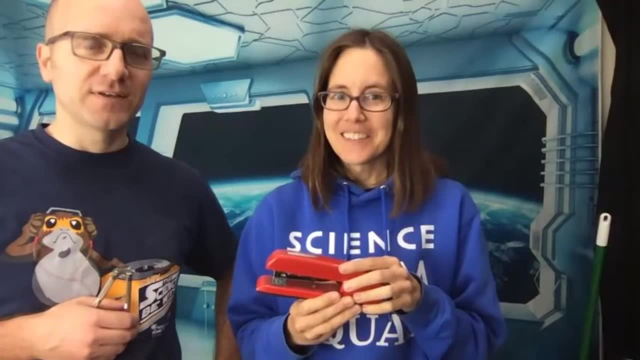 You have your- Is the effect? Is the effect? Yes, So a stapler is really a type of lever. We use these all the time. Now, this one's actually kind of inefficient in the sense that you're going to have to push even. 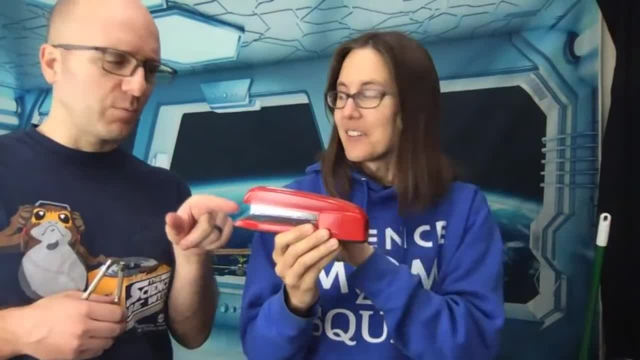 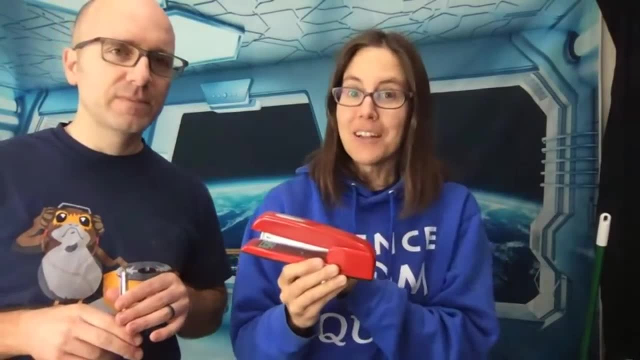 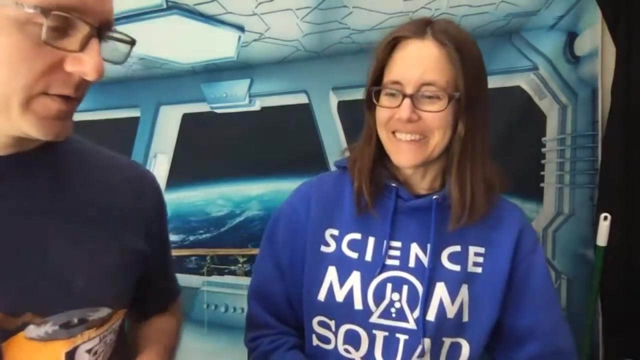 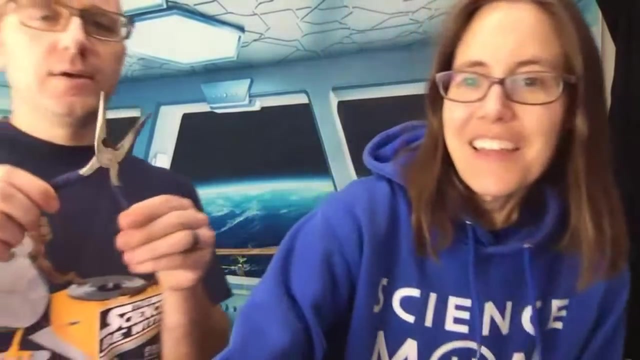 harder here to get the same push at the end, Yes, But since we have a machine that pushes that force all into that tiny little staple and then has a thing underneath to help bend it, it's actually quite a useful tool. Oh, that is pretty cool. Okay, So I actually have a few more items here that I collected this morning. 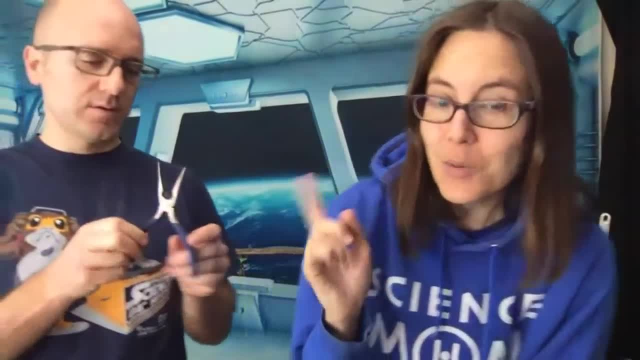 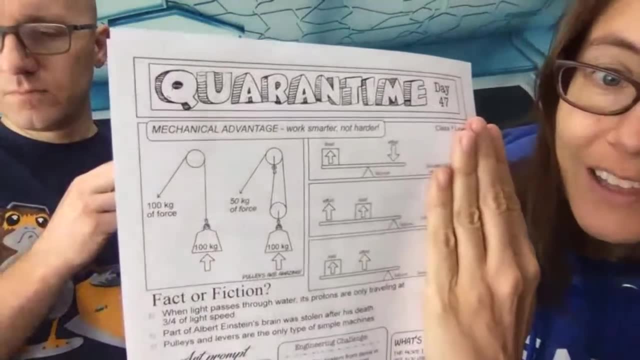 And if you are watching in the chat, if you're watching live, tell us what class of lever this is. And maybe here I'm going to hide the little answers here. but quick little review. So Class One: we have the fulcrum in the middle. Class Two and Three: we have the fulcrum on the middle. Well, so if you wanted to look for the fulcrum, that's what you do And you can also see the fulcrum and all the stuff that's that's visible here. so it's a little sample and then, you know, has a thing underneath to help bend it. It's actually quite, quite a useful tool. 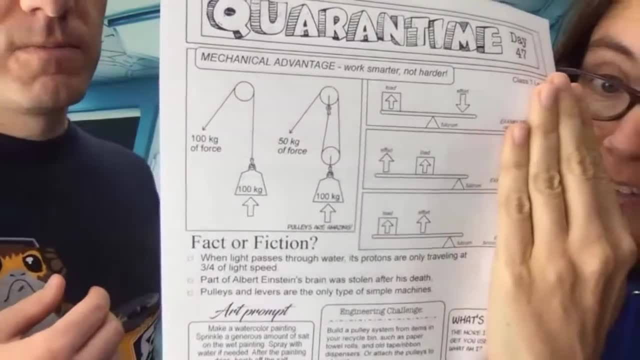 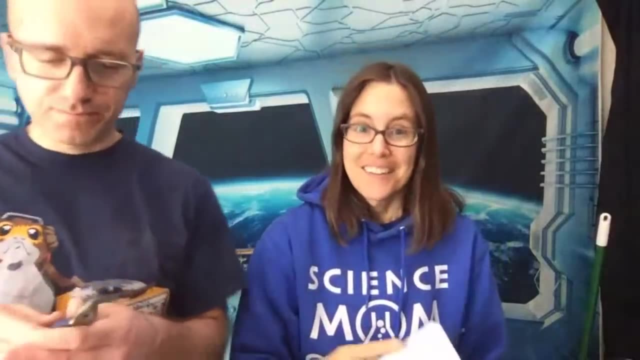 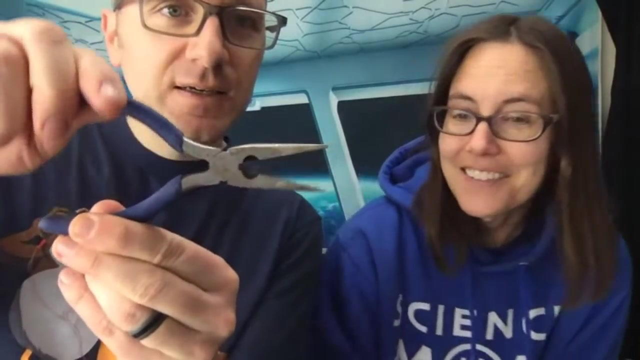 we have the fulcrum on the edge, and if the force is applied to the very outside, that's class two. if the force is applied to the middle, that's class three. all right, so right here i've got set of needle nose pliers. what class do you think that is what? what type of letter? 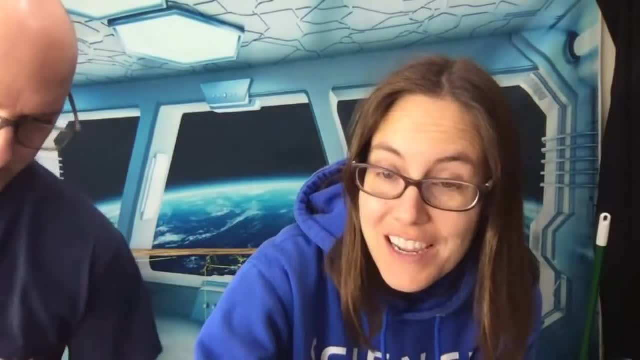 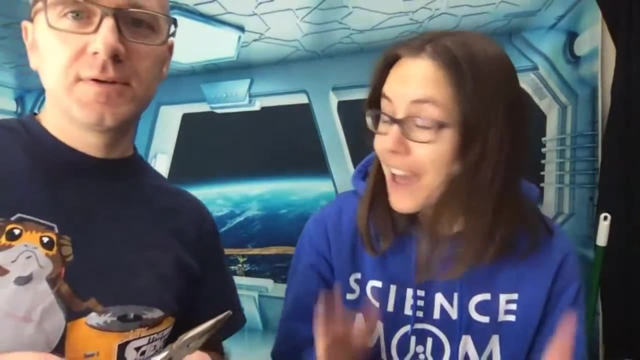 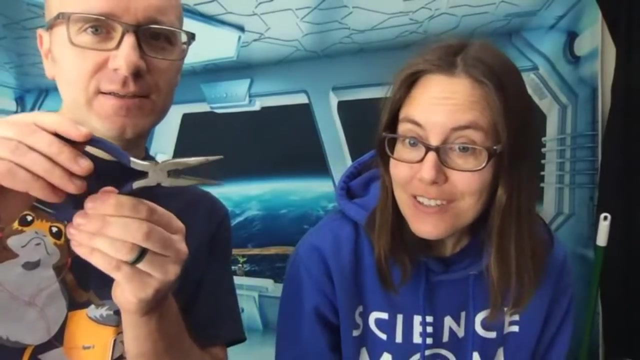 let lover- i'm seeing zara, j, thomas, courtney are all saying class two. king husky says class one, two and three hedging his bets. class one in there, all right, and two bridges says class two. jesse says class two, sheree says class two, class two. 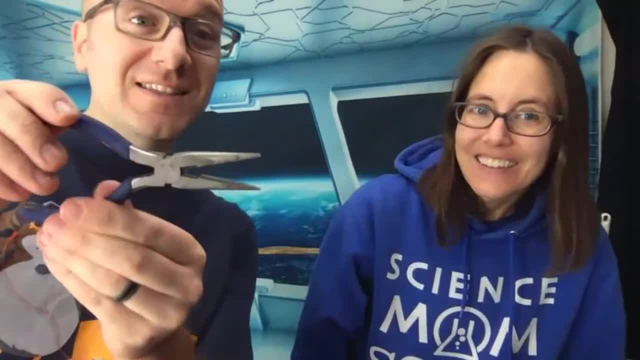 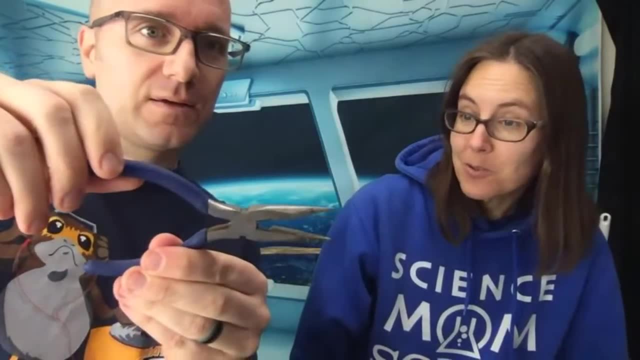 all right, math dad, what is it? carrie says class, class one. all right, this is actually a class one lever, because the fulcrum is right in the middle. so it's just like a pair of scissors, right, uh? yeah, yeah, like scissors, or like the balance beam, the science mom, which is the science mom which is. 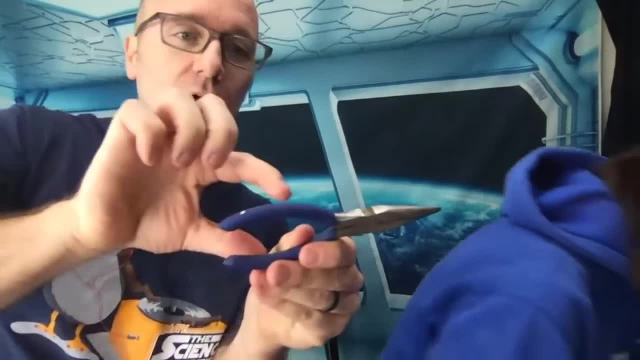 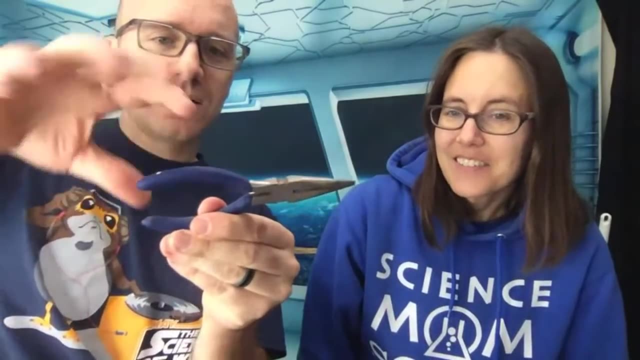 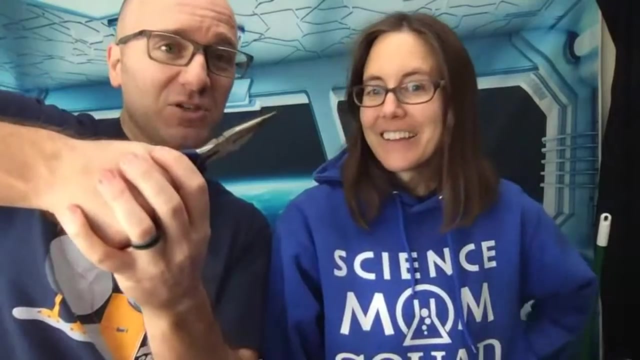 showing us before. so the the longer these handles are, the more exaggerated is going to be the force on the far end. so in this case i'd say my handles are only twice as long as my needle nose end. but boy, oh boy, is that enough? got a decent grip strength here and that's going to really 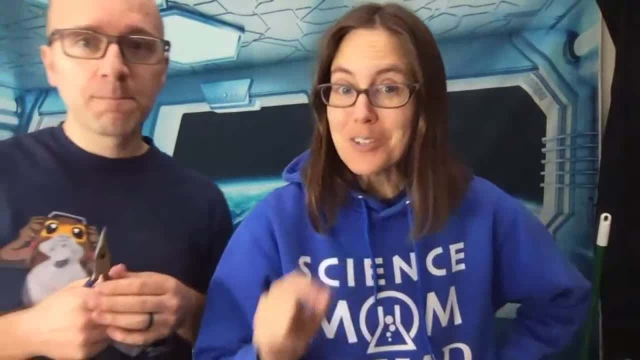 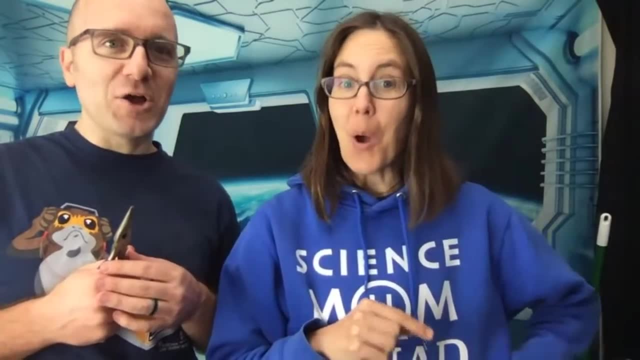 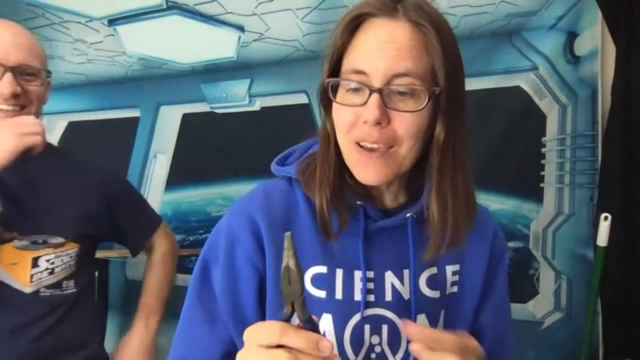 compound to the other end. i just saw a really interesting question go by in the chat. someone said that their son would like to know if needle nose pliers are for taking needles out of your nose. hopefully not, you know, they'd probably work for that. but i think they're called needle nose because the nose or the 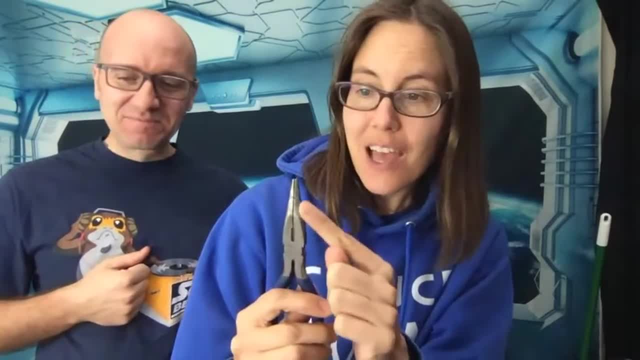 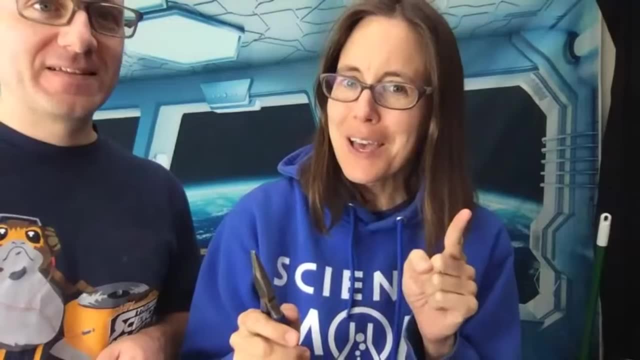 top of these pliers is very thin. most pliers have a have a blunter nose but these thin ones are good for reaching into small spaces. hopefully not anyone's nose, but you know, if you have something stuck like in a crack in between, you know, i don't know the edge of the wall and a couch and like. 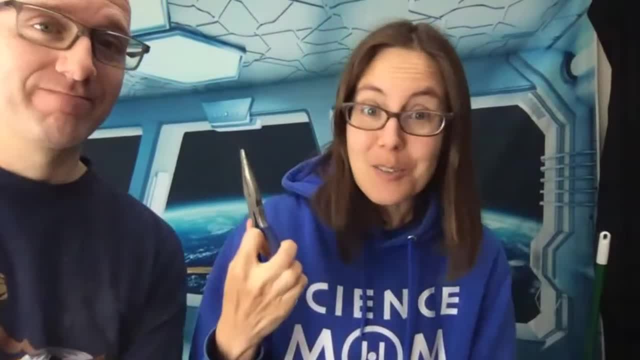 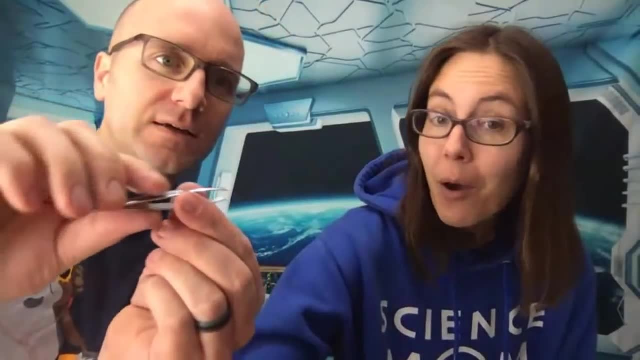 something that you can't move and you want to pinch and pull needles, and those pliers are really useful for that. all right, all right up next a set of tweezers. tweezers. so think about where the fulcrum is and where you apply the force, where the fulcrum is and where you apply the force, and then tell us 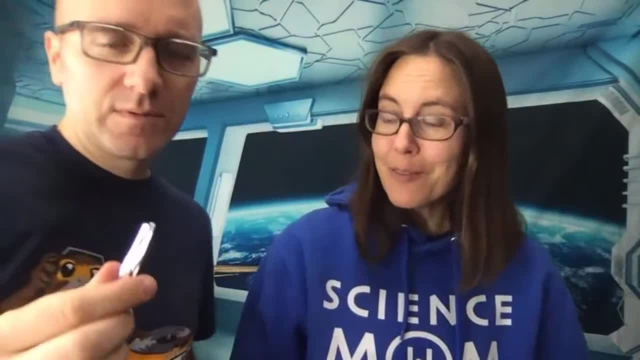 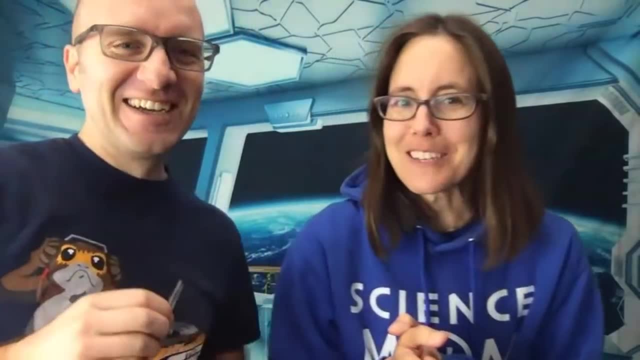 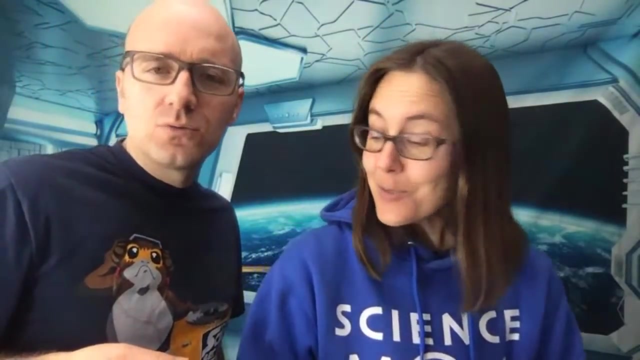 if you're watching live, tell us in the chat what type of lever are tweezers and i'll narrow it down for you. it's either one, two or three. that's not narrowing it down very much. well, it's not four, because there is no type four. he says three, owen says three, sarah says three, olga says three. 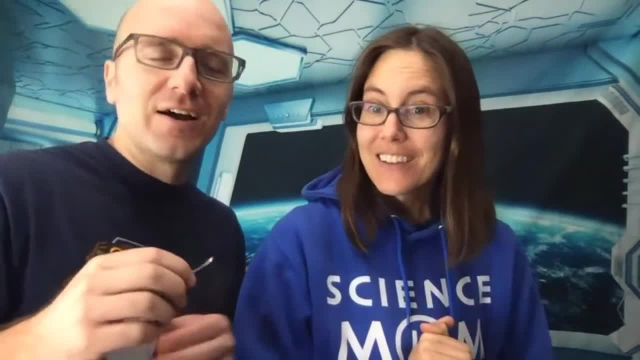 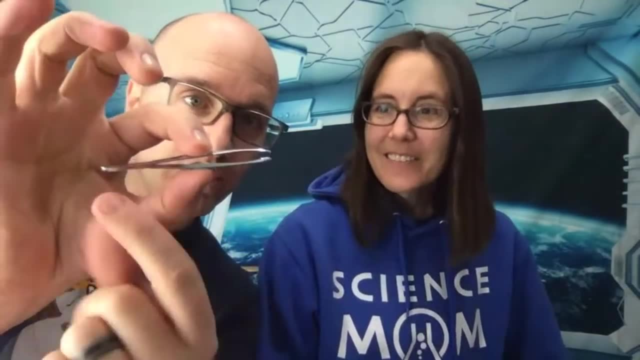 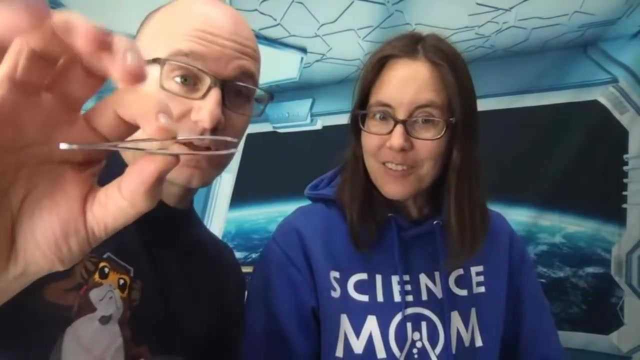 chat seems pretty. courtney says: three panels aligned on this. okay, uh, okay, you've got it. it is indeed type three, so i'm applying my pressure in the center. the fulcrum is at this end here and the effect is right. it's right at the, the tip, so that this is indeed a type three lever, and i mean 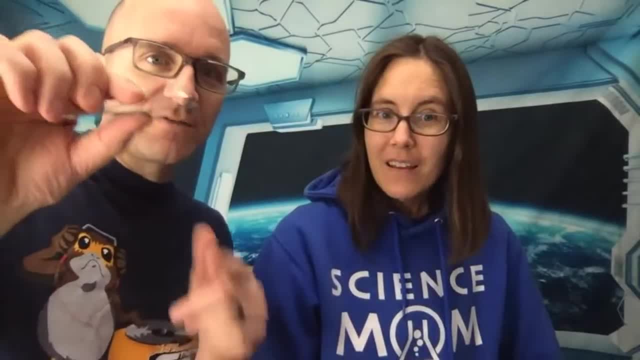 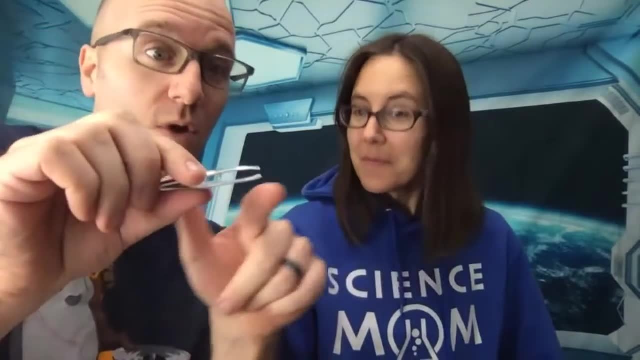 type threes are inefficient in the sense that i actually have to push harder here than the force i'm going to get at the end. however, boy the tweezers, i mean, this is just exactly the same as the other ones. exactly what you want. you want some type of effect at the end that's away from your fingers. 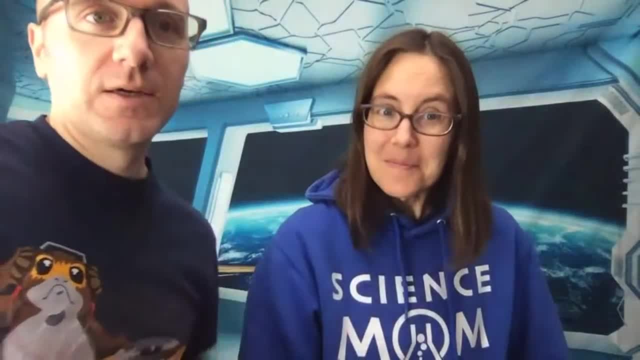 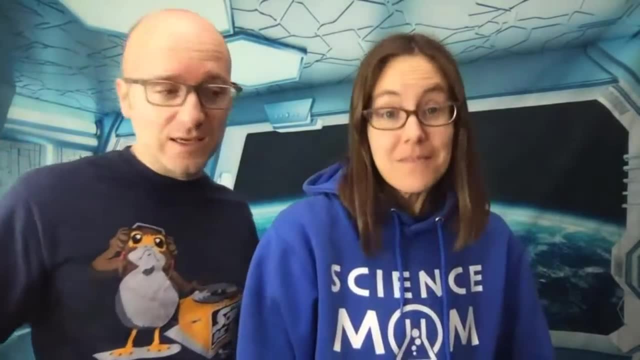 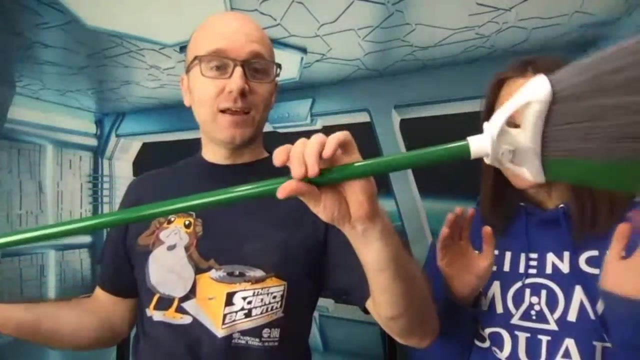 because of the precision work that tweezers can do. so i mean first when i look at type three, like why would we ever do that? but then i started looking it up. yeah, there's plenty of examples and in fact, oh, this is a good one. i've got a broom here, so when i'm sweeping 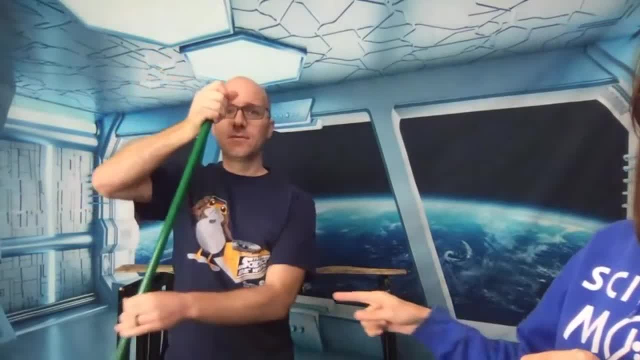 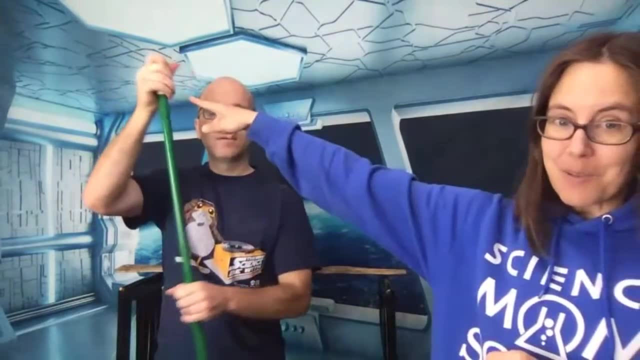 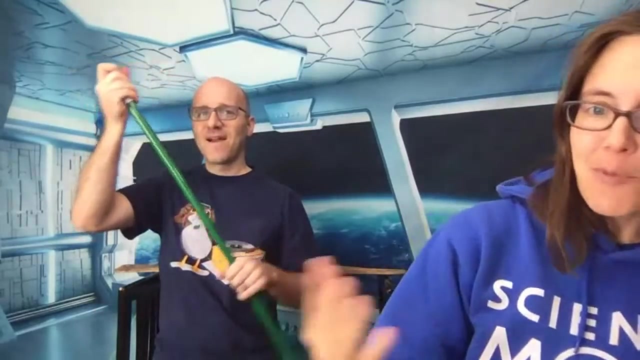 um, so think about where the fulcrum is and maybe try and yeah, so see, this hand up here is not moving as much. so here's our fulcrum. we're applying the force here and we're getting getting an effect down there. so what type of fulcrum or what type of fulcrum is this? what type of lever? 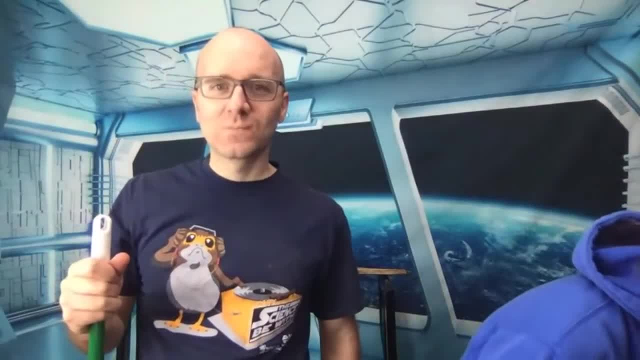 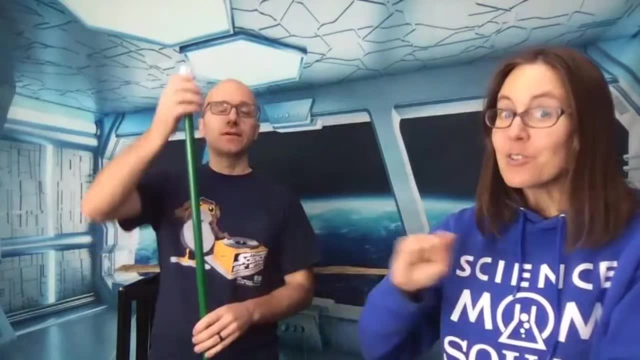 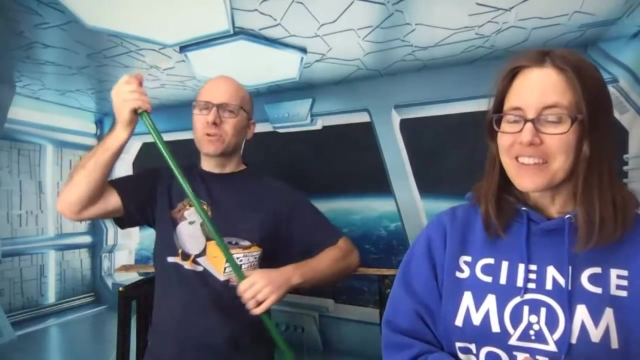 lyndon says class two, larissa says class three. listen, this one's gonna two, three. it kind of depends on how you use it. i think, depending on how you use it, you could make it true. i was trying to hold my top hand steady, because that's actually the typically the one that does stay steady, although there's 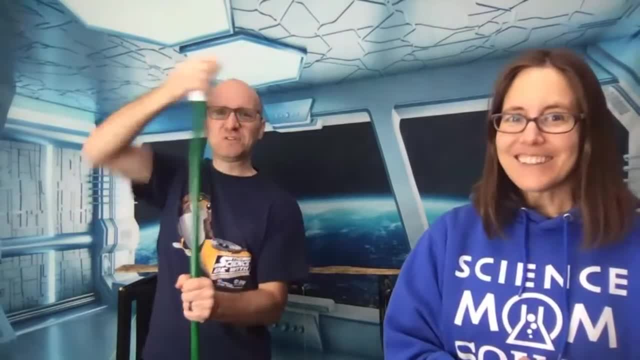 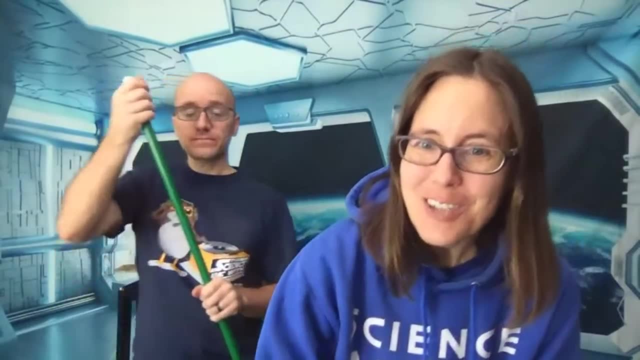 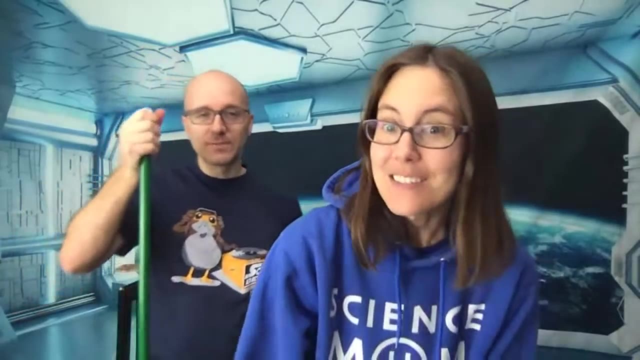 there's no reason you couldn't hold the middle hand steady and sweep that way, although that doesn't work when you think about it, i doubt that's what you actually do. so good job to budapar. to um some, i saw so many people say in class three, debbie, and that is right. this is you. 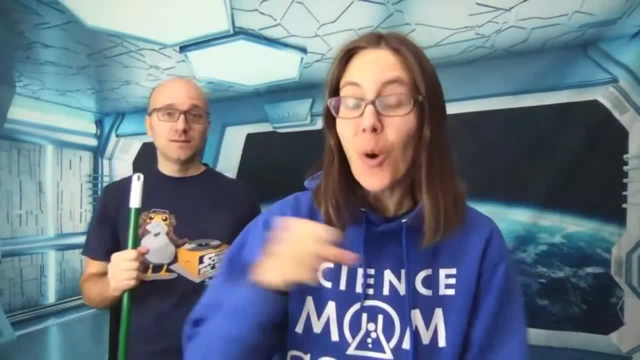 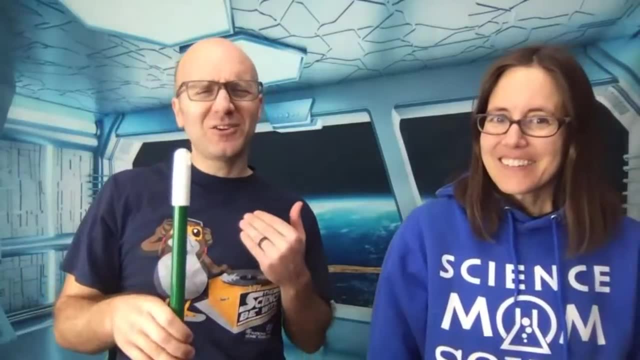 usually used as a class three, although, depending on how you hold it, you could make it into any one of the type of levers. yeah, but kind of fascinating though, because here i am thinking you know, class three, that's not very efficient. i bet we don't see that one very often. oh, my goodness, when was 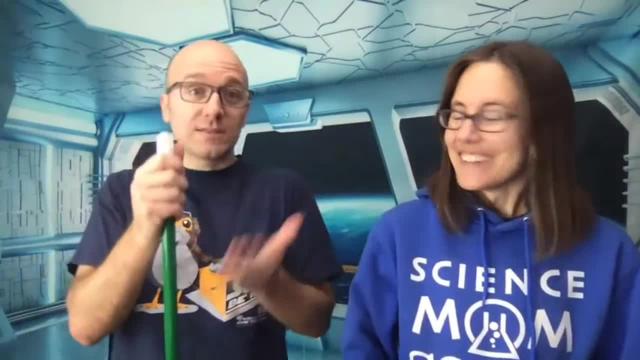 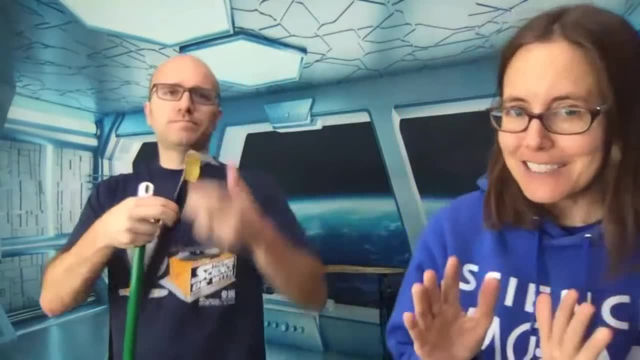 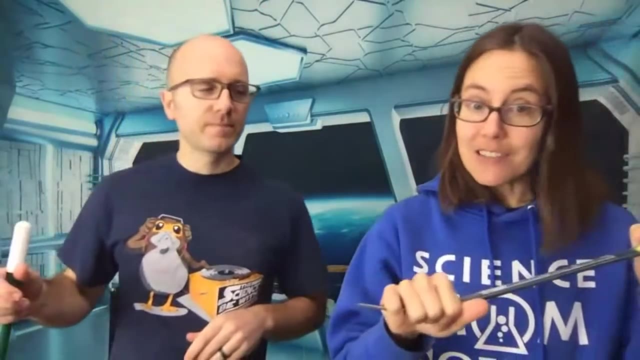 the last time i didn't have to sweep during a day. i'm using these type three levers all the time. um, okay, last one. all right, get ready to put your guesses in the chat. this is a crowbar, and when you use a crowbar, if you have something really heavy to lift that you need to pry up you. 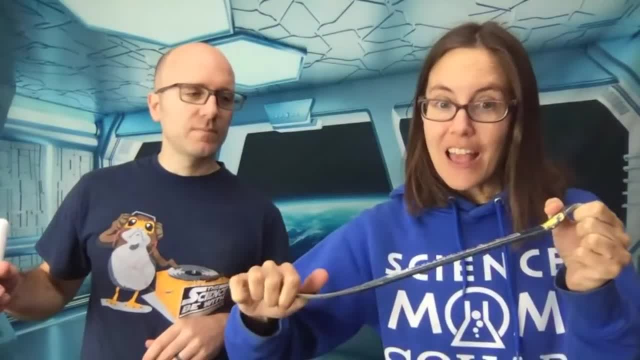 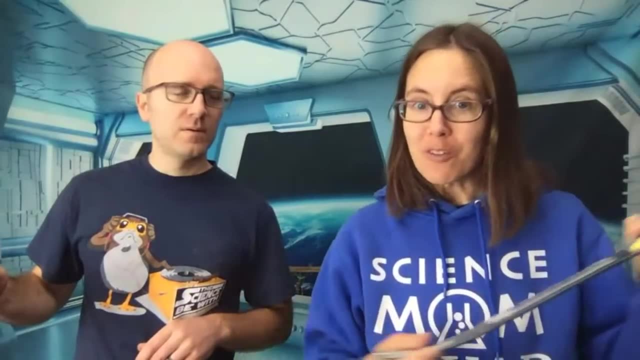 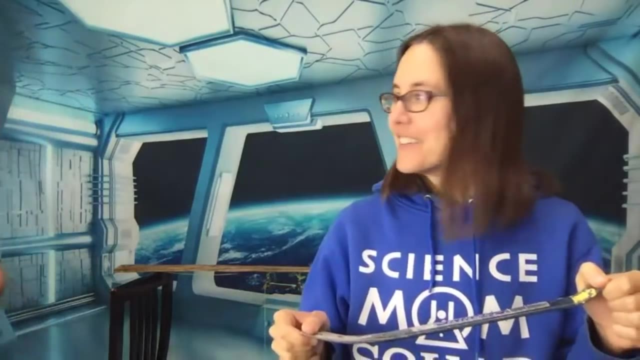 will stick it right here, your heavy object is here, and then you will push up to get, or push down, depending on what action you want to get your object to move. so what type of lever is this? what type of lever is a crowbar or a pry bar? it wasn't actually the description i was. i was 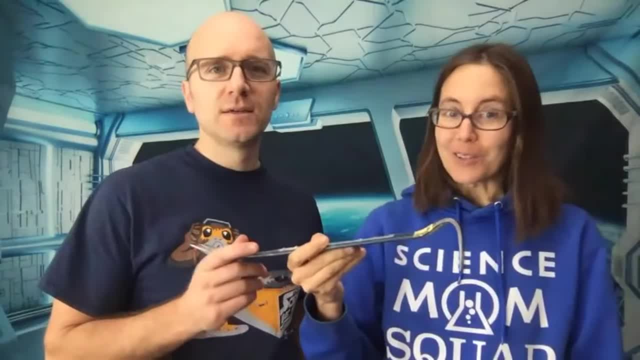 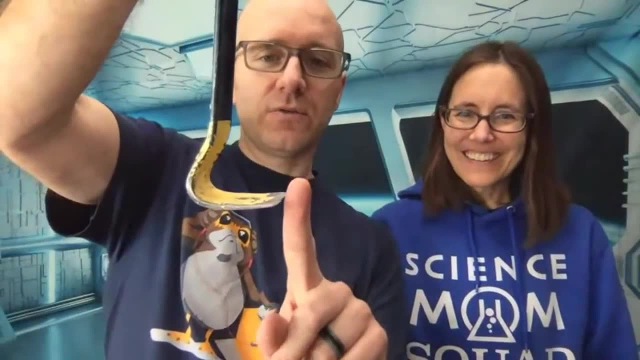 thinking about pulling out nails. all right, you tell them how you pull out nails with this. yeah, well, now, now that you've already given that other one, i'm going to go ahead and do it now. yeah, yeah, the other description, okay. so, so, how? how does it work when you pull out nails? so if 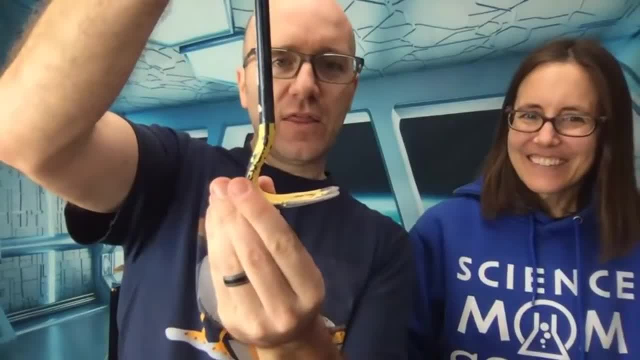 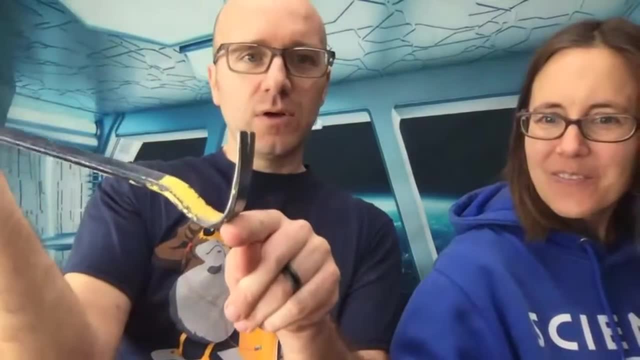 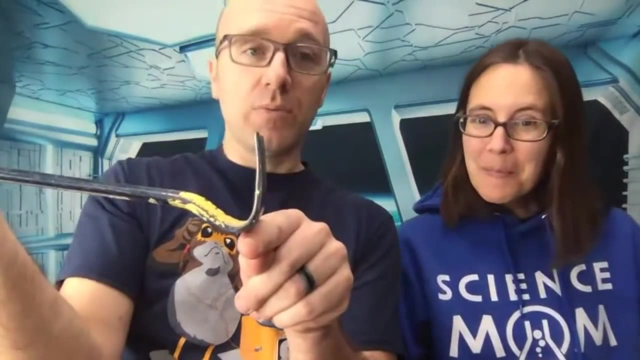 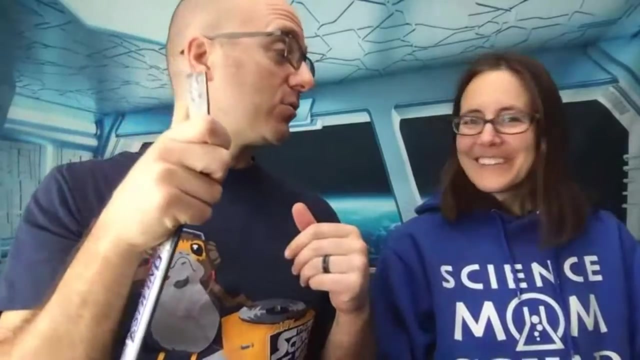 there's a nail head sticking up. you catch it on this end and then the bottom here is resting against the ground and we rotate like so. so the nail lifts up right there. so sarah says class two okay. so so well, i don't know if she's responding to. 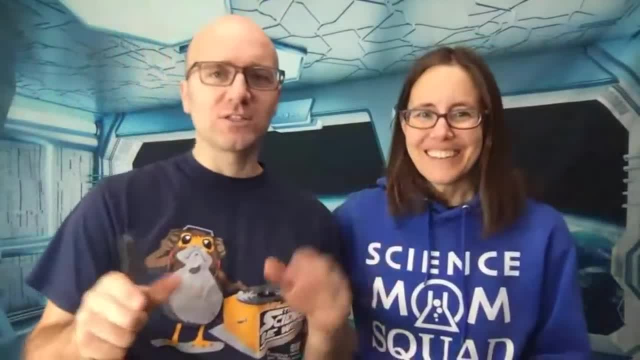 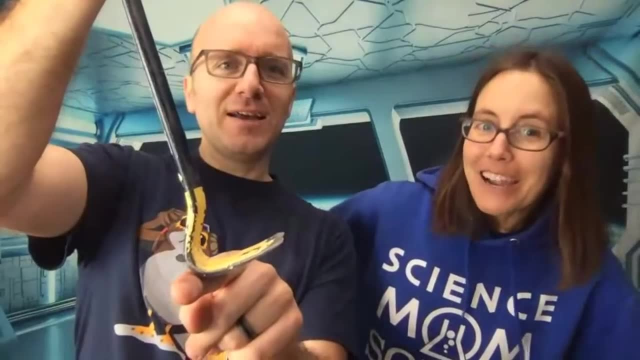 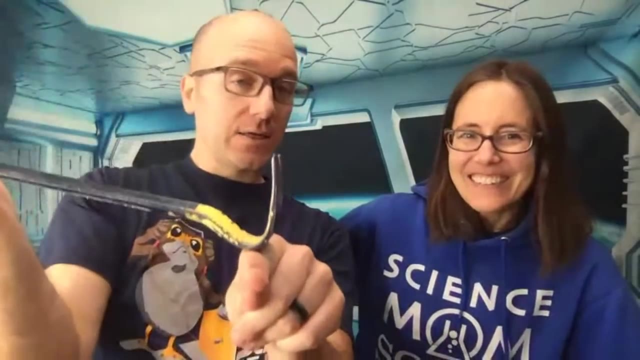 you had described or what I had described, Yes, Okay, So we've messed up the question now. So what I'm describing, Go for. what science math dad is saying: I almost called you science dad, Upgrade, All right. So this would be a type one lever, because the fulcrum is in the center. 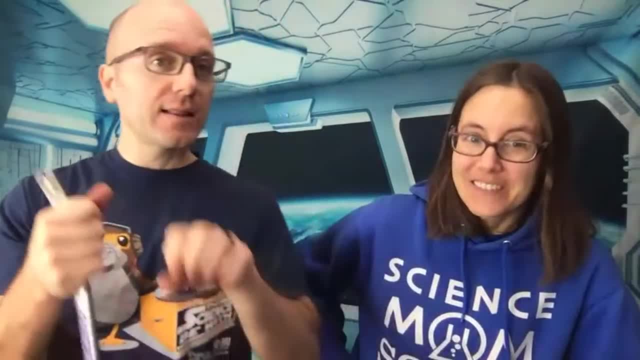 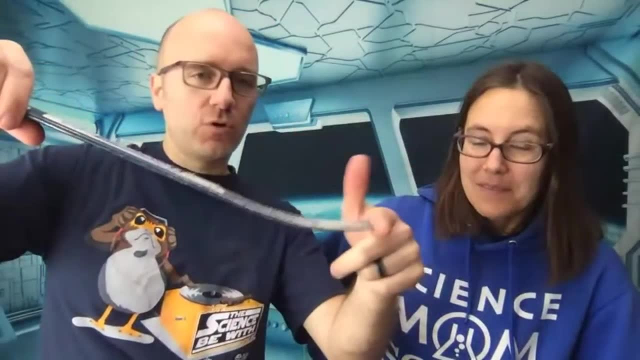 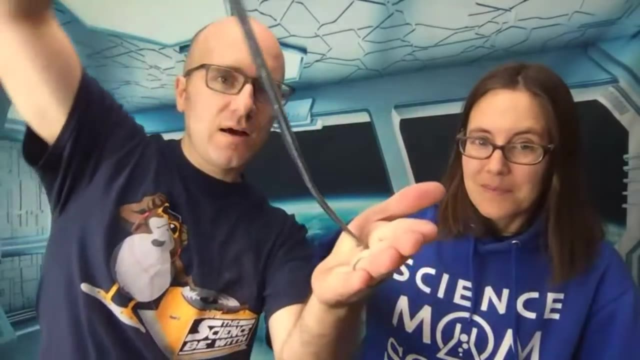 Now what science mom was describing sounded a lot like the way I was using the rock bar to lift the wall where we wedge this underneath. So the fulcrum point would be at this end, and the object is here And so it's going to rotate up and lift. So what type would that be? That would be a class. 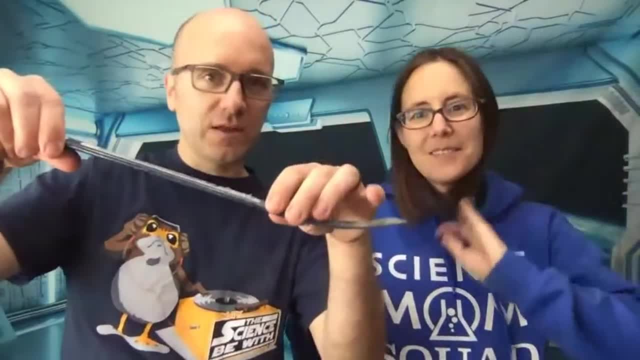 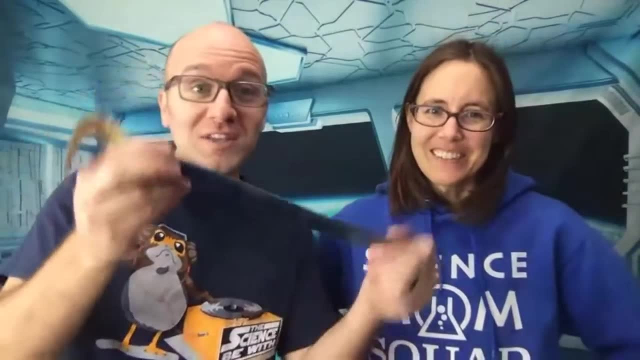 two. That's right, That's class two because the object we're lifting is in the center. So yeah, it's actually kind of cool. I thought there was just one answer to the question: What type of lever is this? Well, it depends on how. 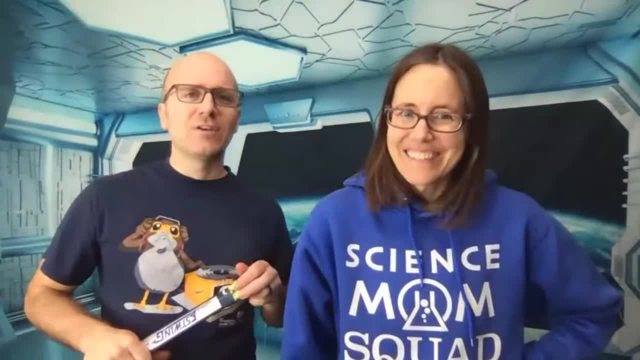 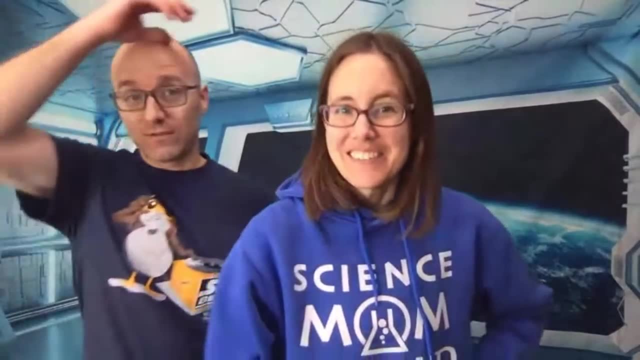 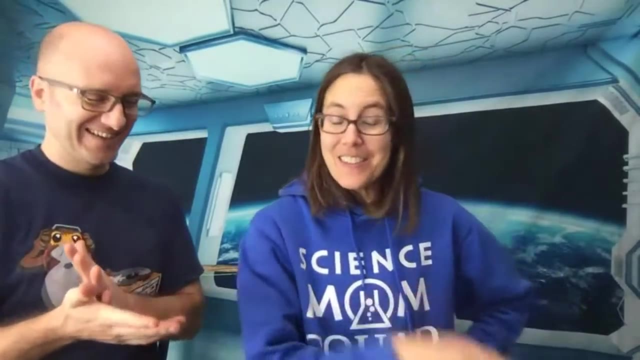 How do you use it? How are you using it? Indeed, So yeah, even something as simple as a crowbar, there are multiple answers or ways of thinking about it. One of my favorite little expressions is: work smarter, not harder, And this applies to simple. 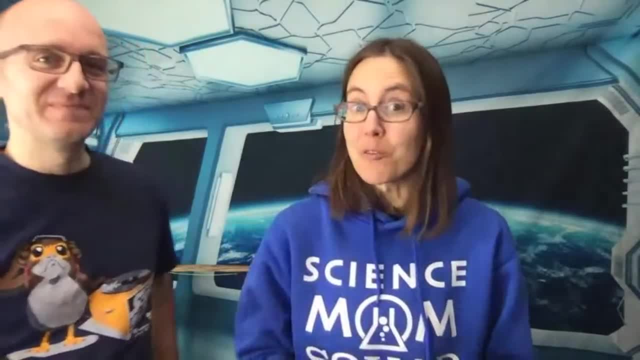 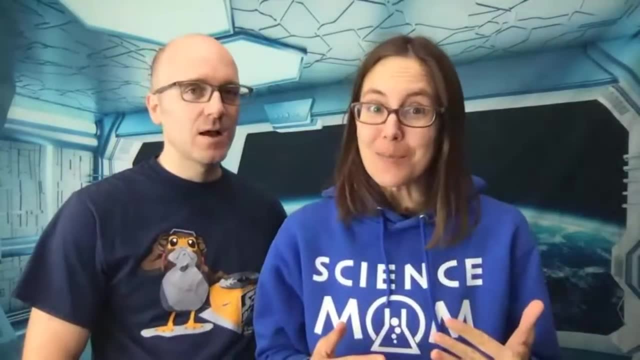 machines so well. There are a lot of ways where you can just apply more force and work harder, but you're not going to make a difference. But if you work smarter and you adjust and use a simple machine, then And the job becomes so much easier. And with that in mind should we move on to talking about 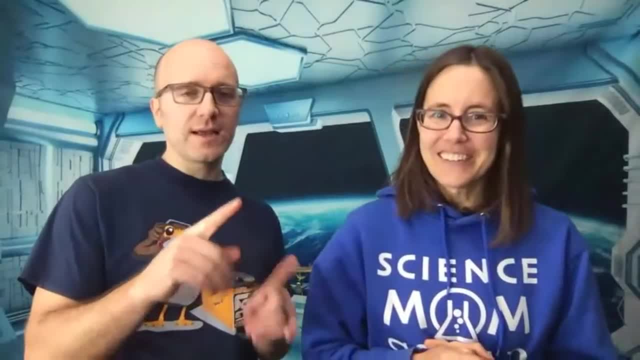 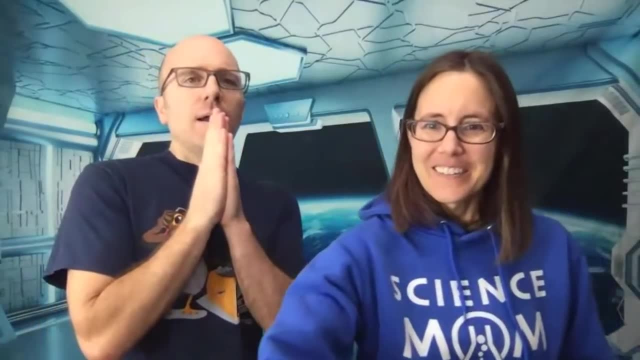 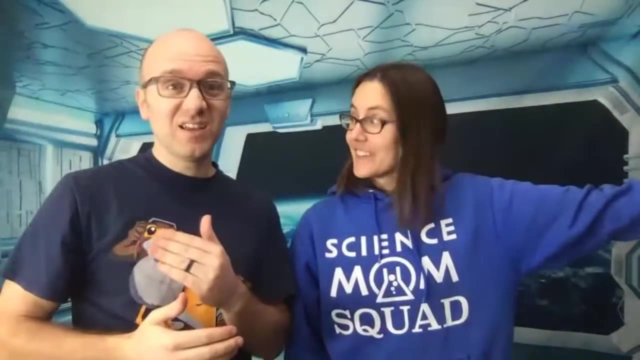 pulleys. Well, just one more thing to say about levers, And I actually do want to maybe revisit some of the math involved, but we can do that more in my math lesson. Your body is full of levers. Every joint in your body that can move it's using a lever, So you'd actually have to know how the 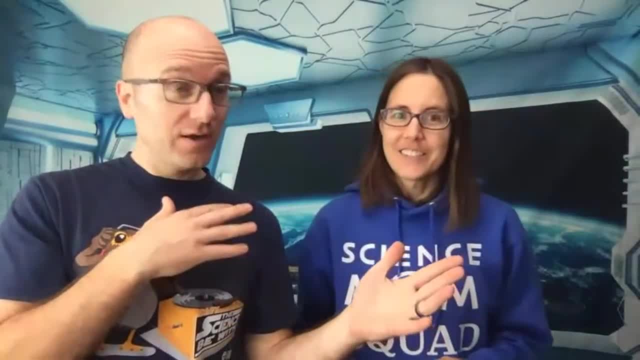 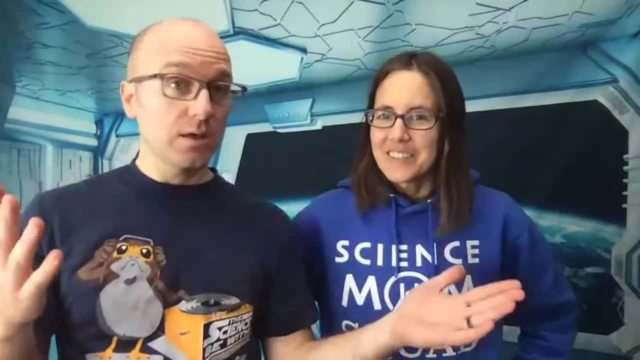 muscles are attached to know which type of lever It is being used- And I don't know the muscles that well or how they're actually attached- but all three classes of levers get used in your body. So yeah, when I say 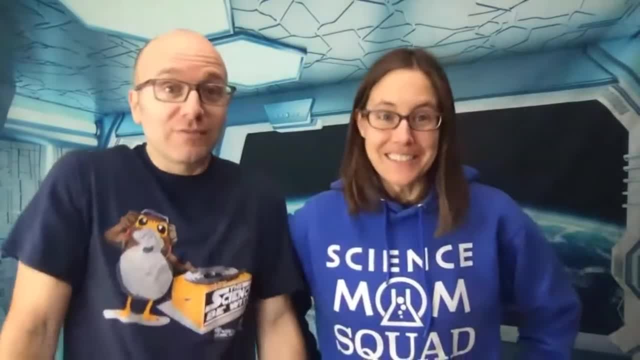 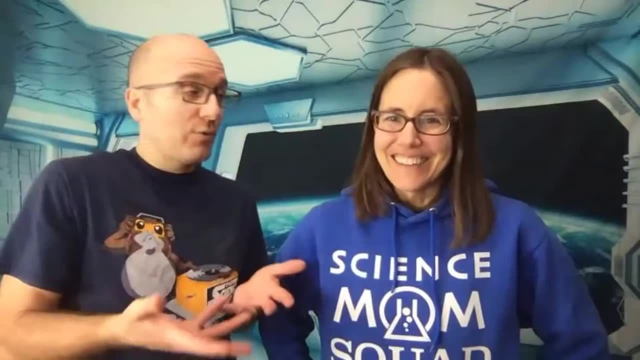 huh, I bet I use levers every day. I bet I use levers anytime. I do pretty much anything other than lie still and think Because, yeah, that's exactly how we move and how we get around. Now Jennifer asked what this board is behind us And to explain that, 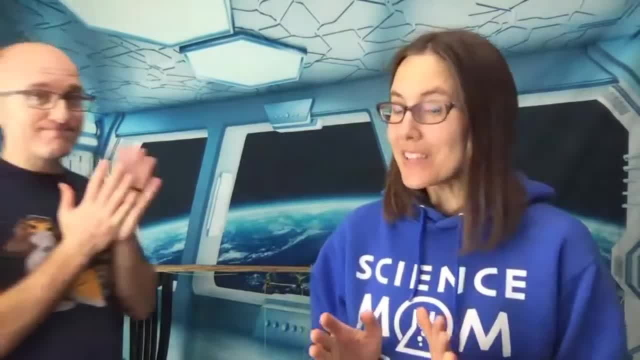 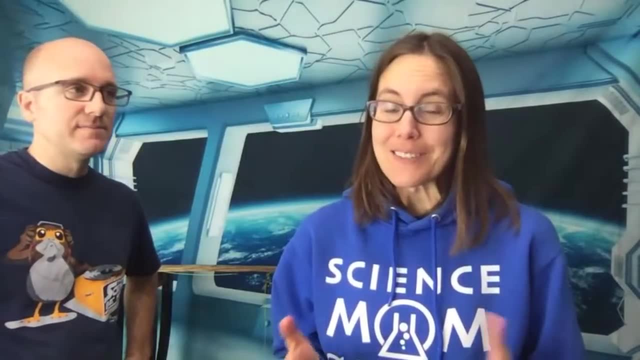 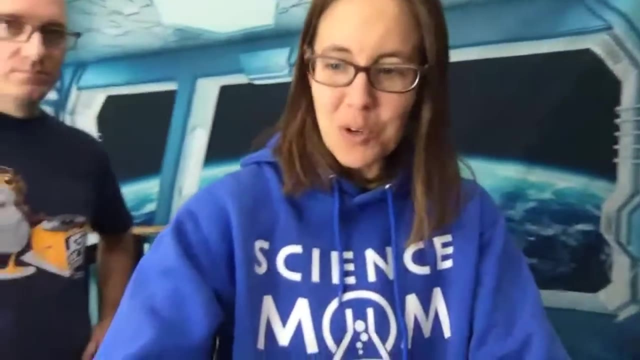 we're going to talk a little bit about pulleys now. Pulleys are amazing And the type of difference that you can make to the work that you're doing with a pulley is really just incredible. So I'm going to shift our view down just a little bit So you have a slightly better view of this board. 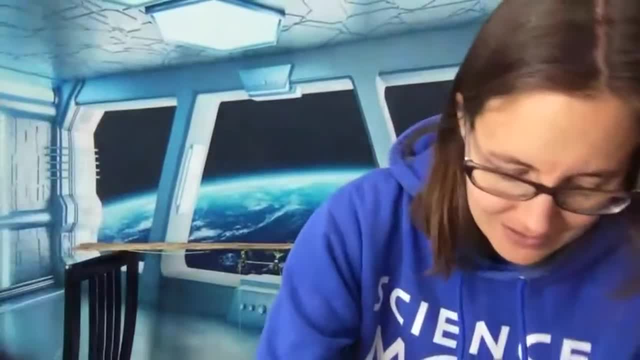 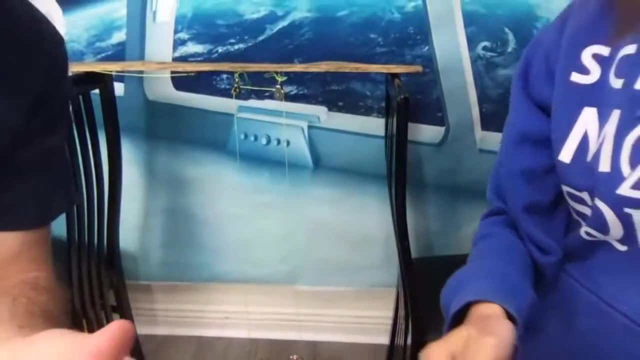 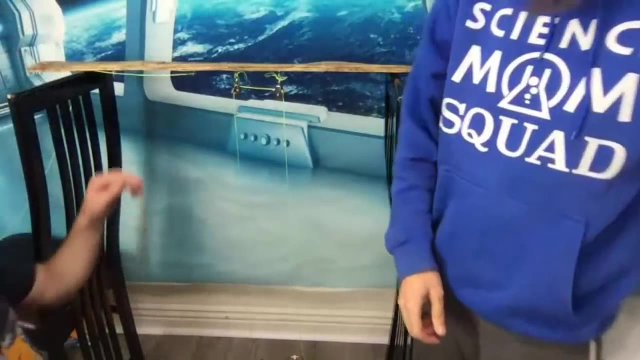 right here, And then let's explain how a pulley works Just a little closer. So here we have a green string And spoiler alert: we're not really in space. You can see that we're not in space. You can see the bottom of our backdrop right there. We're not going to be in space this whole time. 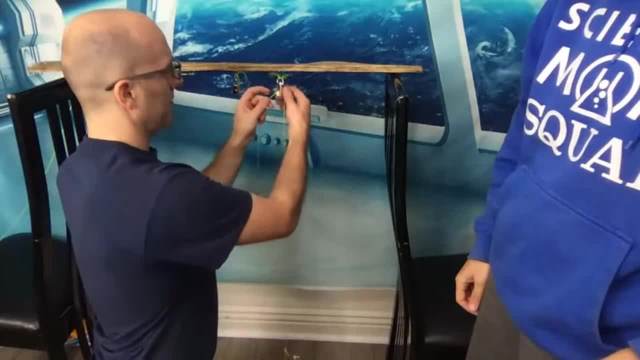 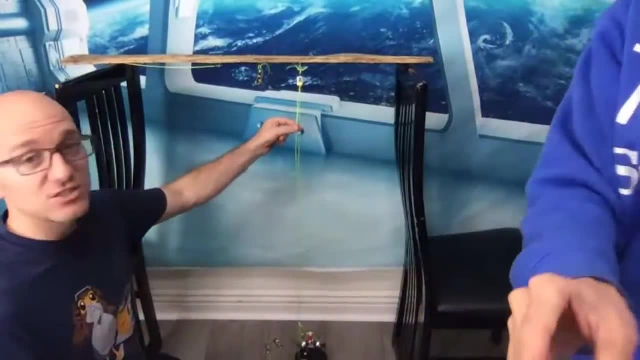 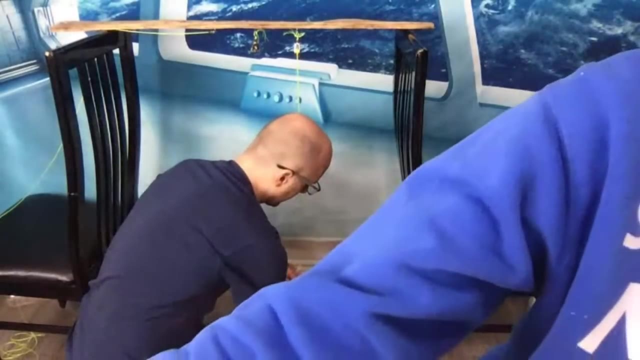 Okay, So I have here. so this pulley is just this nice spinning wheel. The idea is, we want to minimize friction And we have this thin string which actually barely shows up on the video. Kind of unfortunate. All right, So we have this clock, which we bought solely for 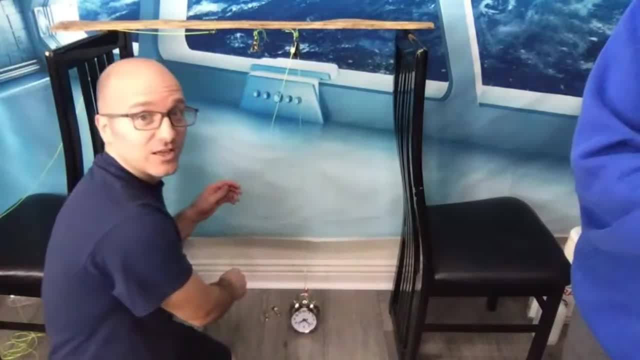 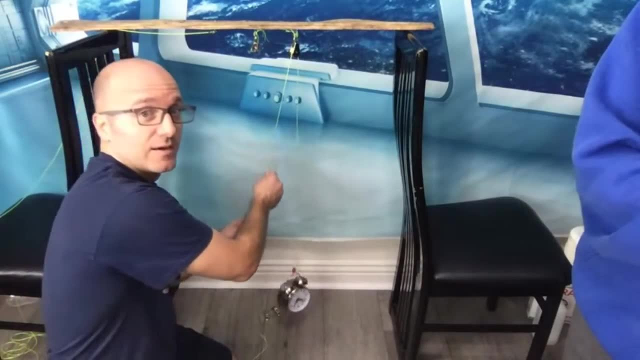 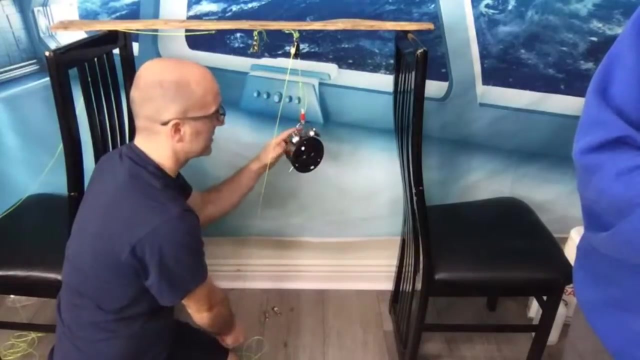 ringing in a vacuum chamber. So now we're going to use it again here. So I'm going to lift this up by pulling on it, And what this pulley has done is it has just redirected the force. Now, did I have to lift as hard to get this? 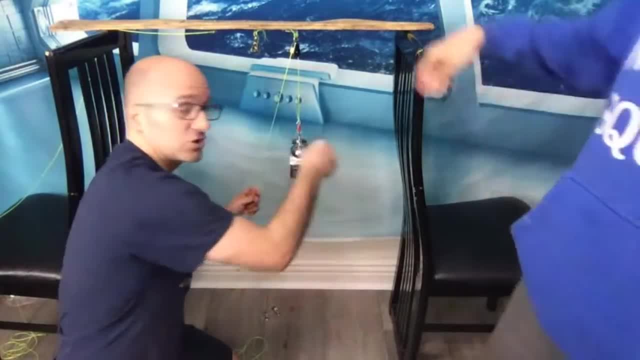 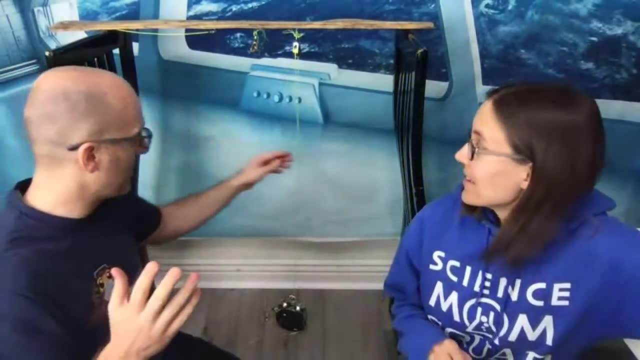 clock to go up, as I would have if I were lifting straight up? Well, the answer is yes. All I've done is redirect the direction of the force. It still weighs the same amount. However, I can use my body weight, And this is really useful If you're lifting something and you have 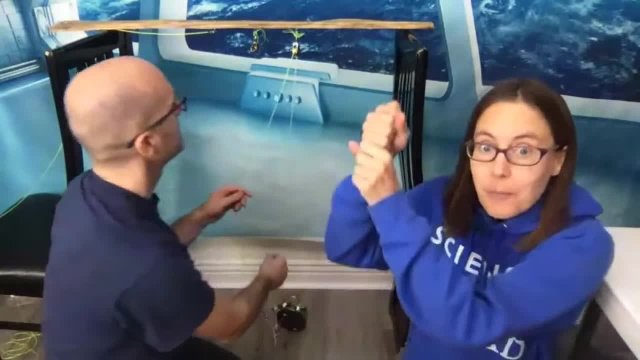 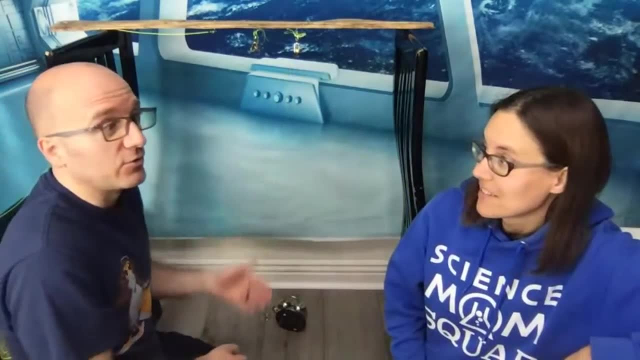 to just lift up. that's a lot more work than if you can pull down, because you can put your weight into pulling down Absolutely Well. not only that, but when you do lift, you have to actually lift your body weight. So I'm not just lifting the clock. when I lift the clock up, I'm lifting my 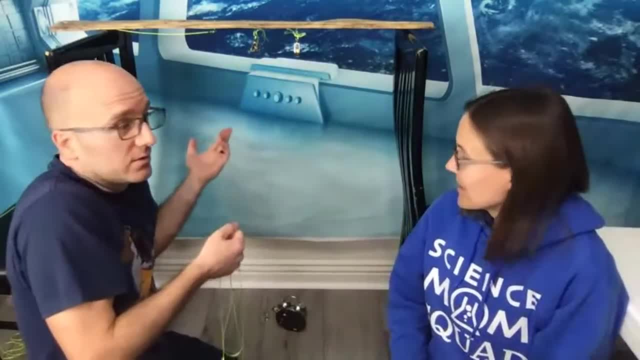 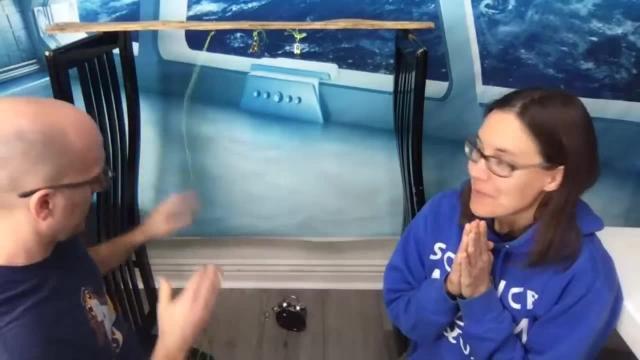 body weight, Whereas if I'm pulling down, I can use gravity to do a lot of the heavy lifting for me. But there's a way that we can make this a lot easier. Indeed, there is, So I'm going to feed this through a pulley. 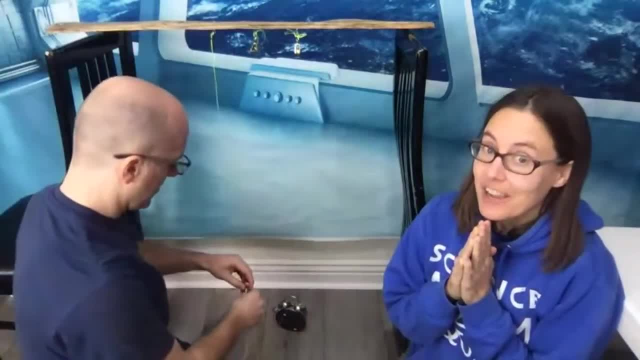 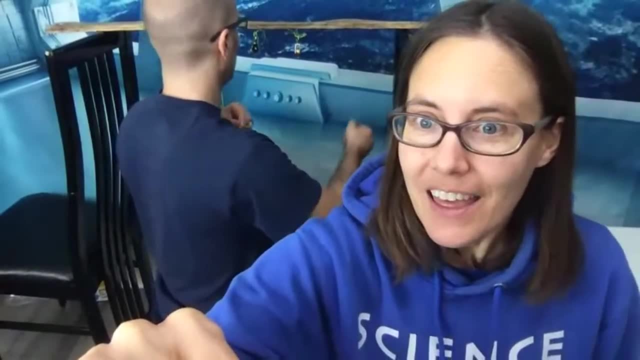 And if you're curious, because our engineering challengein fact I should pull up this slide while Math Dad is getting this ready- Our engineering challenge today is to make a pulley, And if you don't have a pulley from the hardware store, you can make your own using materials just. 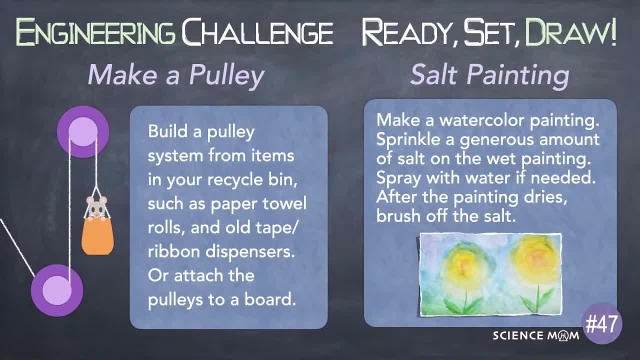 from your recycle box. So the main thing that you need is something that will spin, and you can take a wheel from a Lego box. you know Lego collection. You can find an old wheel or you can make your own wheel by just taking two materials that will slide around each other. that 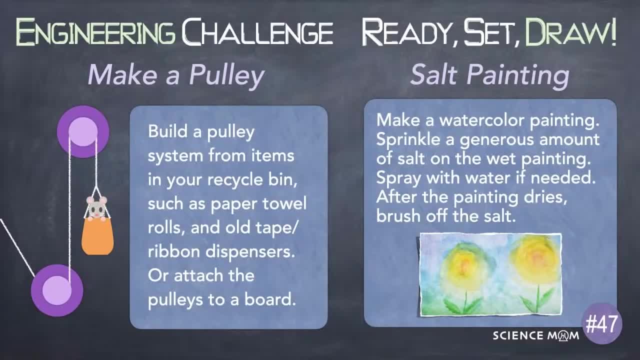 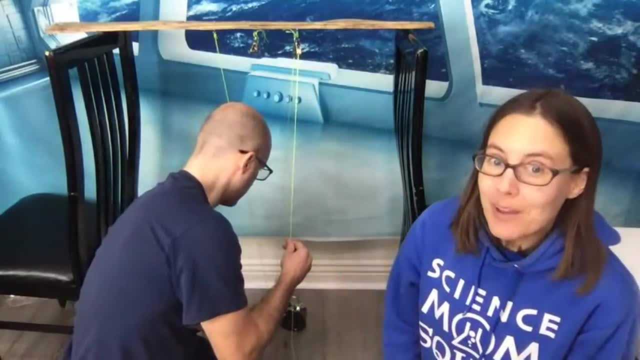 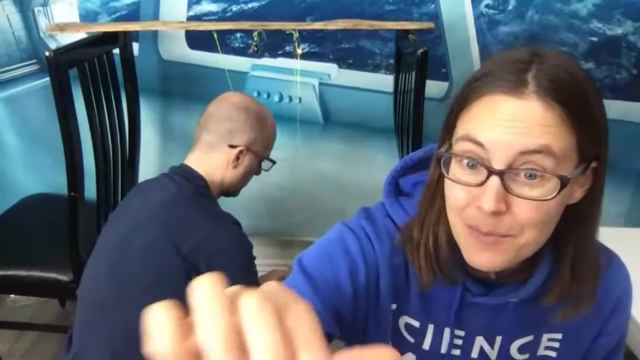 are both round and then putting one inside the other. So making a pulley is our engineering challenge for you for today, to get materials that you have at home and see if you can set up a simple pulley system. And, like Math Dad pointed out, it can be as simple as just. 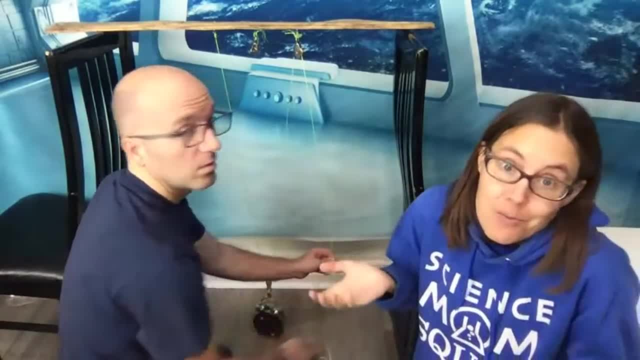 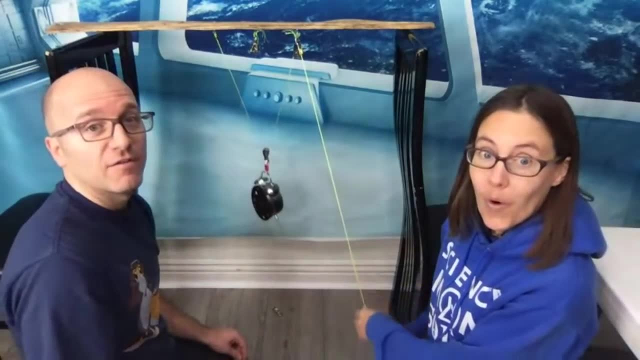 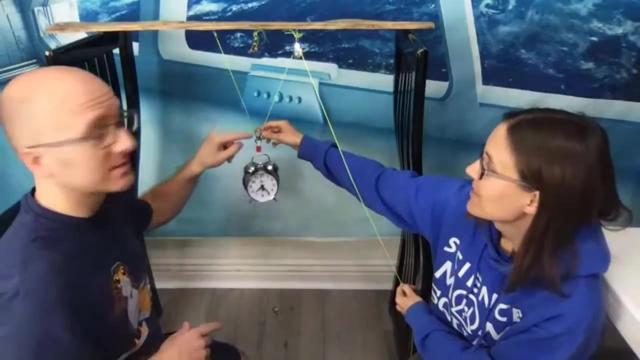 a rope going up over a round thing and then back down. That reallythat's a pulley and it's just redirecting the force. But if you have two pulleys, So now we have a mechanical advantage working for us. So we have these two different pulleys and something interesting happened here, Actually, 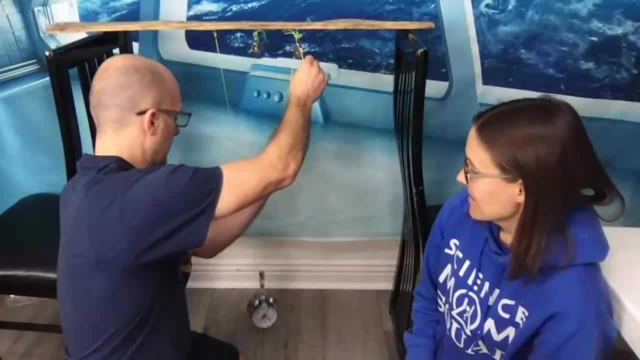 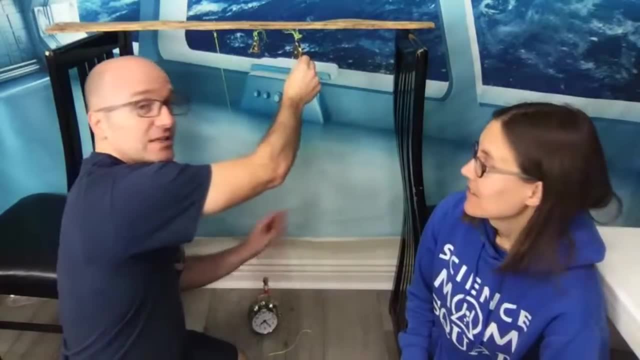 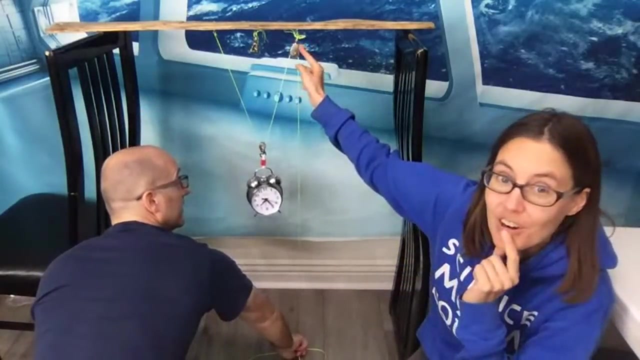 I'm going to lower this back down all the way to the ground, All right. And now I'm going to take the string right at the top and I'm going to pull all the way to the ground. And how high is that going to lift the clock, Pay attention. So he pulled the string from here all the way down to 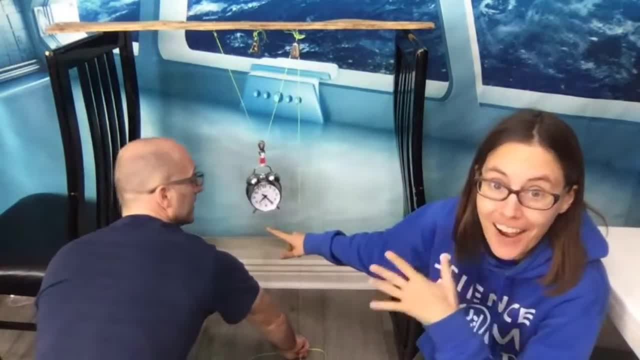 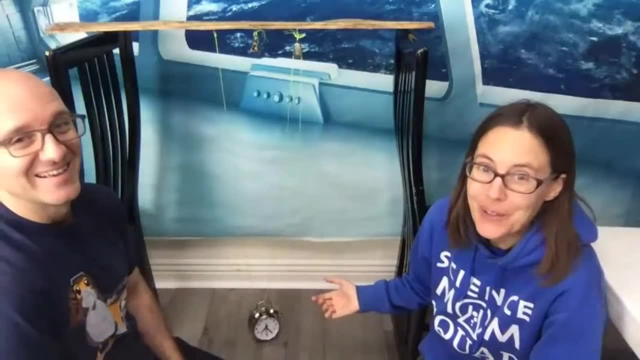 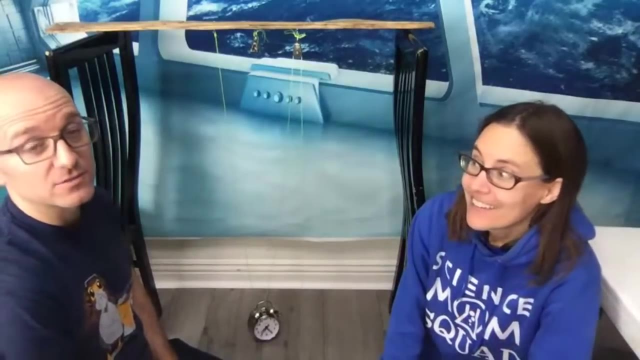 the ground and the clock only went half as high. And this is really where the magic, or the, you know the physics of the pulley- works, because you have to pull twice as long, but the pull is twice as easy. That's right. So work equals force, times, distance is the 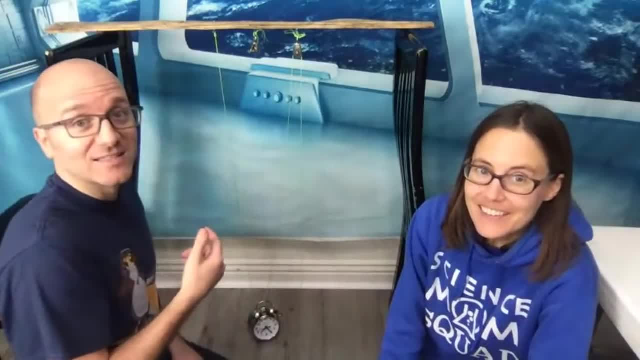 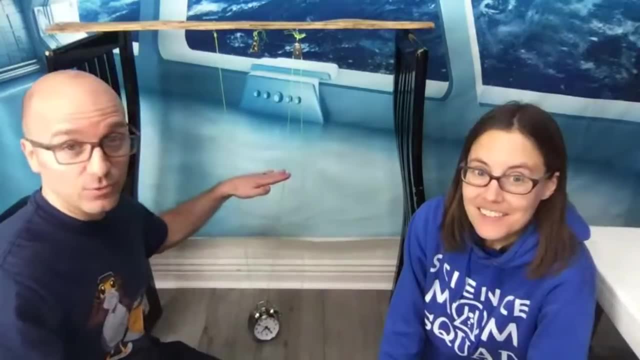 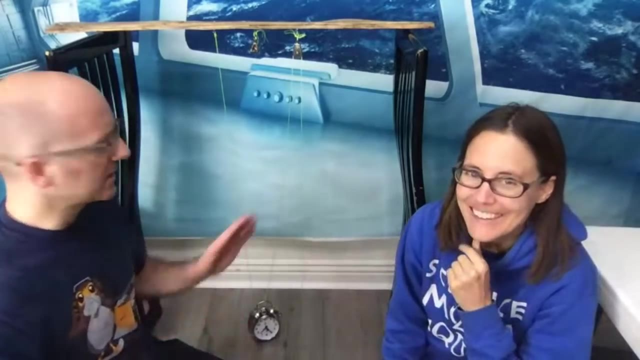 physics equation that's going on here. Well, in this case I just doubled my distance, so that actually ended up doubling the work that was accomplished. Should we show them our fun videos that we filmed this morning? Sorry, Let's do this. Yes, All right. So we thought that this would be. 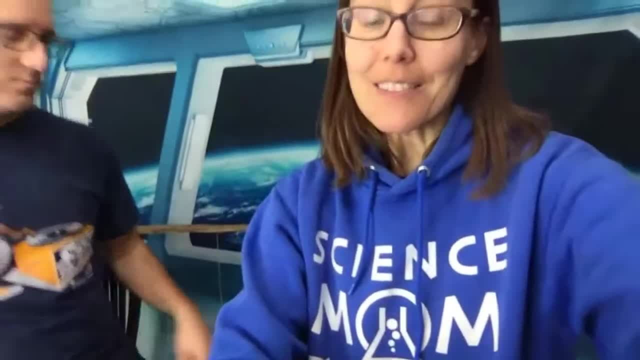 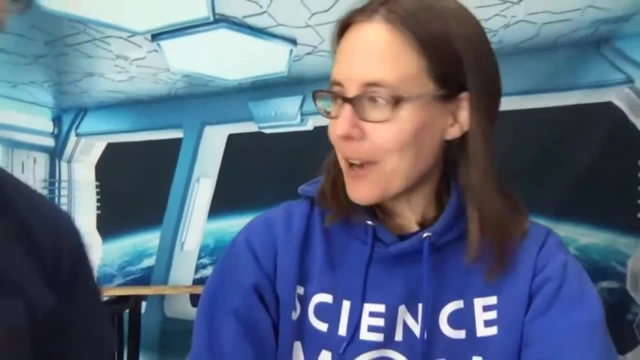 much more impressive with showing you a five pound weight lifting up a 10 pound weight. We're like, oh, this is going to be so cool. It ended up being a little trickier to troubleshoot because our strings kept sliding off of the pulleys, So we filmed a couple of videos. 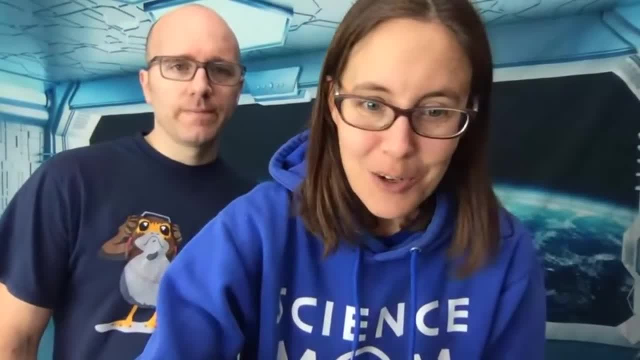 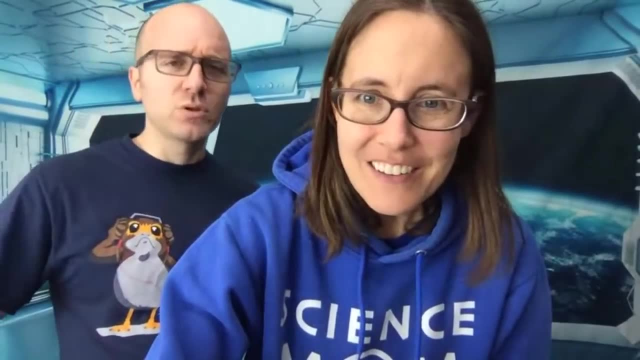 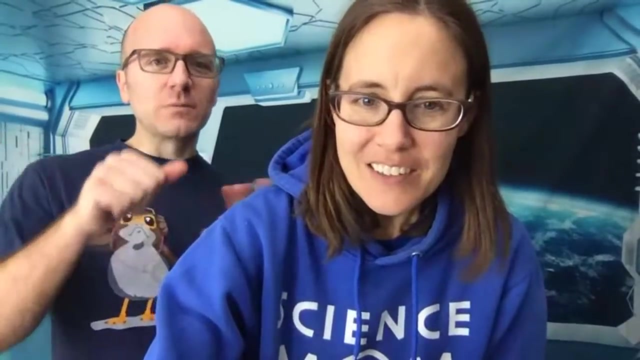 in advance that we're going to share with you. now, Here we go, Anything you want to. No, I mean, it took some finagling to actually get the pulleys to do what we wanted, And there is friction involved. I should mention that. So with friction you're actually losing some. 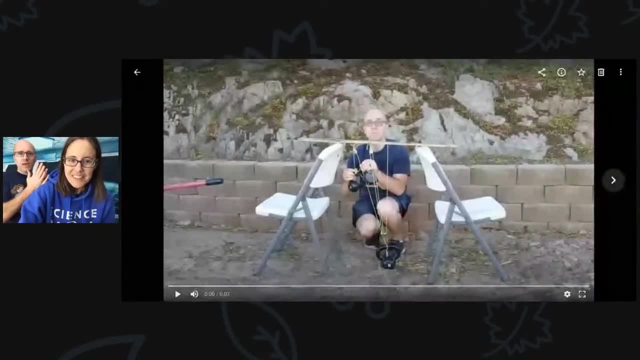 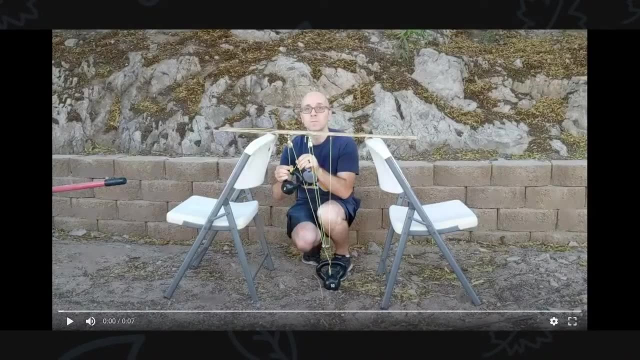 of the effectiveness. but yeah, So here we are. We took our All right. I've got a blooper for him first. Oh, So first you get to see the blooper. So we were all excited And it's like this: 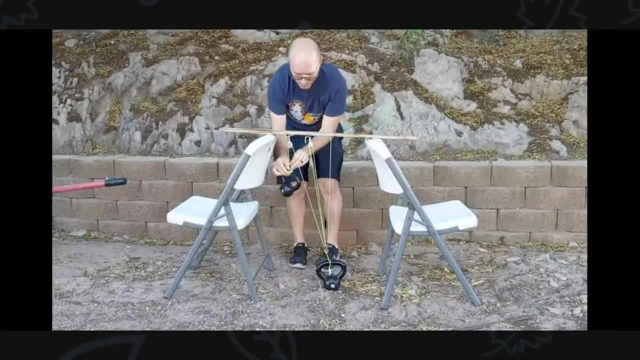 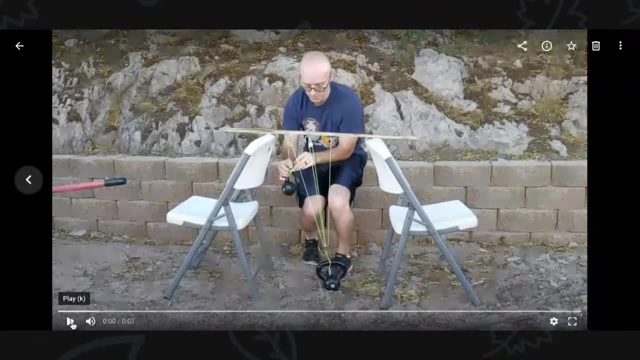 Whoops, It broke. That's kind of funny. We're going to watch it one more time. This is why we did it outside, because this would have cracked our tile or damaged our floor. And I will say: if you are doing heavy weights with pulleys, eye protection is a must. And 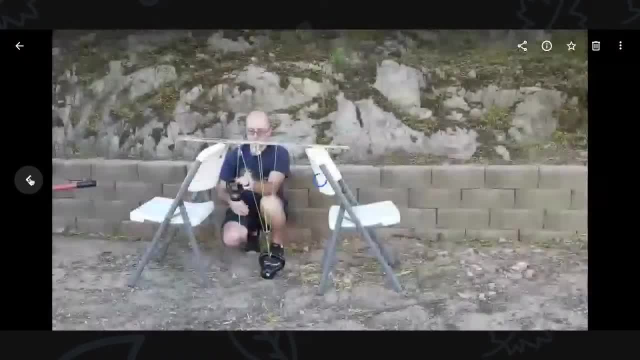 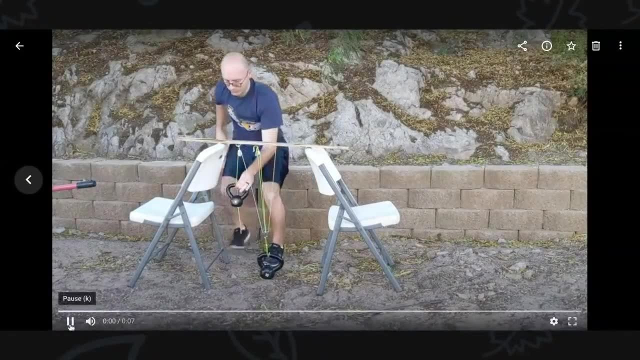 Math. Dad's glasses don't quite count as eye protection, but we'll forgive him. We'll forgive that, All right. Next one. All right, What do you have? I'm waiting for it to load. Here we go. So five pound weight, Drop it down. It lifts up the ten pound weight. 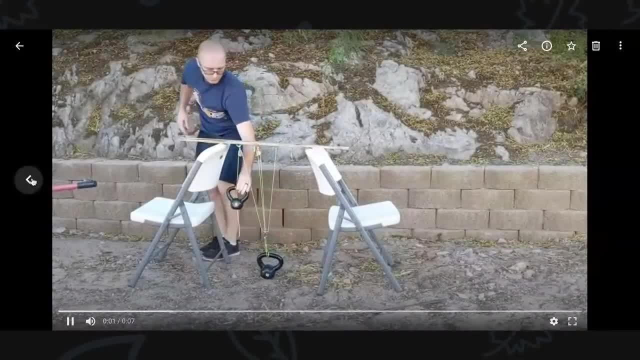 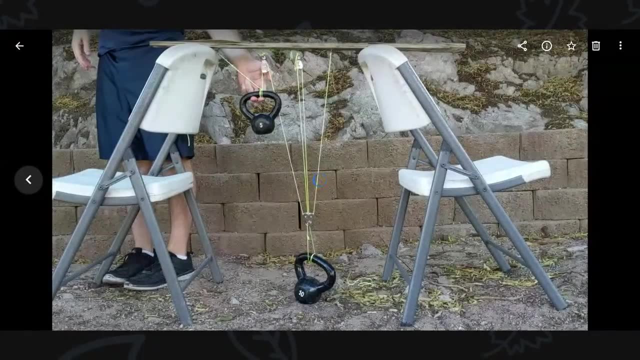 So in this case the five pound weight was able to lift the ten pound weight, BECAUSE- I don't know if you can see here- we have multiple pulleys there, So there's one, two, three, four pulleys involved, And this one's even better. 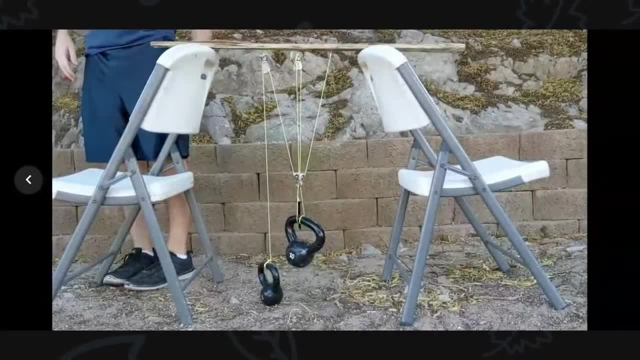 because you can see it going from the very top. It travels all the way down, It lifts that two here And then you have the octopog in the knee: resistance. Yeah, Yeah, Yeah, Good, Yeah, Yeah, Yeah. 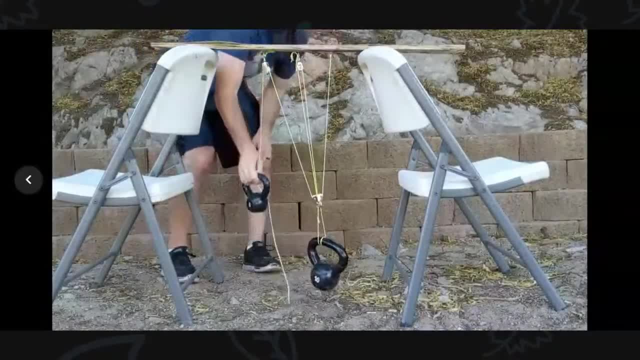 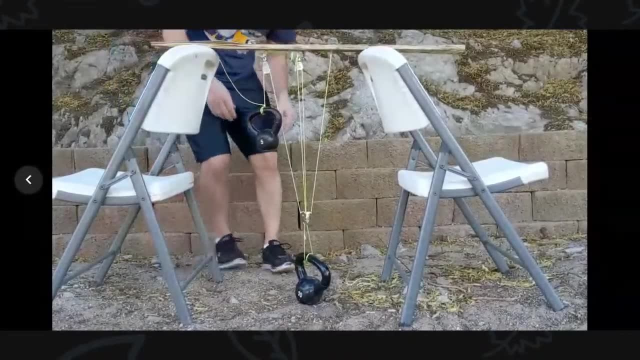 Yeah, Yeah, Okay Yeah. down lifts that 10-pound weight. Look at how much farther the five-pound weight has to travel. So five pounds is pulling up 10 pounds, but it has to travel. Oh, and there the string got stuck. 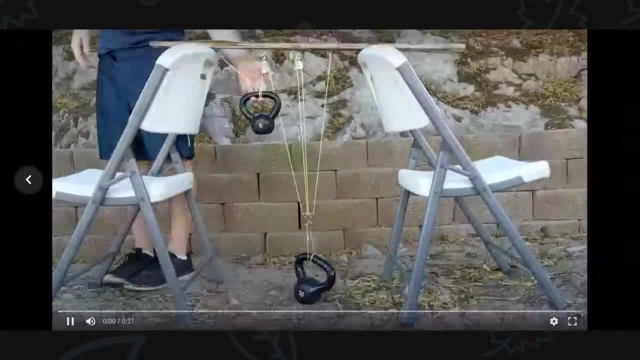 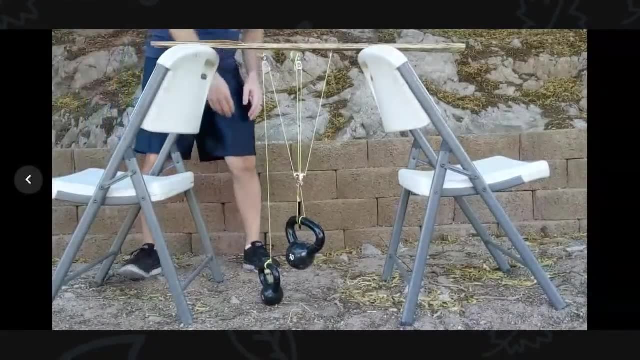 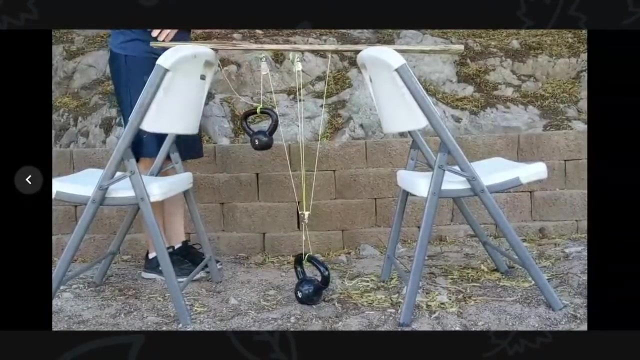 again: Yeah, So in this case our mechanical advantage was four times stronger, but that means we only managed to lift it one-fourth as far. Yeah, So in other words, the lighter weight there had to travel four times further to get down than the heavier weight got lifted up. So 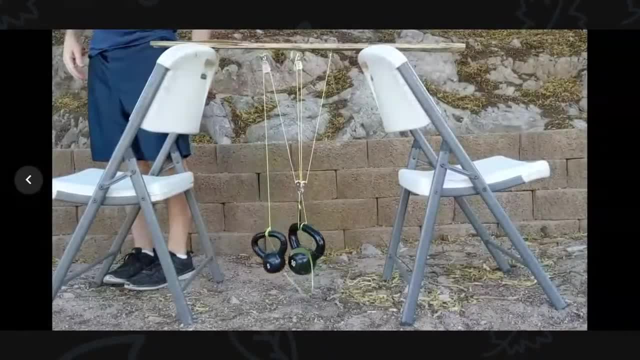 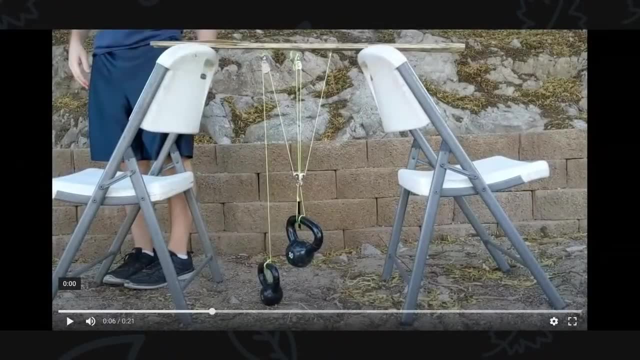 there's a price to be paid for getting that mechanical advantage, but it ends up being enormously useful. Did you use pulleys when you were? Yes, In fact, I was going to go grab some pictures while you do your math lesson, but isn't this so satisfying. 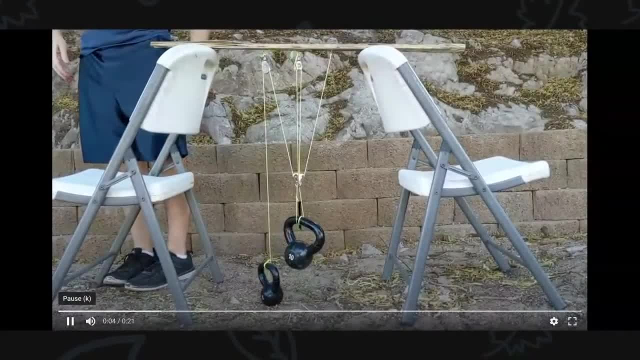 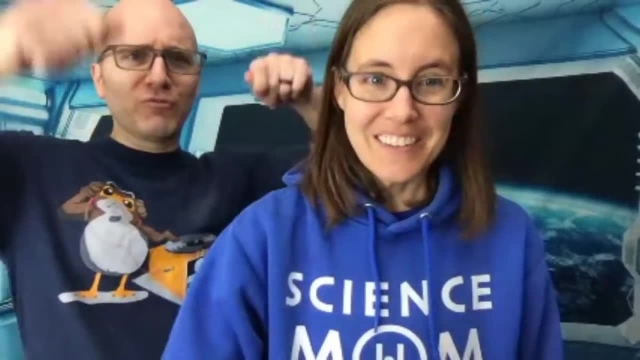 Satisfying. Five pounds, lifting up 10 pounds and then the way that the little string gets caught and flips down, I think is kind of funny. Yeah, I mean it kind of sounds impossible when you think about it. Like, oh no, I'll just hook up a five-pound weight and a 10-pound weight and we 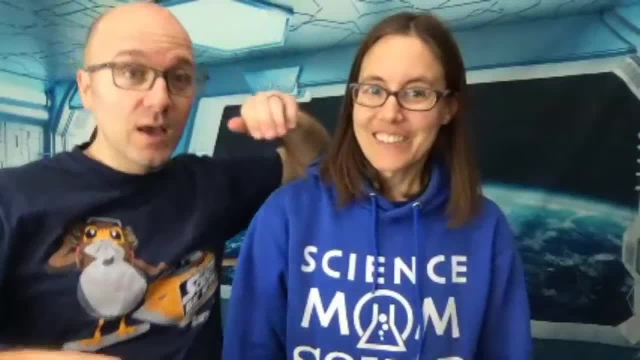 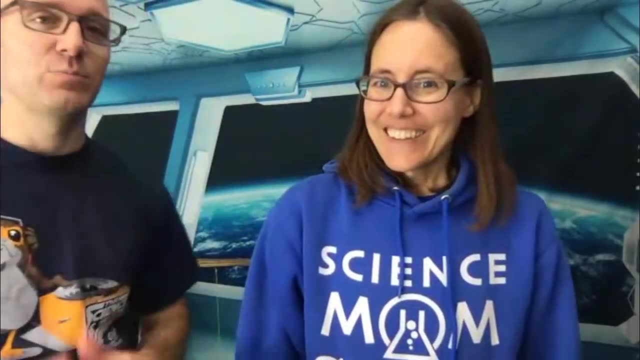 all know what's going to happen: The 10-pound weight's going to pull the five-pound weight up as the 10-pound weight goes down, but not if you've got it rigged the right way. So that's pretty darn cool. And Kathy asks if we tried a 10-pound and a 20-pound. We did not, And it turns: 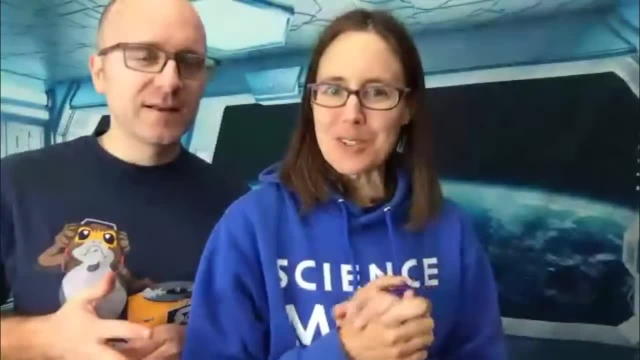 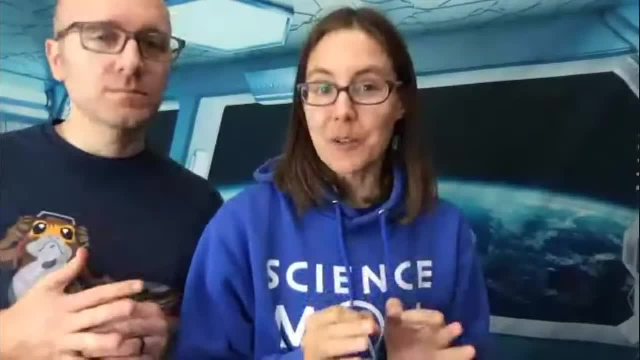 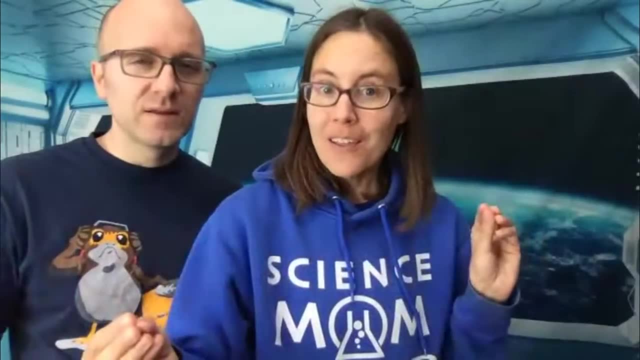 lesson. But with pulleys you do need to be careful because as you increase the weight- if you get to you know, several thousand pounds- there is so much tension on that rope that if one of the ropes breaks that can be really dangerous. So with just a five-pound, 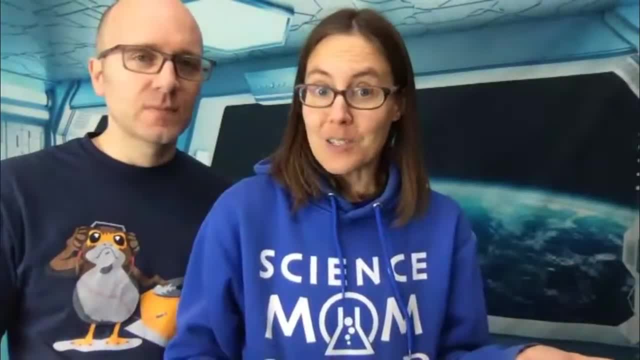 and a 10-pound weight, we're totally fine, And 10 and 20 pounds, we'd be fine as well, And it still would work just as just as well. Although our string was really small, We'd want a thicker. 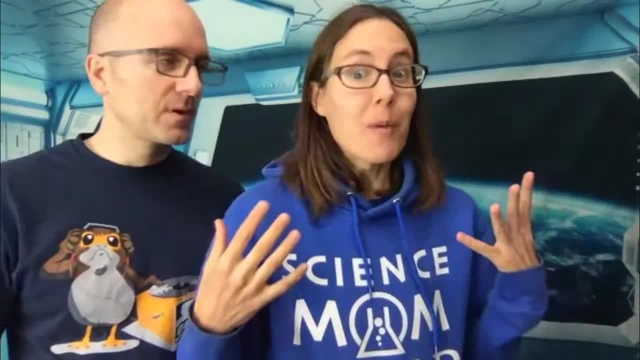 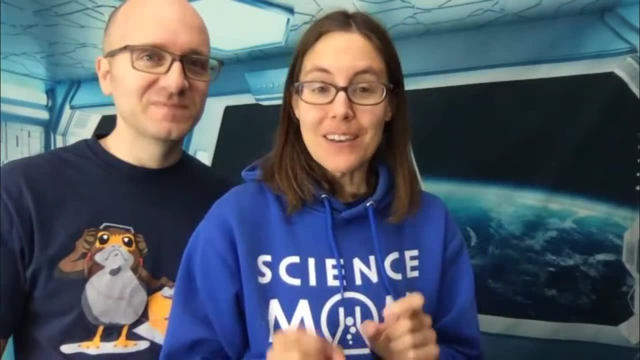 string if we were going up our weight. But if you get into the realm of a thousand pounds, when you're lifting things that are a thousand pounds, make sure that you've done your research and you know what you're doing, because accidents with shifting weight that big can actually be kind of dangerous. 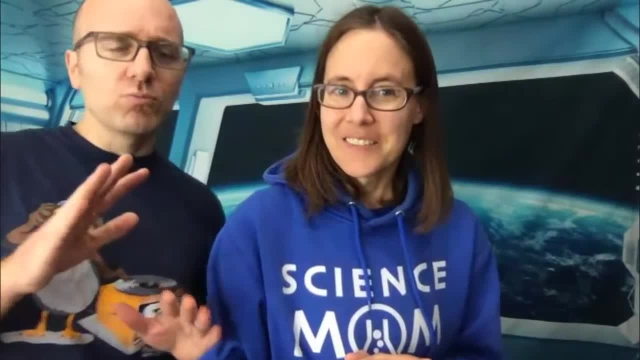 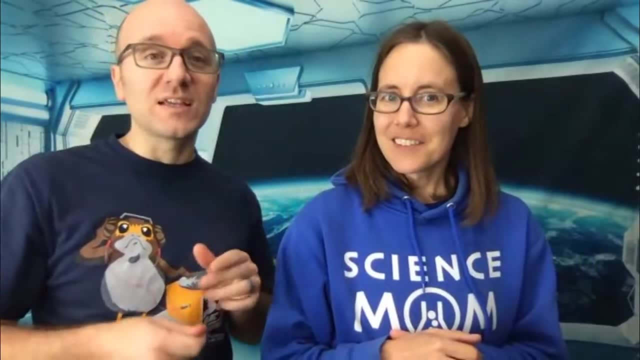 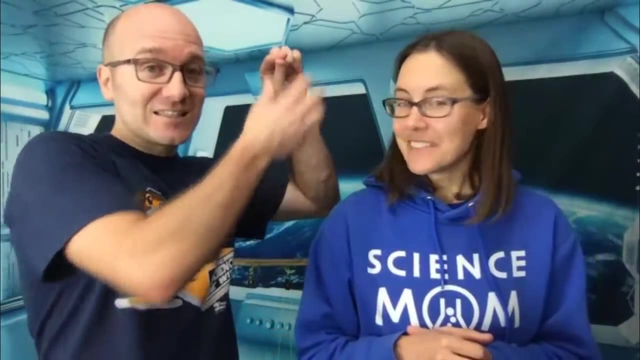 That's right And just as also as a- I don't know if it's a warning, but just a heads up. you can't just put, run the string through a bunch of pulleys and expect to get mechanical advantage. You actually have to hook them up the right way so that the distance that you're 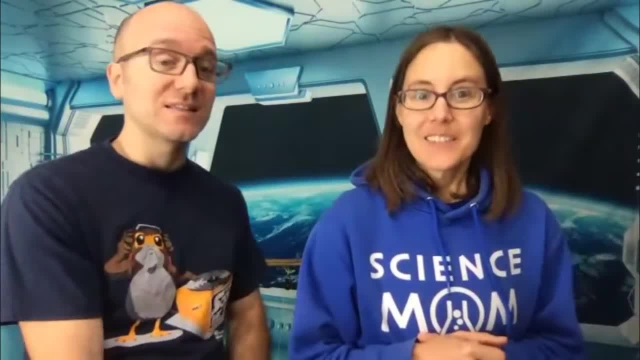 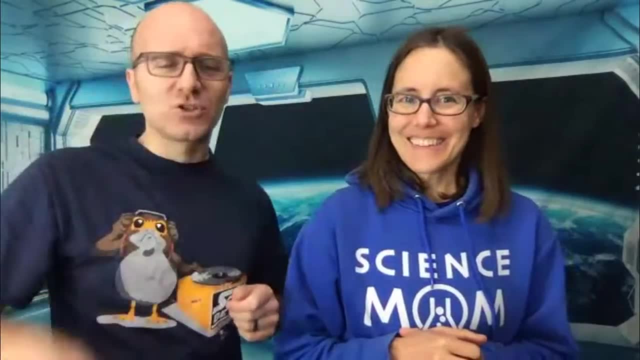 pulling ends up being much larger than the distance the object is actually moving, So it takes some thought. I just started trying to hook these together and run the string through them. Yeah, Okay, That didn't do anything. My first pulley system was a fail too, because I was like 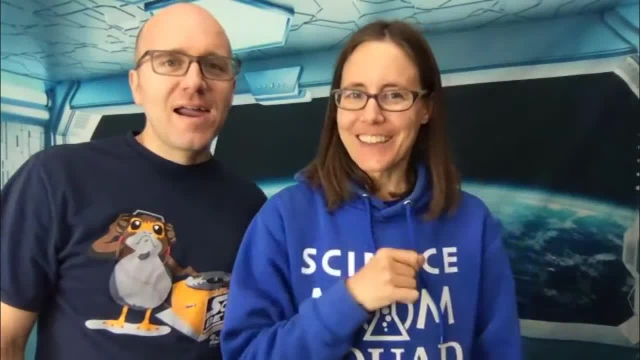 oh, I'll just make this cool up and down pattern. And then I was like wait a second, Yeah It didn't work, And then I had to redo it. Kind of fun, but yeah, it didn't didn't do much. 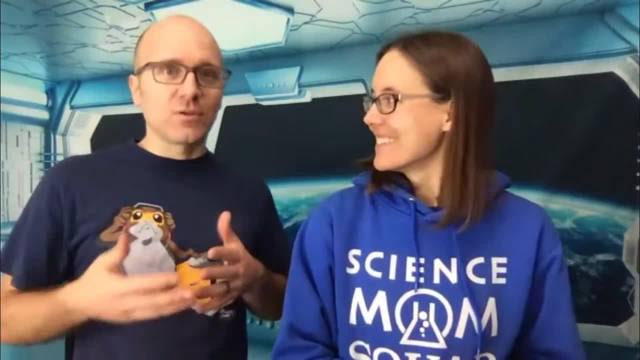 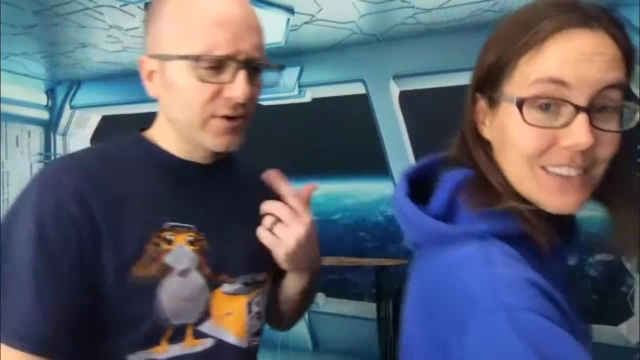 as far as gaining mechanical advantage. Yeah, Which is the whole purpose of these simple machines. All right, Math dad, I think it's time for fact or fiction. I'm ready, So I don't know, I'm giving you the fact or fiction. Math dad is giving me the fact or fiction. All right, Science mom, Fact or. 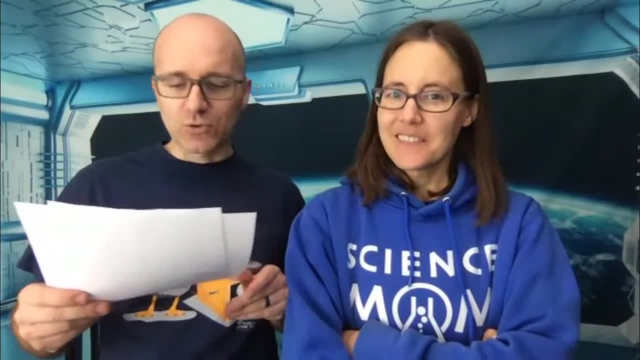 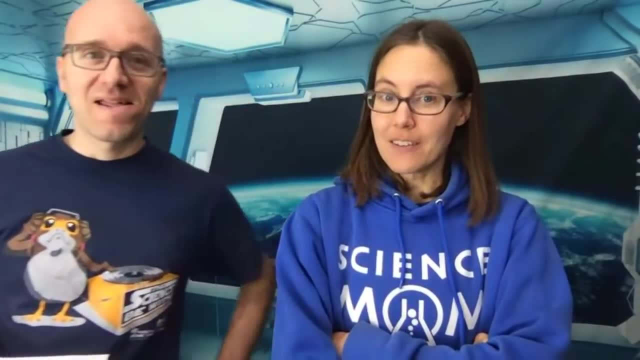 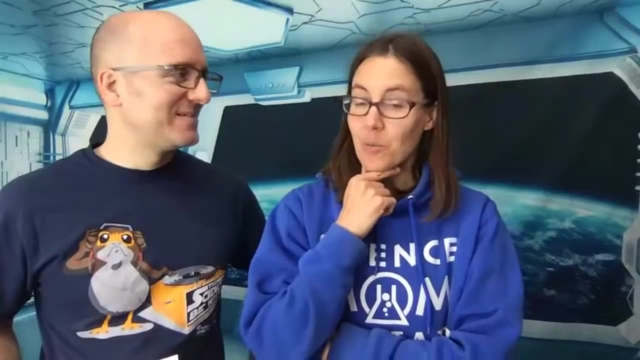 fiction. When light passes through water, its protons are only traveling at three-fourths of the speed of light. When light passes through water, it slows down, So the speed of light is a constant. Um, but water, water is pretty amazing. I think this one, I think this one is pretty amazing. 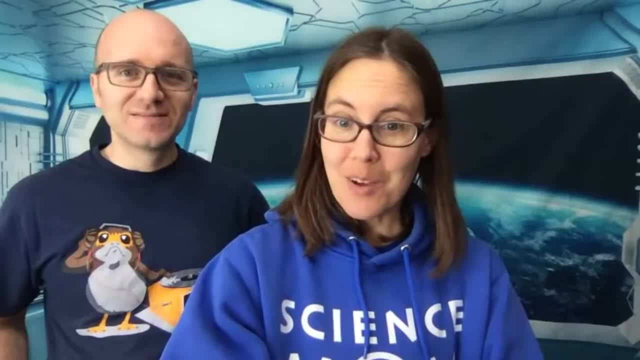 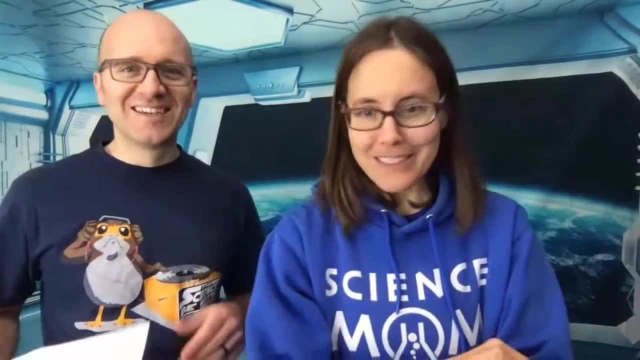 This one is true, I'm hoping. Carrie says true. I'm hoping for some more effort, more grace Gaming wolf says false. David says: trust me, it's true. I'm going with David. All right, It's true, I think. 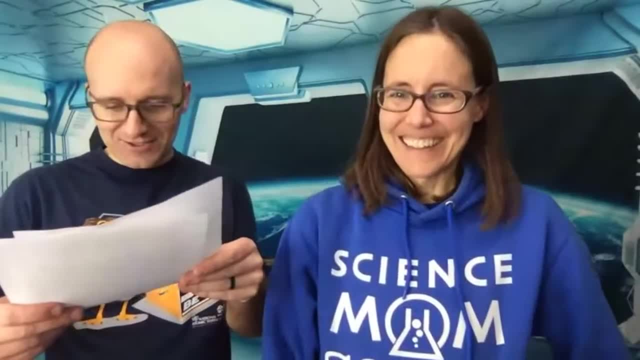 he tried to lead me straight the other day, but I'm not, I'm not, I'm not sure. but um, okay, So this one's actually true. So what science mom said out loud is is often the short version, Oh. 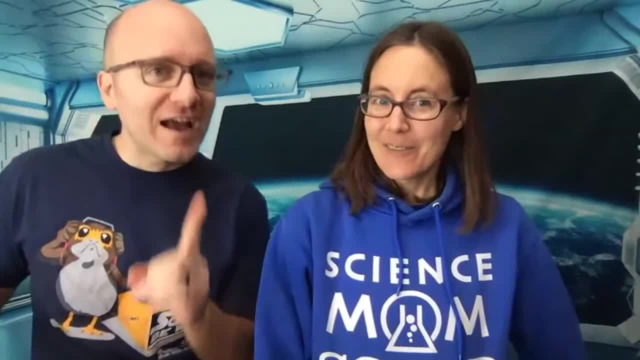 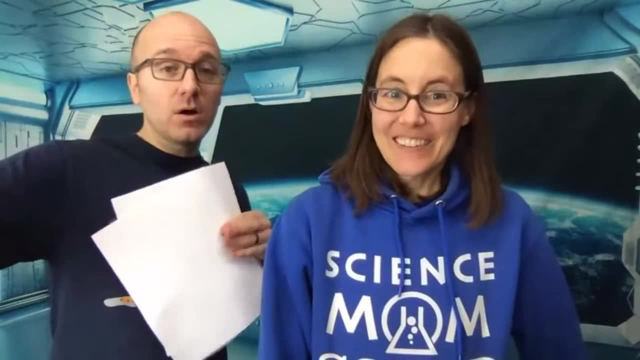 the speed of light is a constant. Now, the speed of light in a vacuum is a constant. I like that clarification, Yeah, So yeah, when this, when light is not traveling through any medium at all, then it always goes at a constant speed. 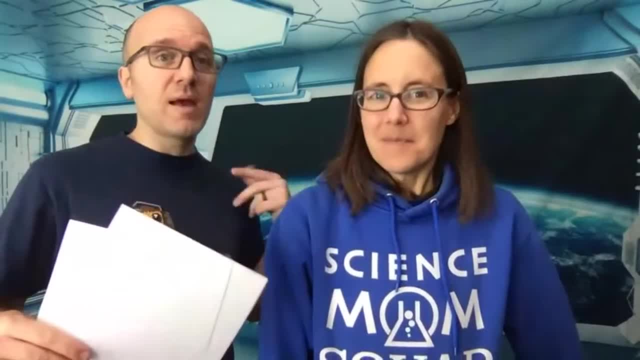 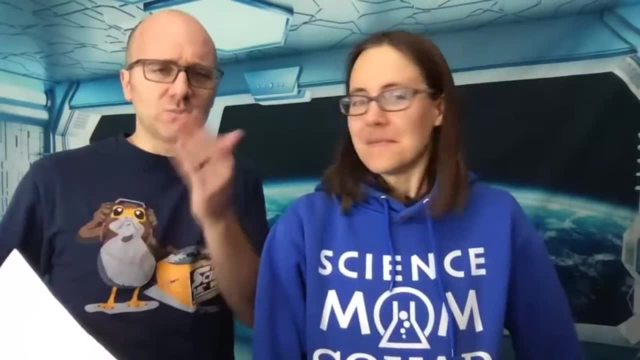 but just like any wave, as it passes through a medium, it actually does change speed. Now, of course, to us, we can't. we can't see the difference between the speed of light and three-quarters of the speed of light. I mean, that's just way too fast for us to comprehend. 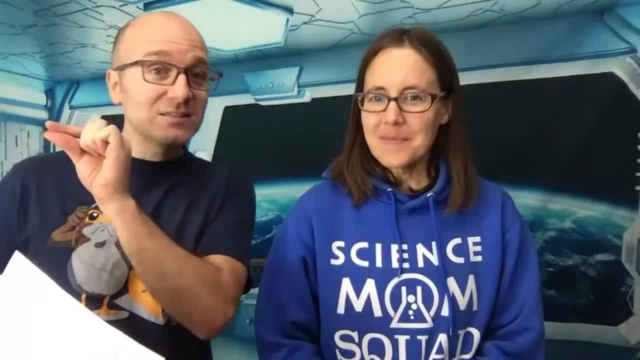 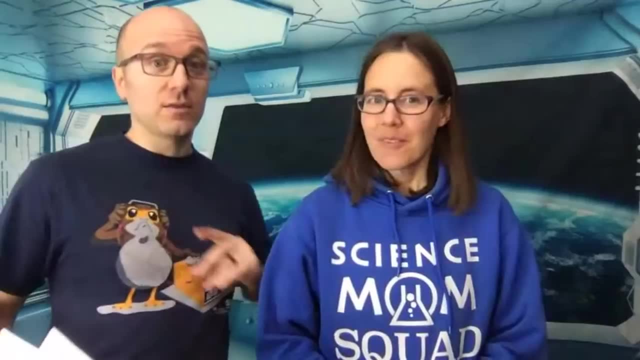 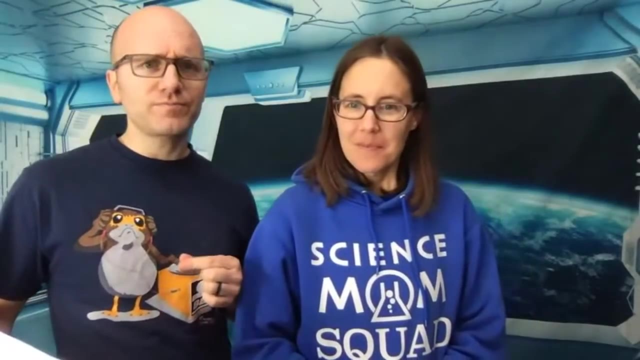 but indeed, as light passes through water, it does slow down and loses about a quarter. but water's not the substance that slows it down the most. There there are others. I mean through a diamond, it would go even slower. and boy they use these super cooled semiconductors. 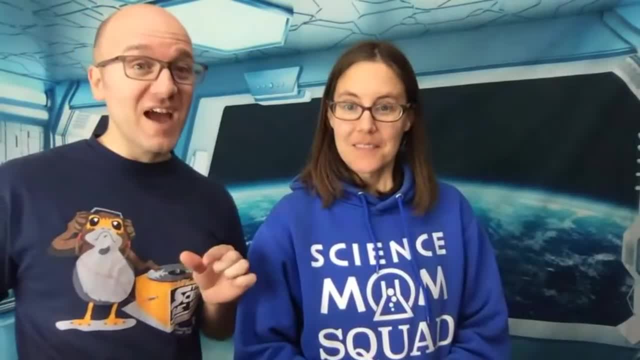 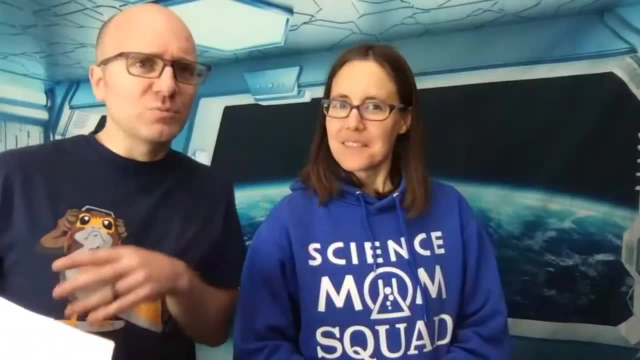 And it turns out they've been able to slow it way down And in fact, uh- this boggles my mind And apparently it's true, Uh, cause I was reading it as from multiple sources- and but they were able to actually bring it to a stop and then restart it. What Yeah? 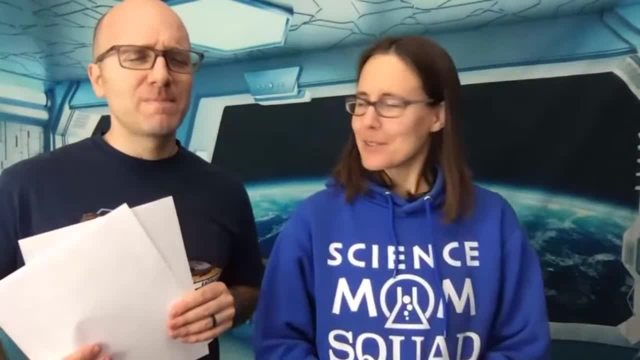 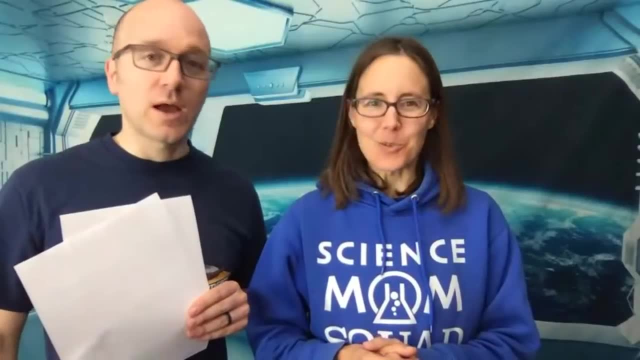 Yeah, My mind was boggled because it what did they use to bring it to a stop? What were they shining light through? Uh, uh, it was some semiconductor that was super, super cooled. I think semiconductor, that's super awesome. Yeah, My mind was pretty blown, but you can actually 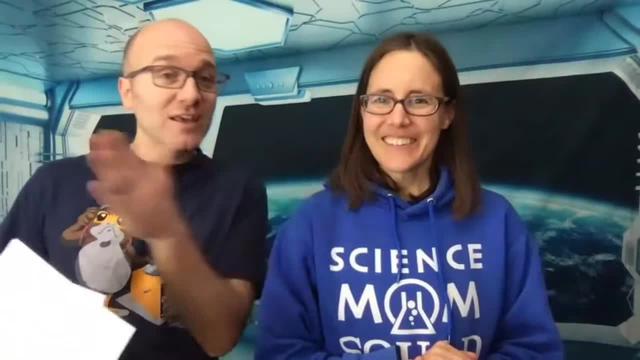 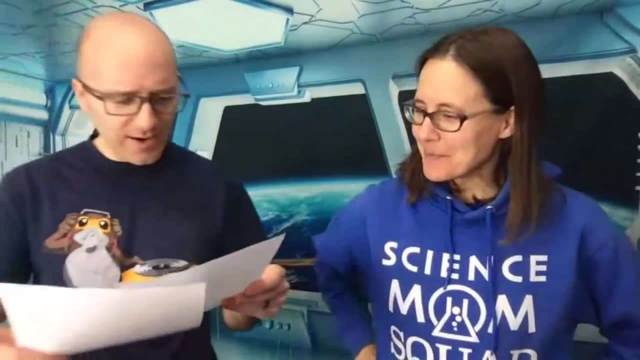 slow the light down until it's traveling at a speed that we can at least recognize. So kind of crazy that that's even doable. All right, Next one. All right Up next. Okay, True or false? Part of Albert Einstein. 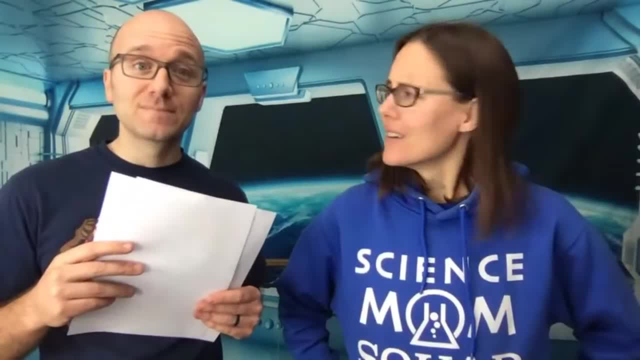 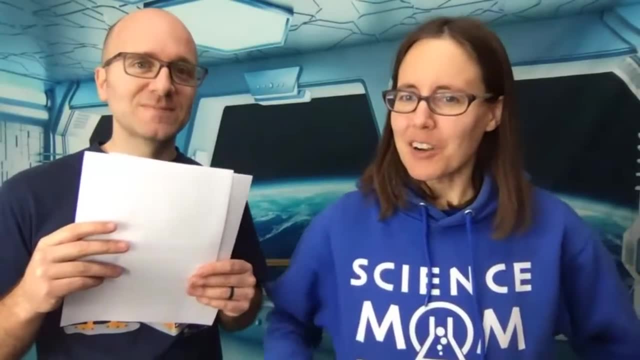 Einstein's brain was stolen after his death. Part of Einstein, Albert's Albert Einstein. Albert Einstein's brain was stolen after his death, True or false? That is the most bizarre factor fiction I have ever heard. Um, okay, Yeah, Deep. 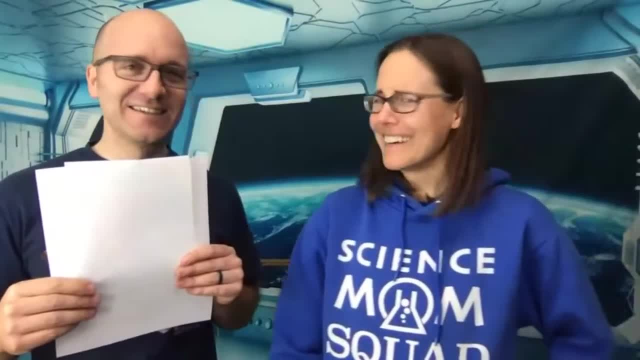 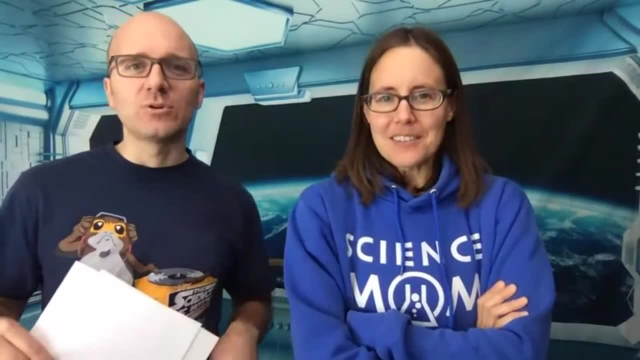 is like what I? that's me too. I'm like what? Cause I? obviously Einstein was pretty smart and yeah, Okay, So I can understand his brain would be. I can understand like researchers, Cause some people will donate their body to science. 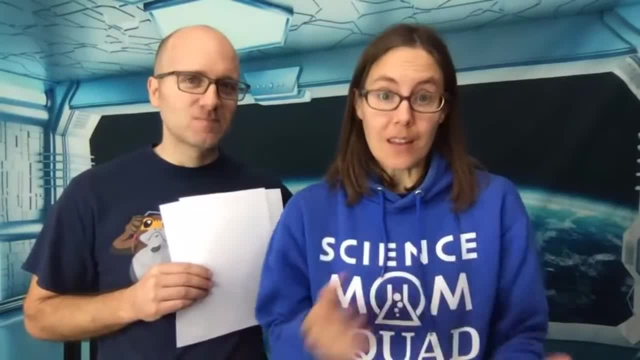 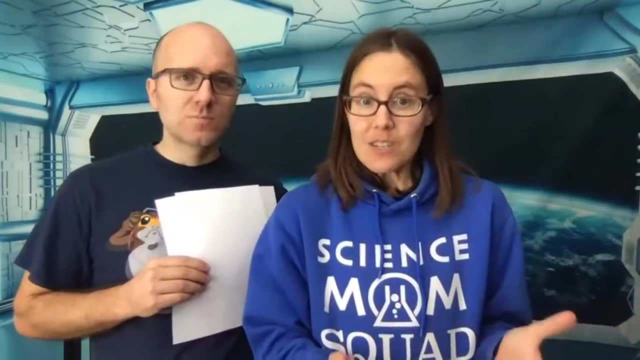 And you know for like for doctors and people to study on, because if you're going to be cutting into a real body when someone's alive, you want to have practice beforehand. So cadavers are used for research and that's a really important part of research. So I can understand like wanting to. 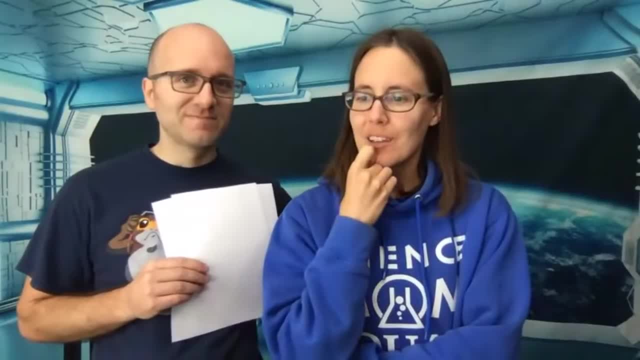 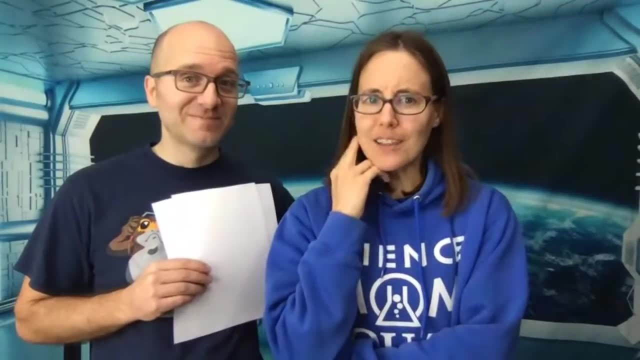 look at Einstein's brain and see if they're like extra neural connections or something. But then if he didn't give permission, I guess technically you could say that his brain was stolen. for that I'm going to say false. I think Albert Einstein would have donated his brain to science. I don't. 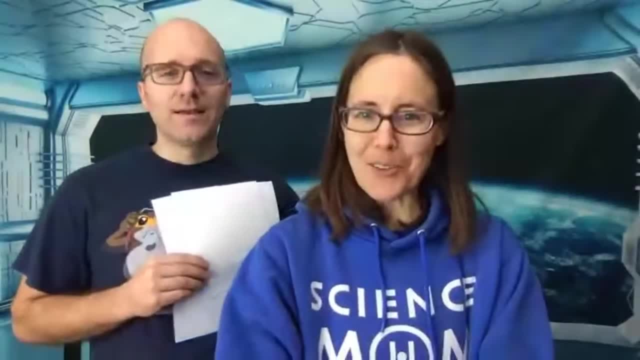 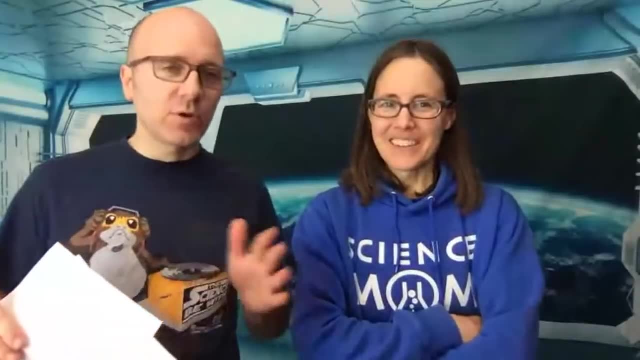 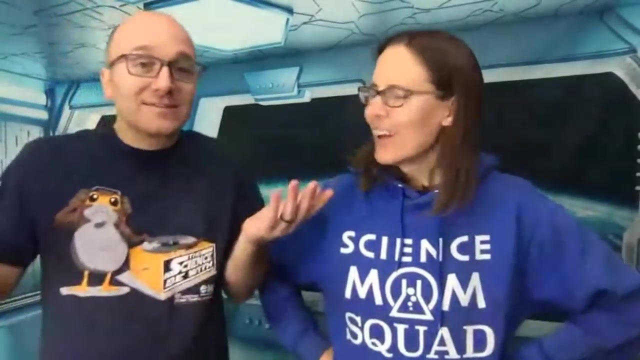 know That's actually true. Oh man, Now I'm seeing all the truths and Cassandra and puppy love Hogan, Everyone's saying true, Yes, So he, he didn't want it, He wanted to be cremated and his doctor took the brain and his eyeballs and yeah, All right. So I'm just going to go right out there and say: 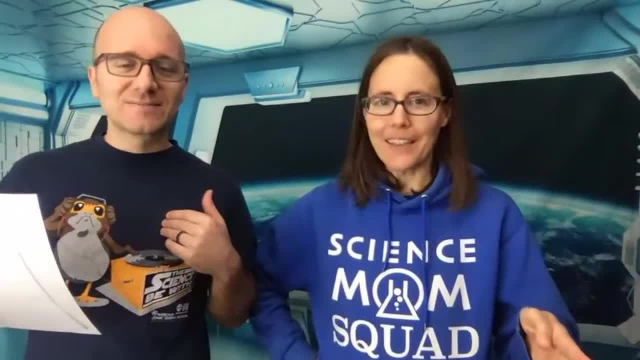 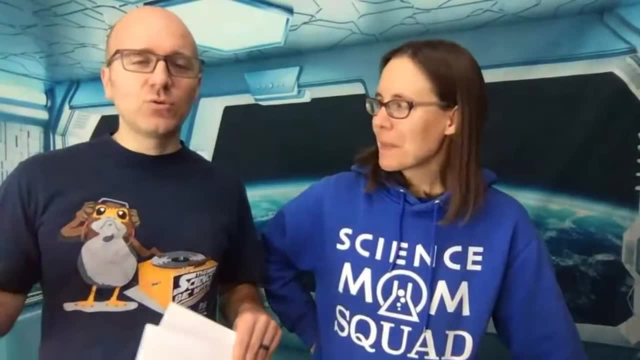 that if someone says like this is how I want my body to be treated after I die, like everyone else should respect whatever they say. I agree, Yeah, Shame on the doctor. And unfortunately it didn't do do much good. I mean, it seemed to have some extra folds in places, a few anomalies. 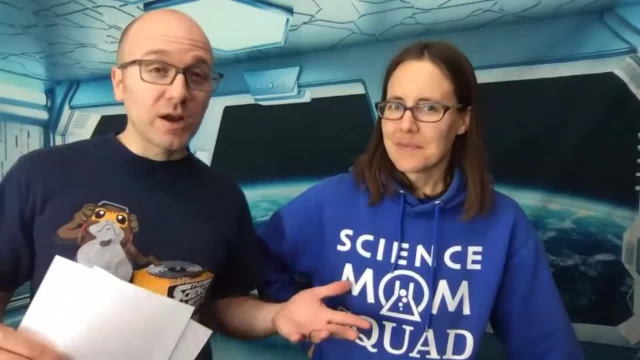 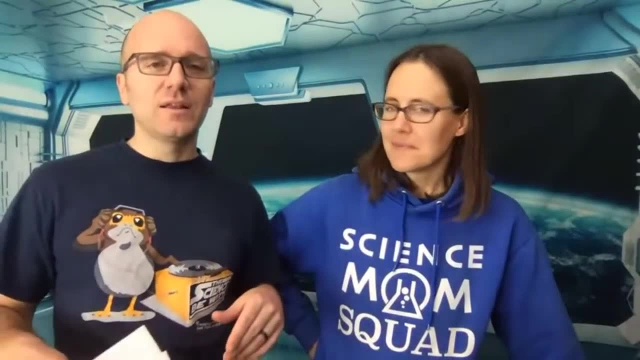 but for the most part ended up being a pretty normal brain, and they didn't really even have the techniques back then to do the type of studies. They couldn't take care of it. They didn't have the DNA know-how that we have, So they didn't actually learn much from it anyway. So 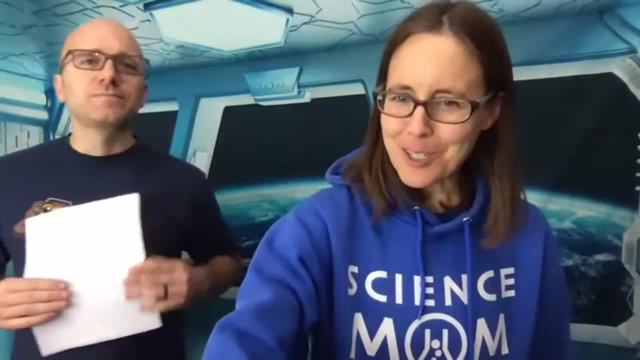 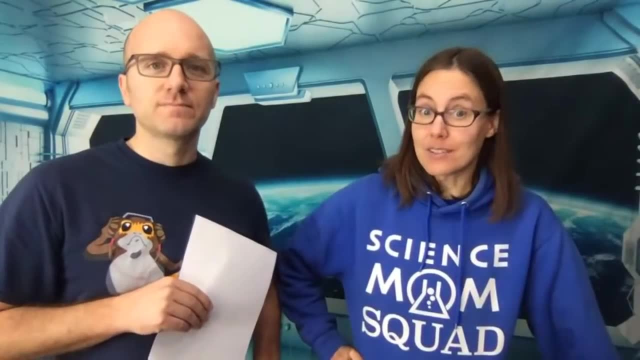 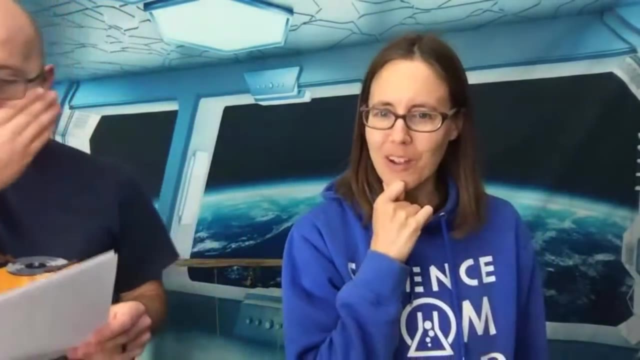 all right. Well, that that factor fiction- makes me feel kind of grumpy, All right. Sure, False pulleys and levers Are the only types of simple machines. false, There are more types of simple machines than pulleys and levers, Although at the moment I'm having a hard time thinking about what other 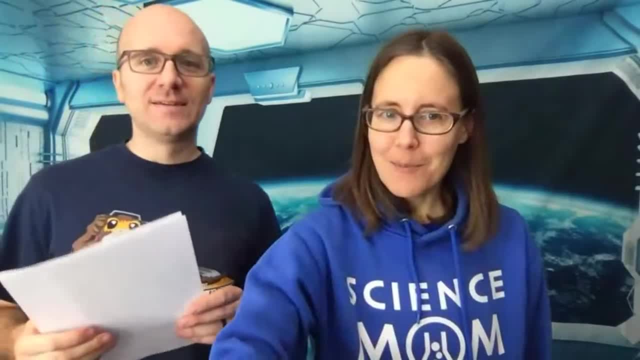 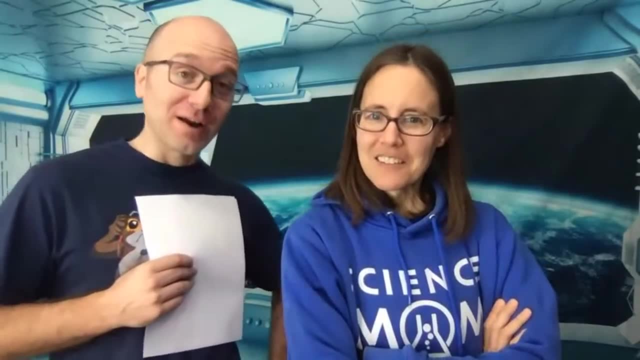 examples there might be. Help me out in the chat. What other type of simple machines are there? That's a good question. I know there are more. Let's ask the chat here that there are indeed more. So you are correct. All right, I was right, There are more simple machines besides. 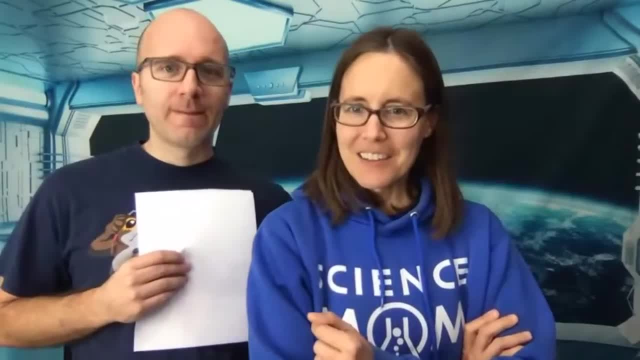 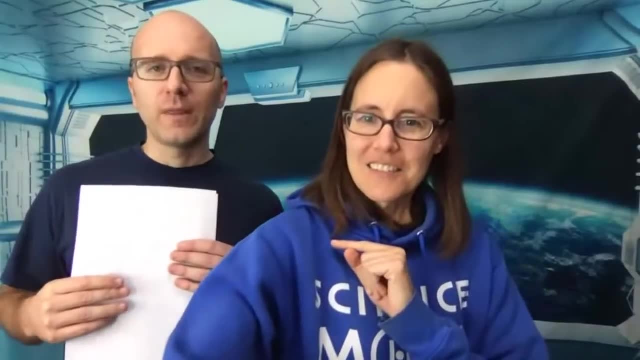 pulleys and levers. What's an example, though I'm drawing a blank. I'm drawing a blank- things that give us Mechanical advantage is what we're we're looking for, And I should say I mean, this is kind of 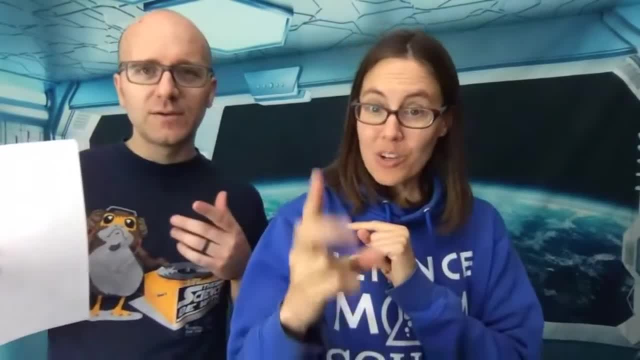 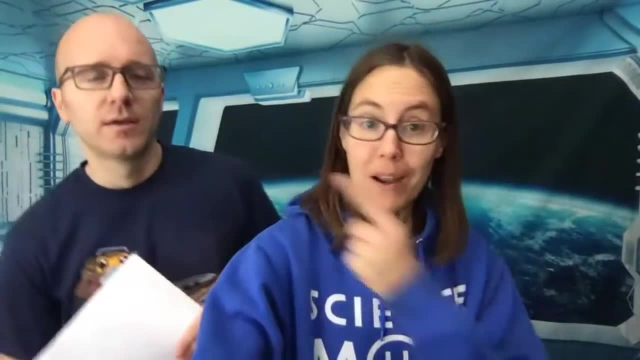 this Renaissance idea, these things that got studied. So a catapult and a wheelbarrow, Those are two great examples. Those are both. I mean, you can think of them as levers, right, Yeah, Levers are being used there. Yep, Oh, a ramp, Okay A ramp. So an inclined plane is what they. 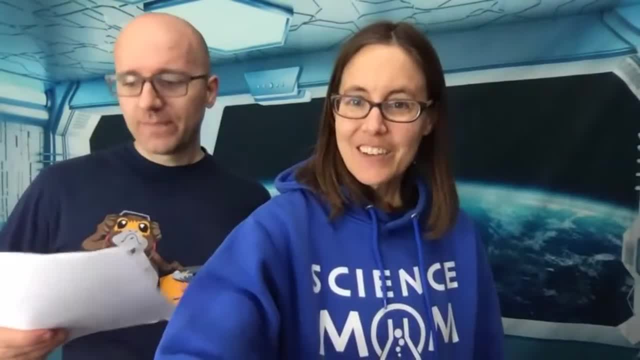 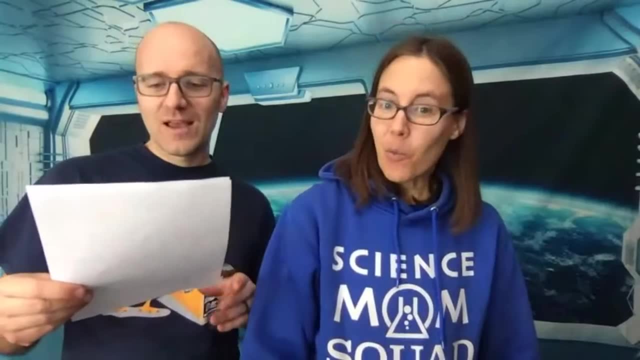 the Renaissance scientists called that Good A screw. Thank you, Brenda. A screw, Very nice. A wheel, A wheel. Okay, Yeah, The wheel should have thought of a wedge, which is like an inclined plane And the way that that's. those are the six types the Renaissance scientists identified. 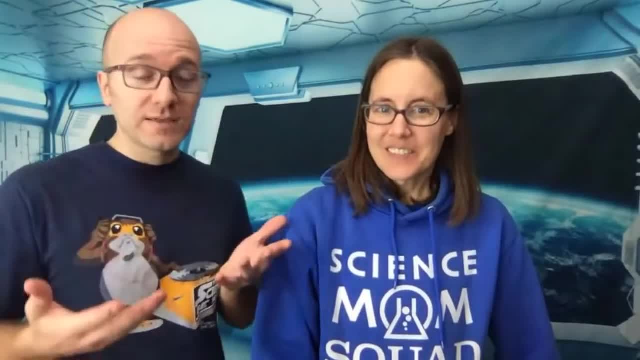 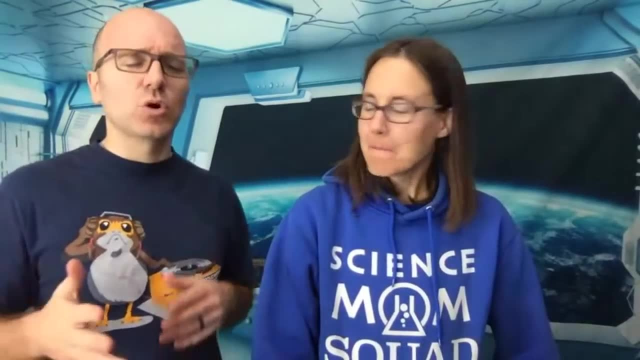 And it's not that there aren't other things. I I think you could classify up to a hundred different things as simple machines And it turns out it's a little more more complicated than that And you start combining these simple machines and you get a complex machine and you got. 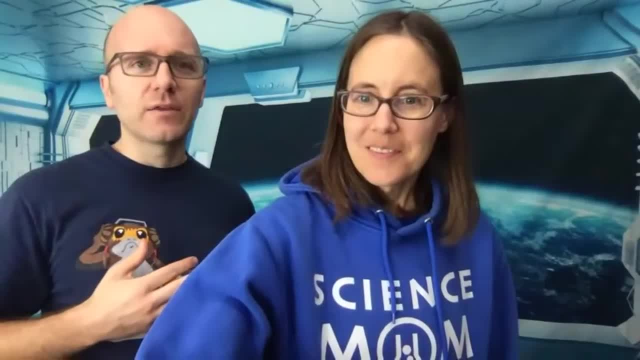 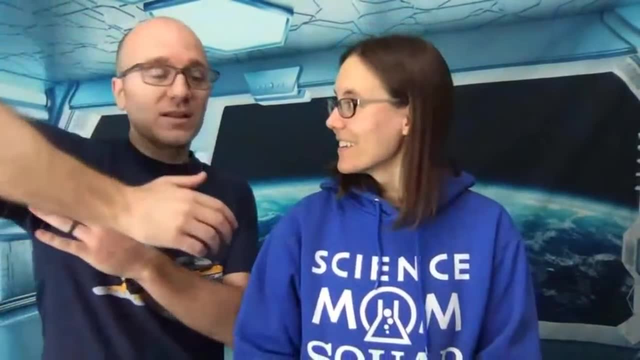 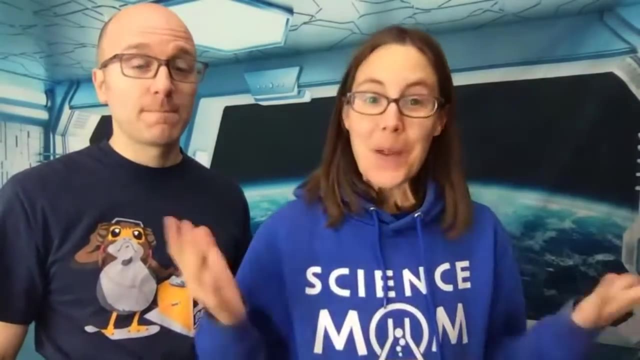 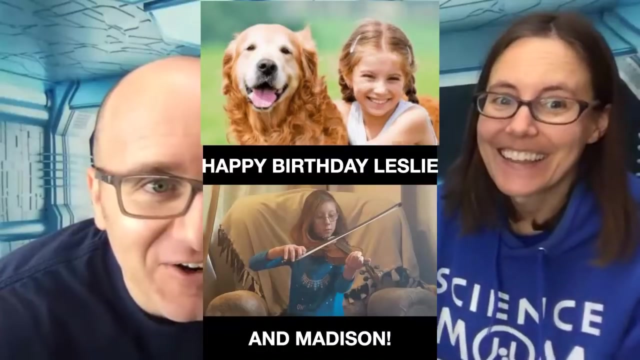 pulleys and levers Combined together and you're able to build things like an automobile and certainly our body. We've got compound levers in there with the ways our arms or joints move. So guess what, Matt? We have birthdays today. Oh, whose birthday is it today? So happy birthday to Leslie and Madison And I. 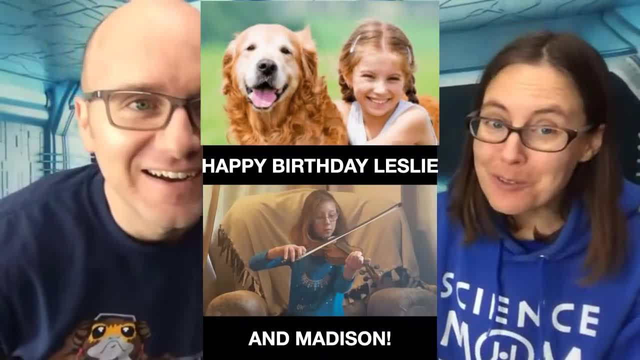 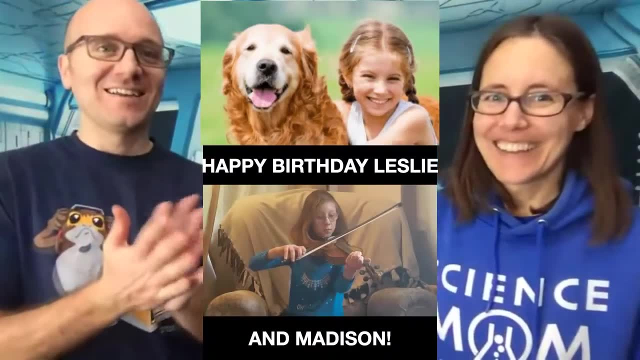 have to say, I love these pictures here. So, Leslie, with a beautiful, beautiful dog and Madison playing the violin, You can play the violin too. That's right, I play the violin and I, yeah, have for many, many years. I don't pull it out as often. 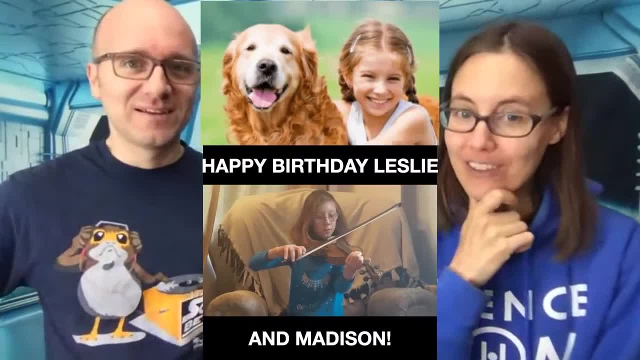 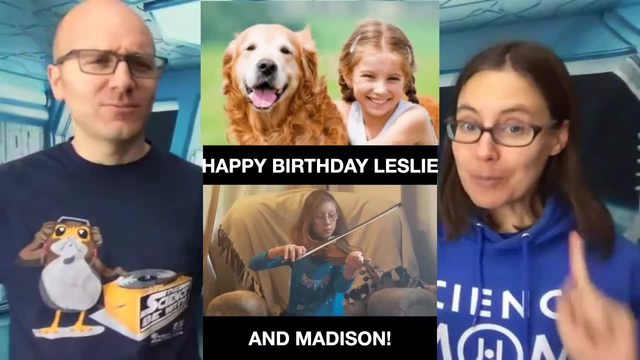 now, as I perhaps should Now for a birthday song. don't start yet. I know that you're just going to like, be like. oh, I'll sing the song that I sing every single time, But I know that more people are getting tired of hearing. 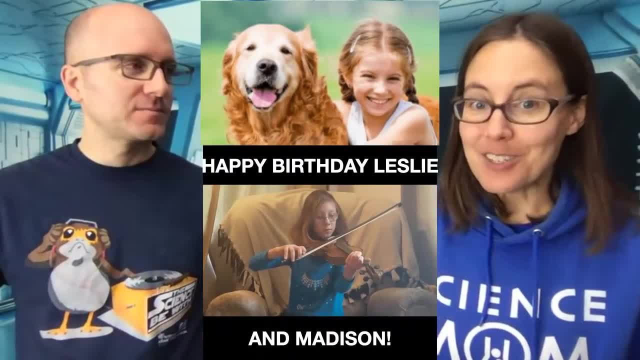 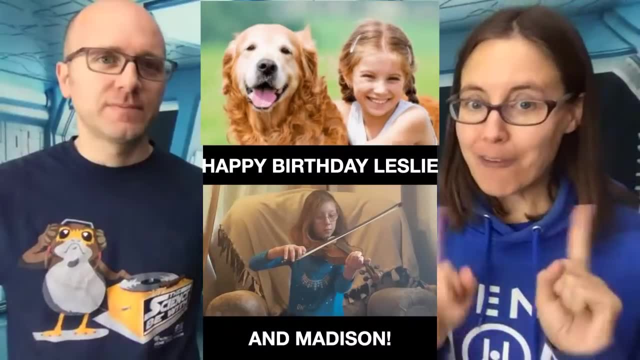 the same song over and over again. So I think it would be fun if in the chat you told dad to either sing it like a chipmunk in a really high, squeaky voice, or sing it super fast. So put F for fast. 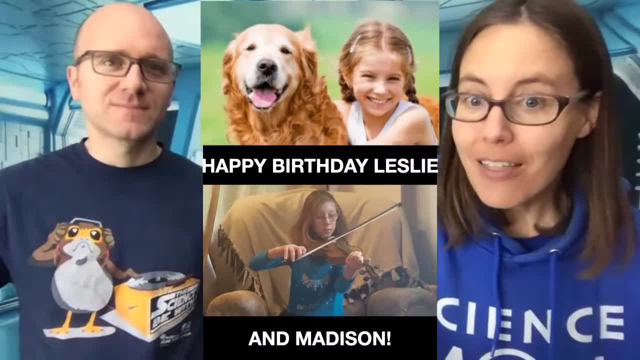 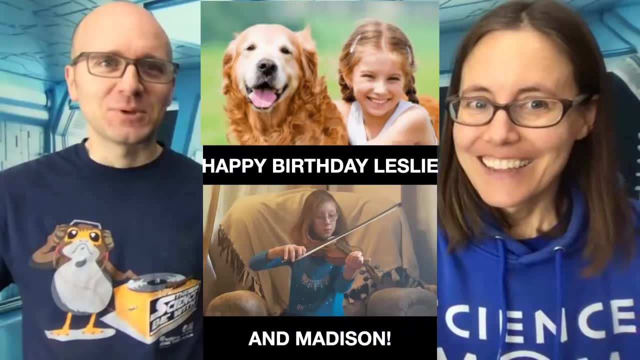 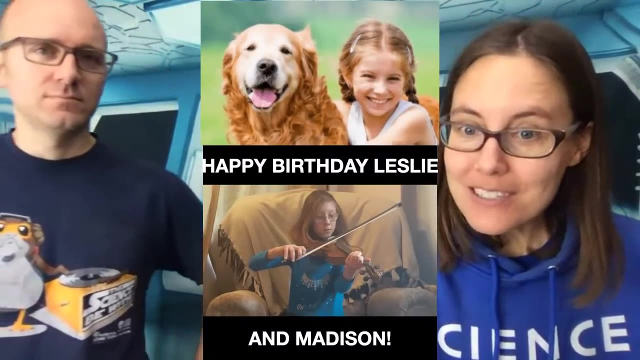 Or C for chipmunk in the chat And whichever one we see the more of. that's how he will sing the song as a happy birthday for Leslie and Madison. What makes you think I can sing it as a chipmunk? Good luck, Beth. dad, I'm seeing a C from Owen. I'm seeing an F. Oh, I'm seeing more Cs. 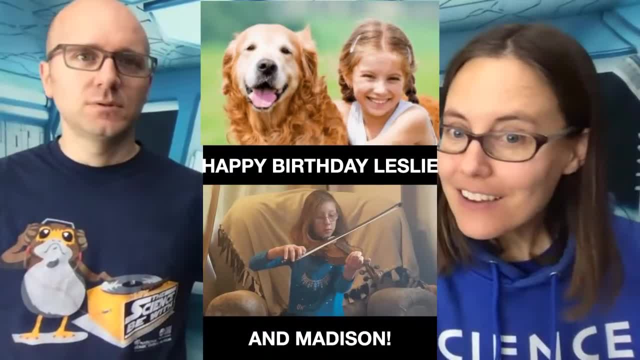 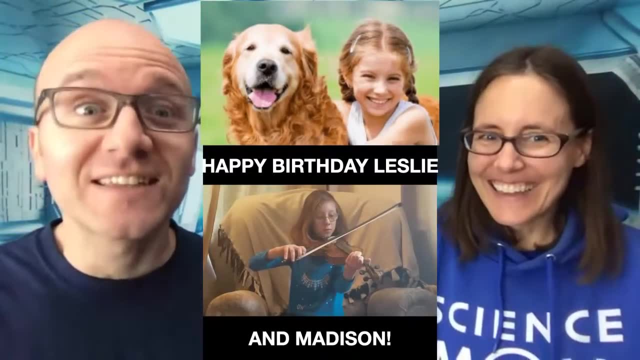 Alyssa and Owen and David and Alice and Tammy. All right, Fast chipmunk. Raina says: fast chipmunk. There you go, Fast chipmunk. All right, I'm singing out a song. I don't know the words. I don't know the words to the song. 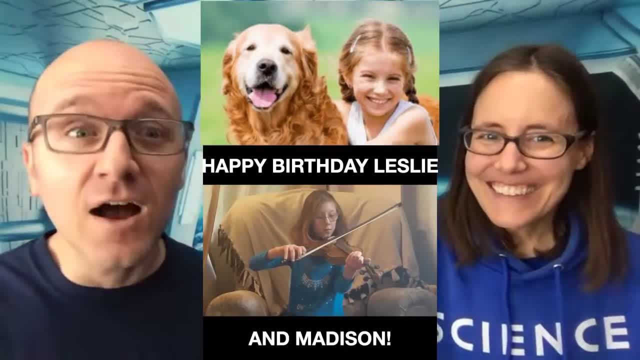 I'm singing. I'm singing as long, but I don't know the words to the song. No, I don't know the words to the song. Awesome, Good job, Beth, dad, And a happy birthday to Leslie and Madison. 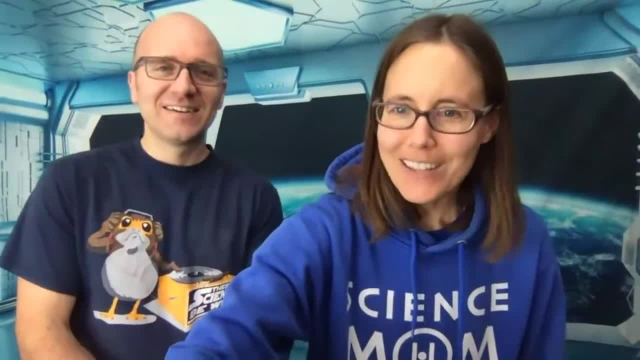 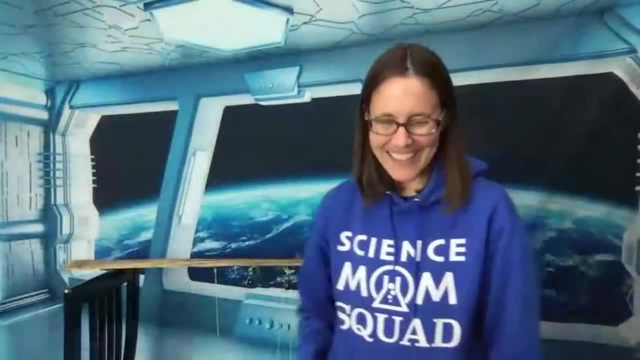 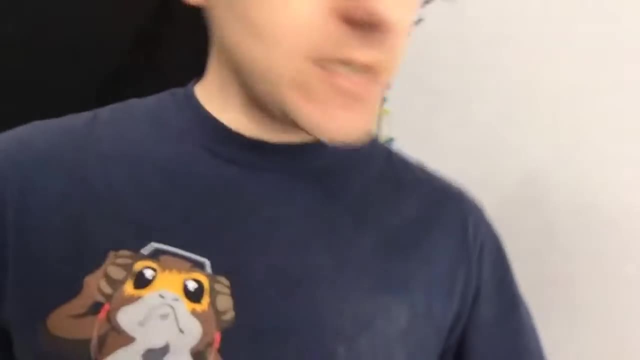 Indeed, Anyone who is joining our show for the first time is probably like what in the world just happened? Yeah, that's where they turned it off right there. Now it's time for math. All right, Turn this guy around And we are going to talk about circles, but I wanted to. 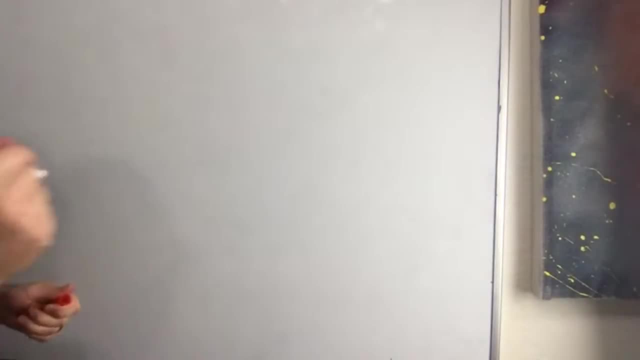 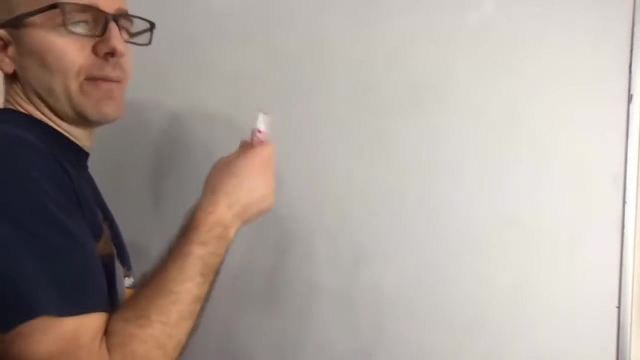 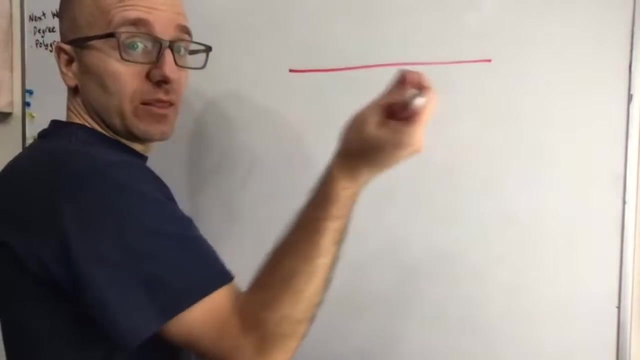 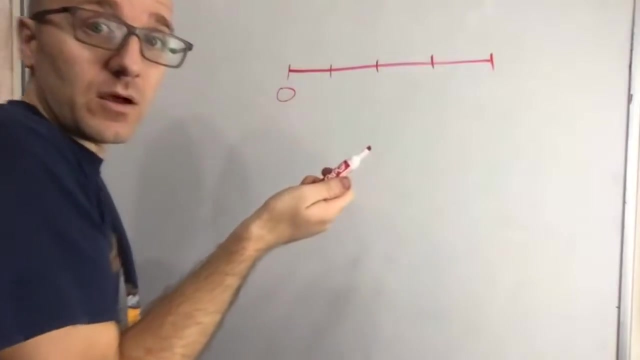 first of all, talk about levers a little bit more and this idea of mechanical advantage And in fact, if you think back and happen to have seen the video we watched about how to find the average of some numbers, let's say along the number line, So yeah, suppose I've got zero, one, two, three, four here along my number line. 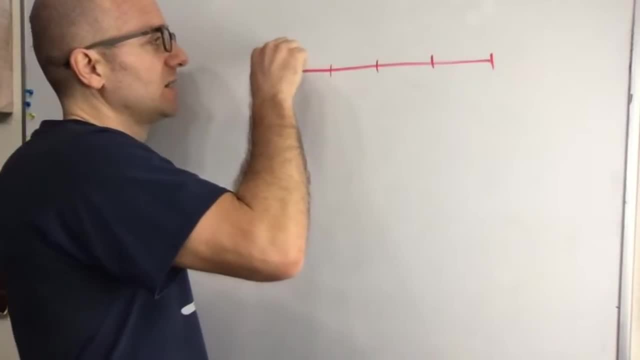 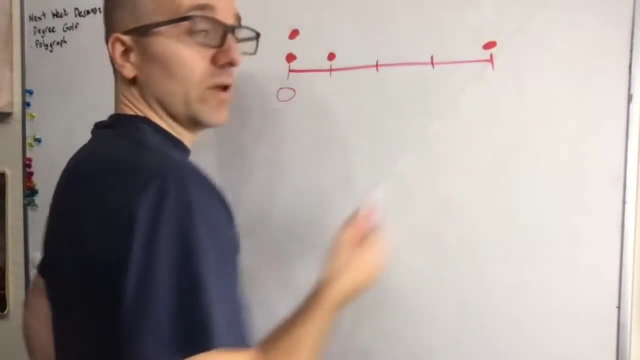 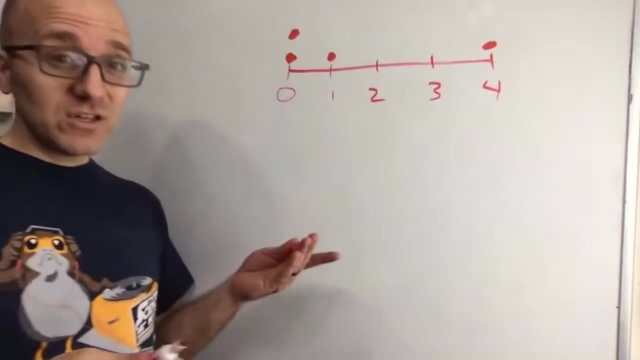 What? what we were able to do is we said, OK, suppose I stack Two things here, one thing here and one thing over at four. One, two, three, four. How could we find the average of those numbers? Well, I count one, two, three, four numbers. 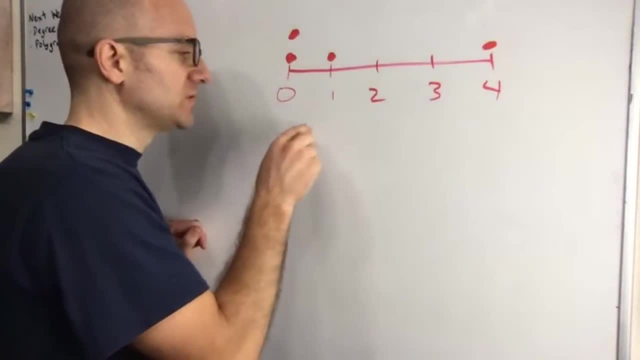 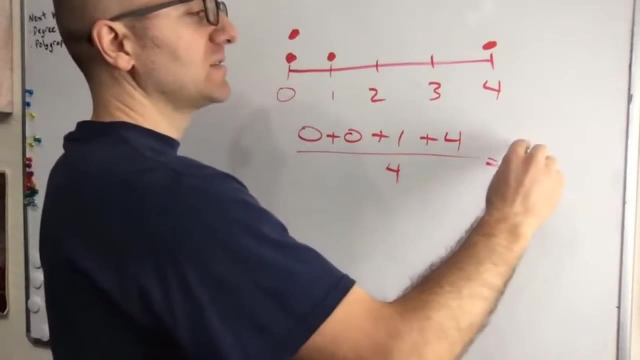 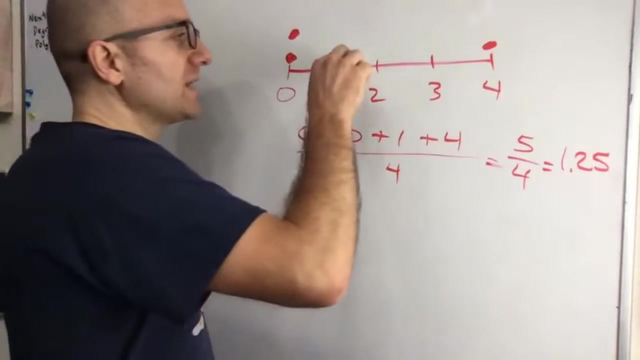 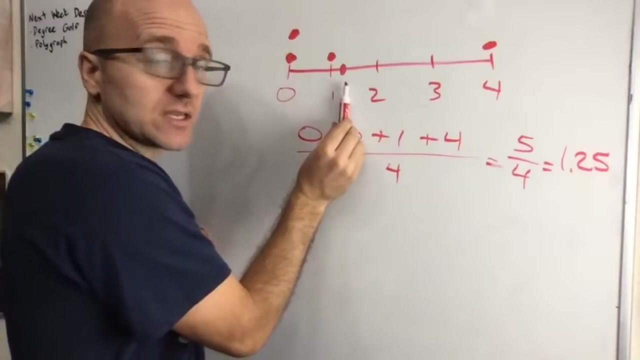 And if I take their average, so we would just do zero plus zero plus one plus four, all divided by four, And it works out to be four, Five over four, or one and a quarter to one point two, five. What that told us was that right here, at one point two, five on the number line, that was the balance point. 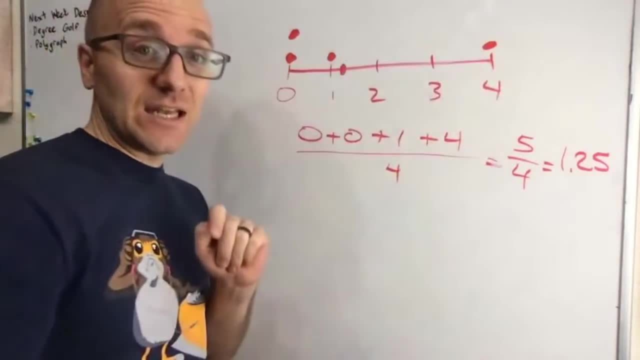 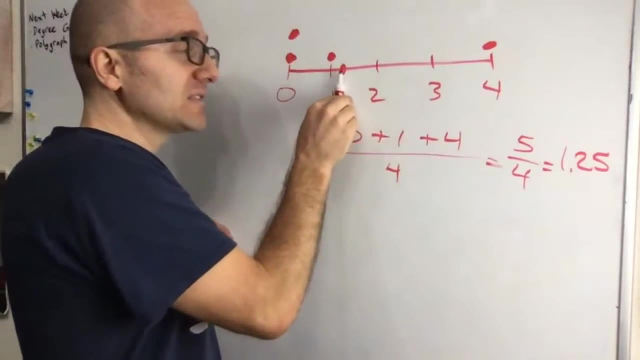 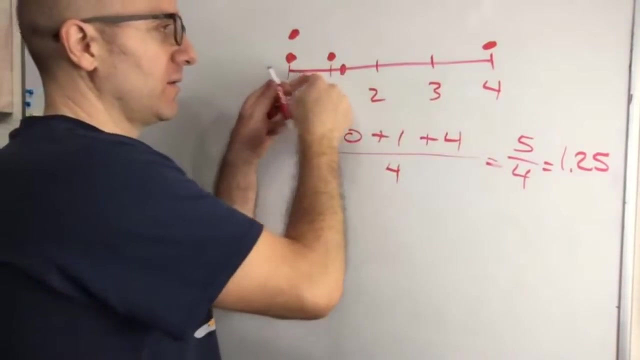 So if this number line that I had drawn was a teeter totter- and we're assuming that the line itself has no weight- then the balance point is exactly the average. So if we, If, If science mom had had this at the beginning, we could have actually calculated where we would need to set the objects. 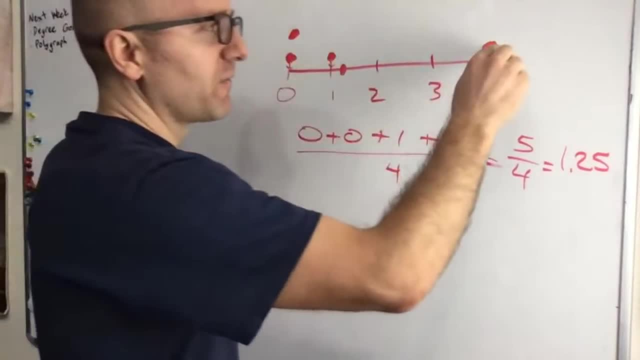 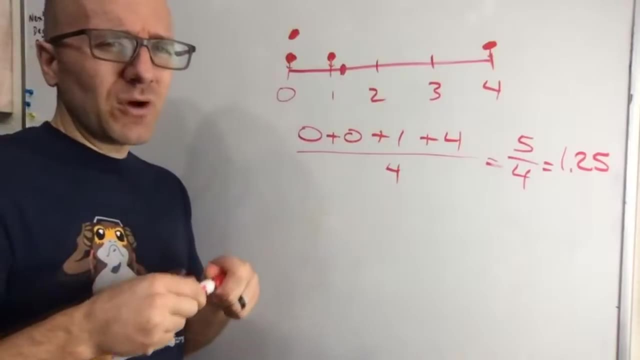 And that's assuming that all their force is exerted as one single point. I mean, it's easy to you kind of have to oversimplify those, And we're always the problem with mathematicians. And when we do physics we're always assuming there's no friction. 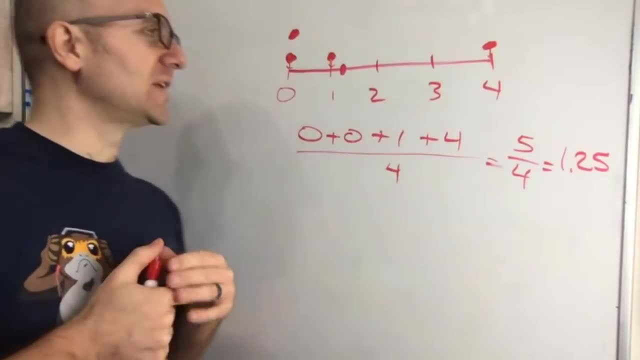 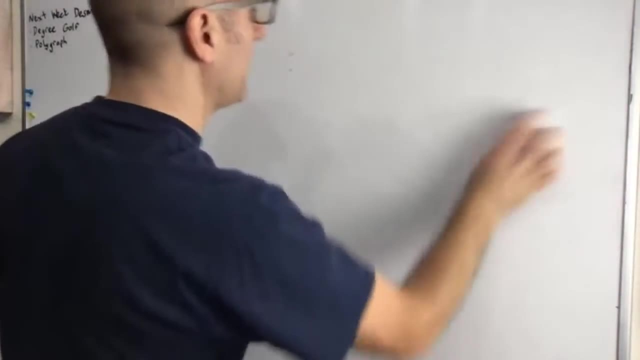 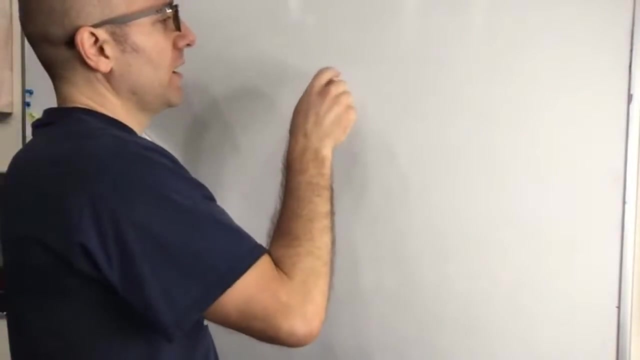 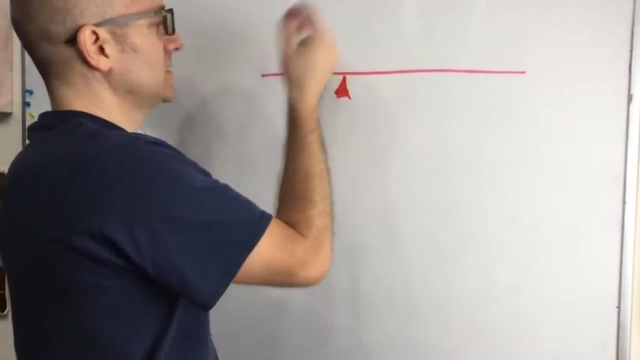 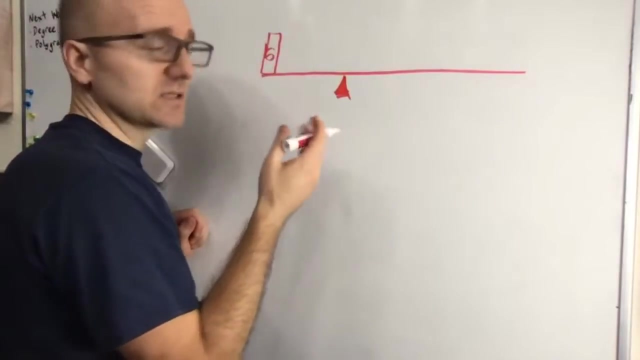 And in the real world, yeah, there's usually some friction, There's no way of getting around, But this is a fact, that the work is equal to force, times, distance. So if I had my, my fulcrum here and my board, and if I put some object here that weighs I don't know, six whatever's, six pounds, six kilograms. 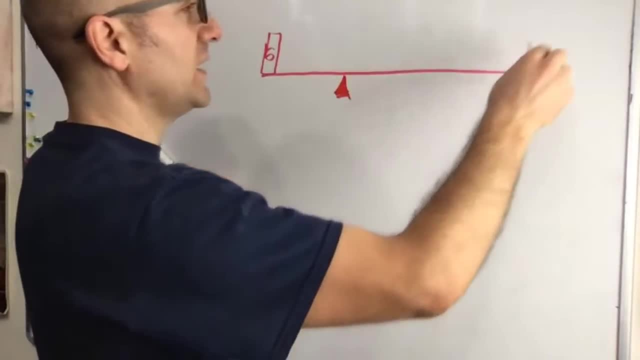 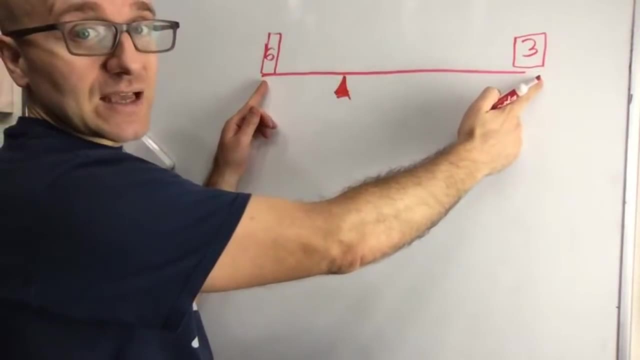 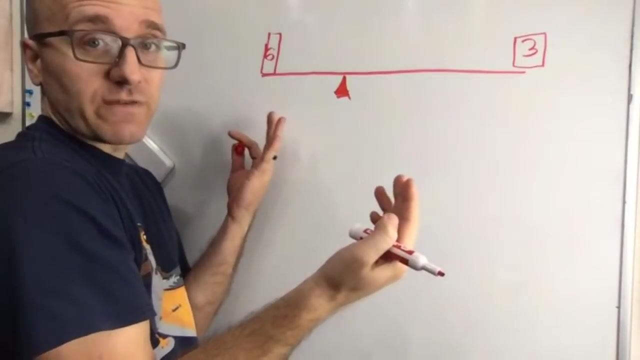 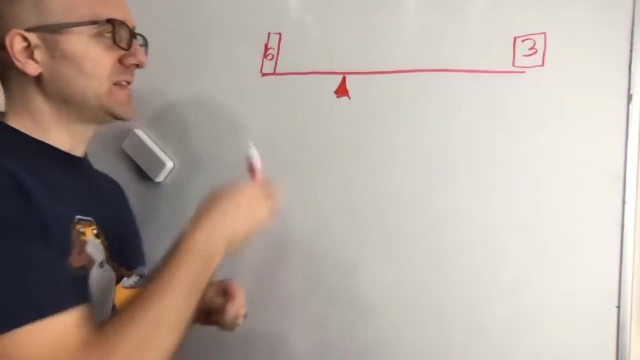 All right. Then I have another object that weighs three kilograms Or three whatever's. Then if I want it to balance, I literally have to double the distance to the fulcrum and then things will balance just fine. So on a teeter totter: sometimes I would try to get a teeter totter with my kids and I actually have to sit pretty far up the board, maybe, maybe near the middle. 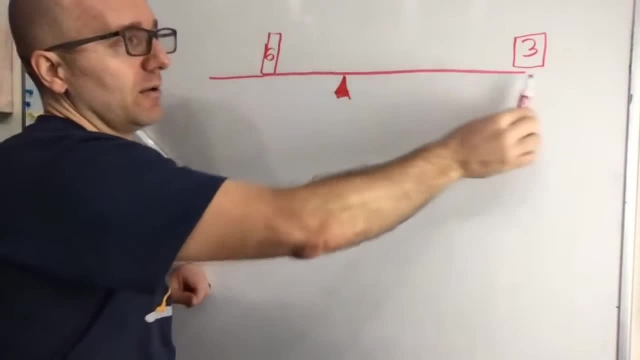 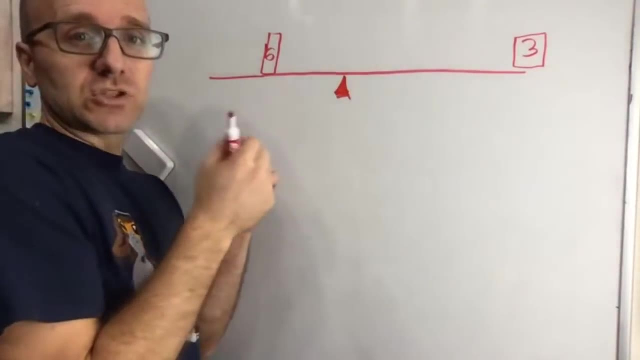 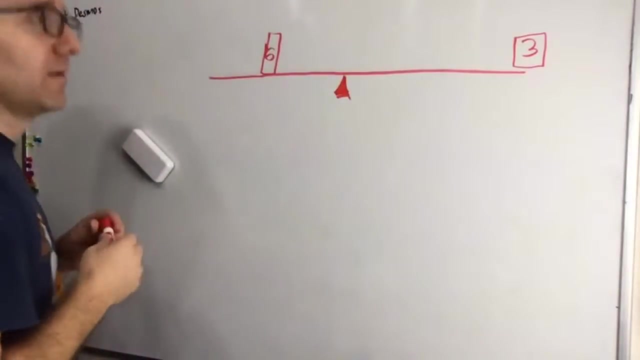 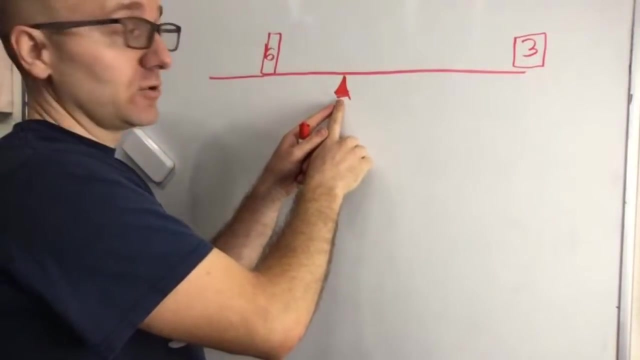 But then it worked just fine. We were able to to teeter totter, even though I'm way heavier than my kids. So I'm just trying to point out: you can mathematically compute these distances and It was long, long. you know these masses or, for that matter, you could compute the masses just by identifying the distance that it took to get the fulcrum to come to a level. 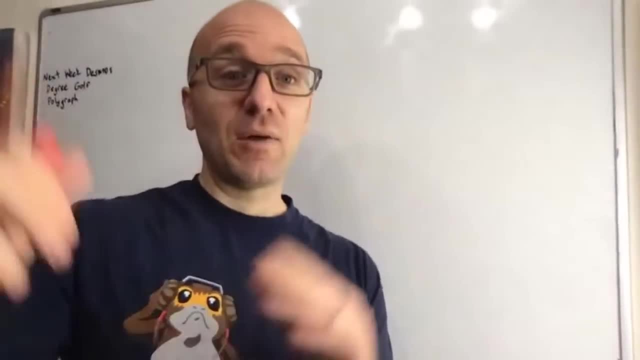 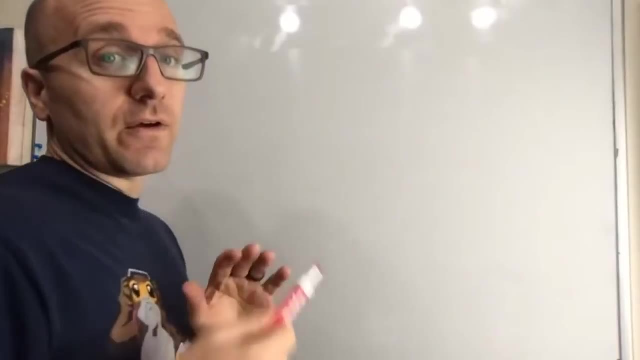 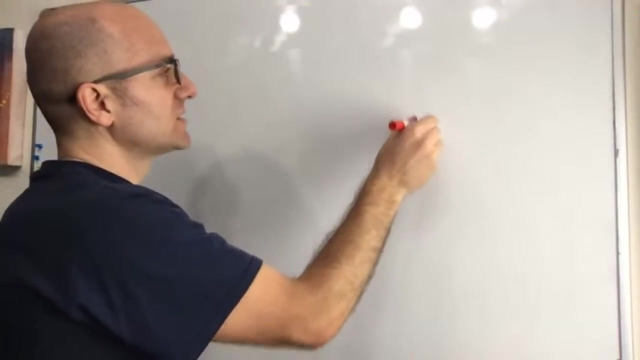 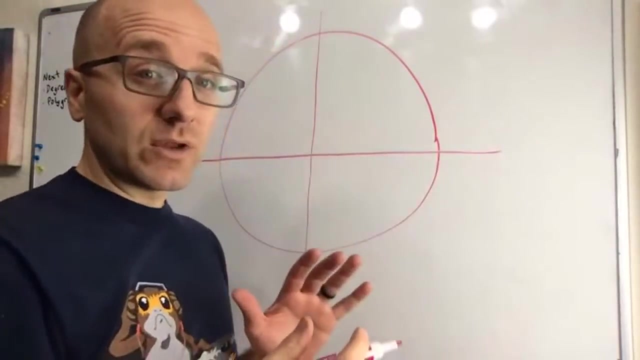 All right. So I want to talk a little bit about circles, And there's lots of things we could talk about. The first thing we're going to talk about is just a review of degrees. So inside of a circle, We had really just talked about angle measures from zero degrees up to 90 degrees. 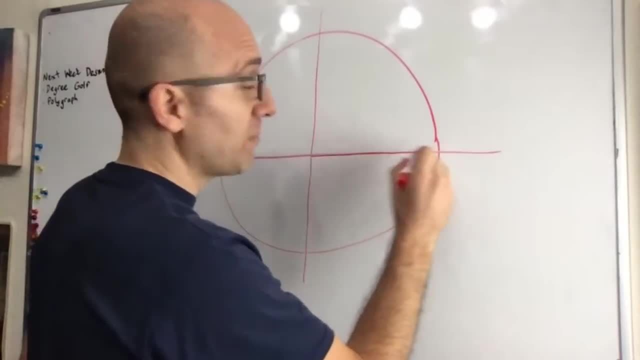 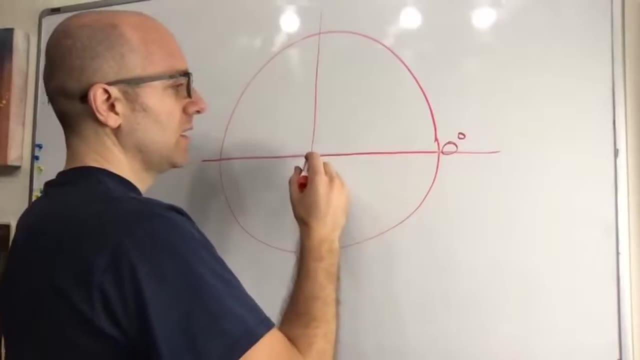 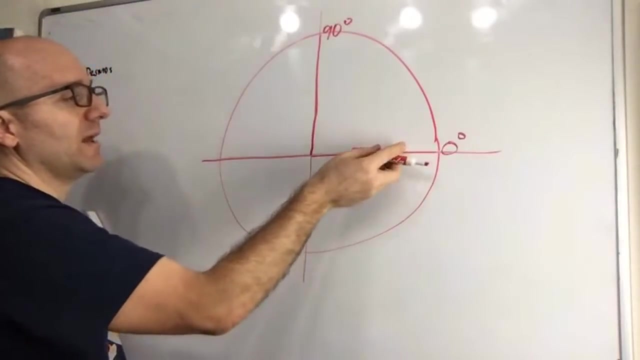 So we typically start along the positive X axis, thinking of this as the origin. So this direction is zero degrees. If we went straight up, we ended up with 90 degrees, And then, if I go another 90 degrees, I'm up to 180 degrees. 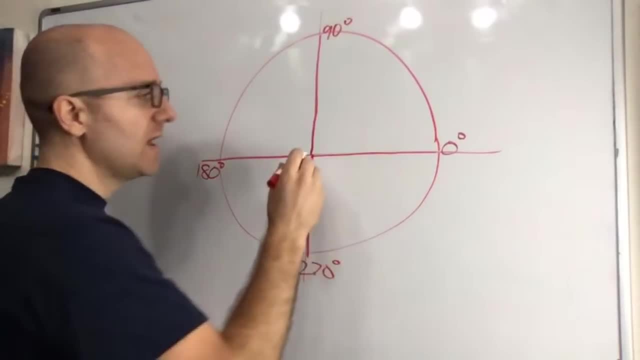 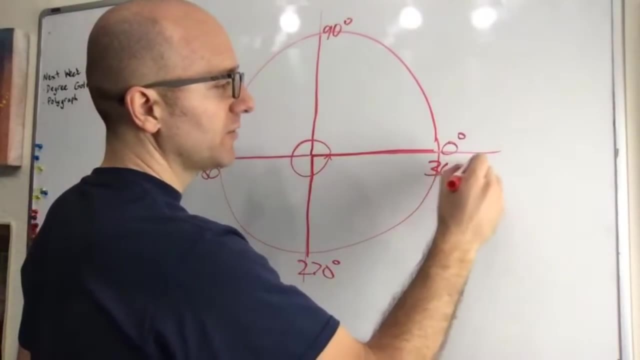 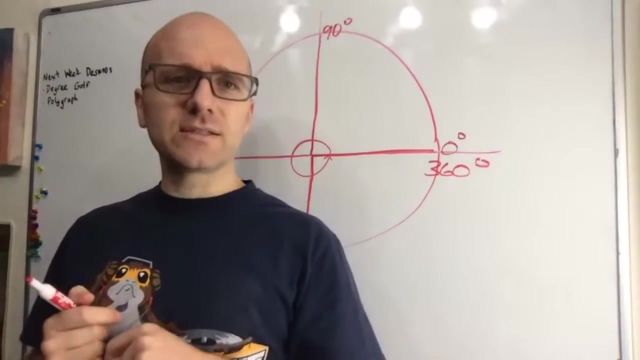 Another 90 degrees gets us to 270 degrees, And then, if we go all the way back around, so full trip around, then we're at three hundred And And 60 degrees. So Here's the question: is zero degrees, a zero degree angle, the same as a 360 degree angle? 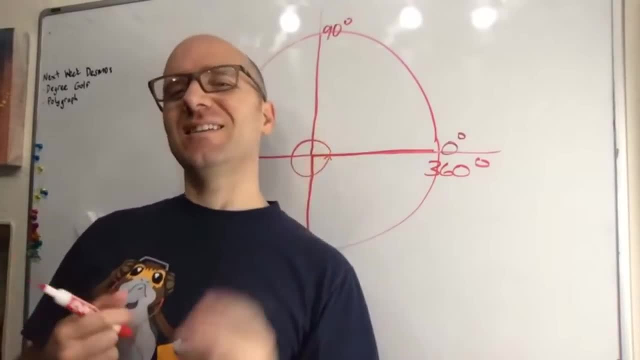 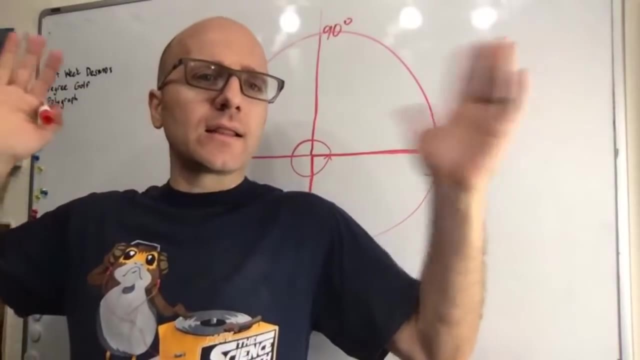 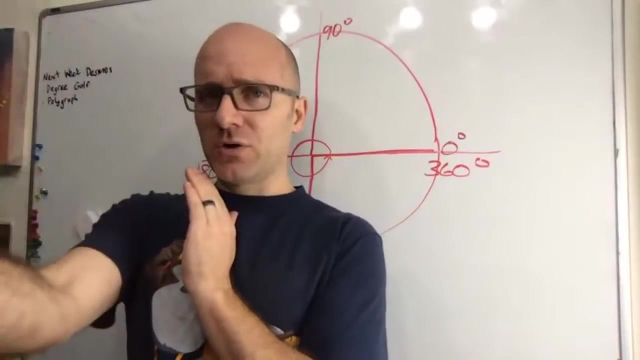 Yep, She says yep, And I would say it's kind of kind of a trick question. It's at the same point on the circle, That's right. So in a in a lot of contexts, it just doesn't matter if I'm, if I just said, all right, if I'm navigating, all right, I need to go zero degrees in this direction or I need to go. 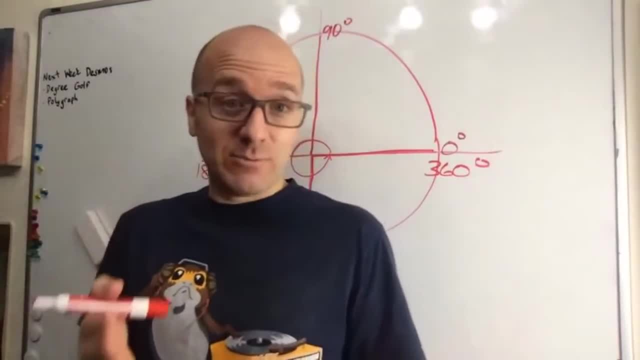 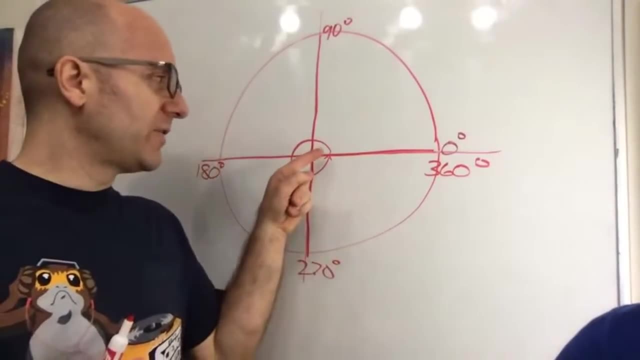 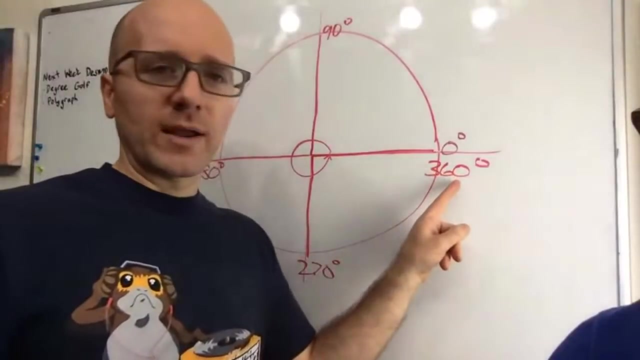 360 degrees in this direction, I'm still going to end up in the exact same spot. It just didn't matter at all. So those two angles are co-terminal, but there are lots of contexts where it mattered that I spun around. if I was carrying a rope and I spin around, I get wrapped up in it, or yes, or I get. I get dizzy as I spin. 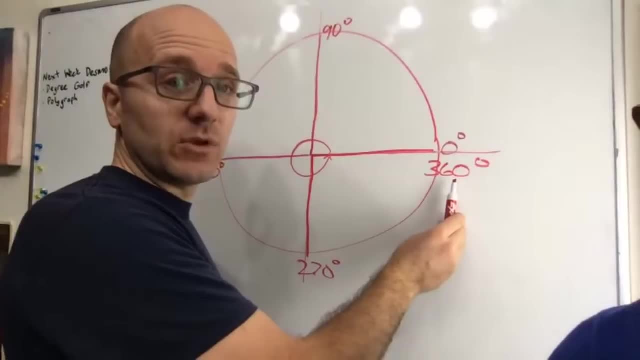 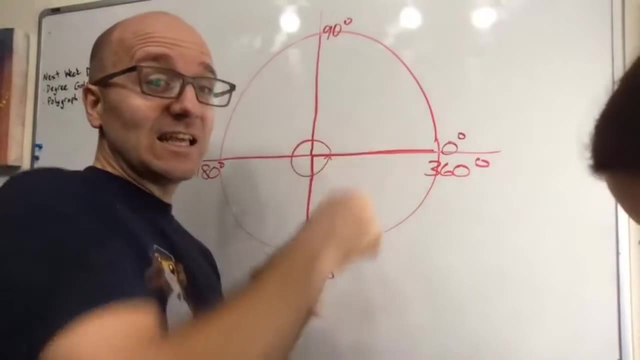 I mean there are some reasons why you wouldn't want to use 360 degrees when you meant don't turn at all. So we call these angles co-terminal because they terminate in the same Point and the same. we could go around a bunch of times. 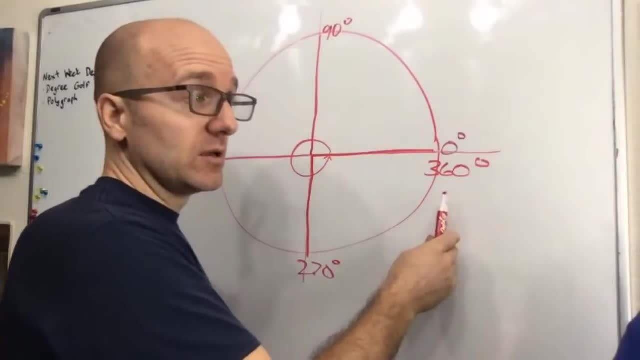 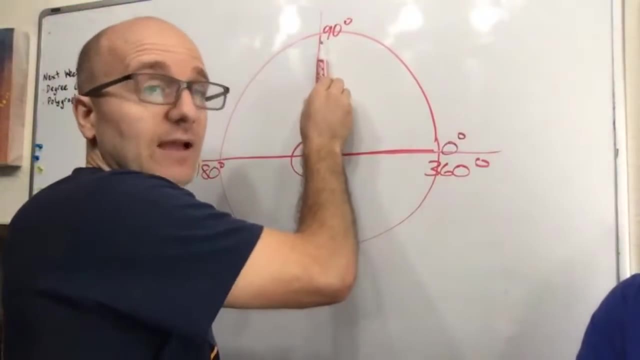 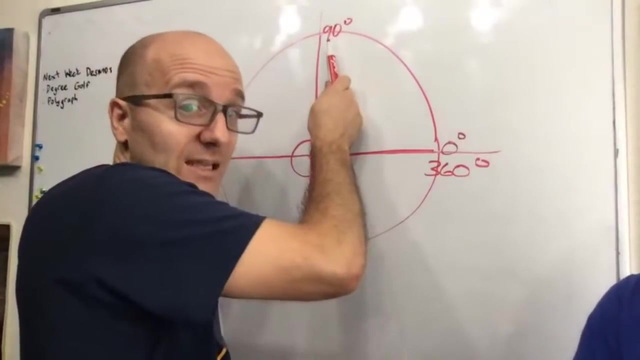 And as long as we end up in the same spot, the angles would be co-terminal. That's the first time I've ever heard that word, Oh really. Oh yeah, That's a good word. And, of course, a 90 degrees. if I added 360 degrees to it, we would get 450 degrees, and that would be co-terminal with a 90 degree angle. 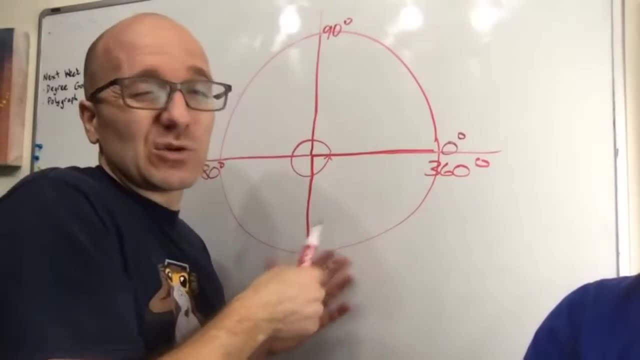 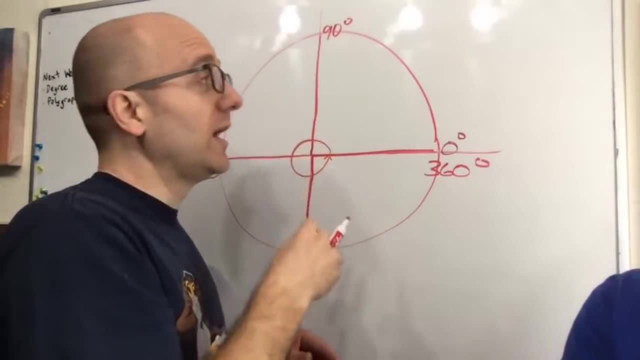 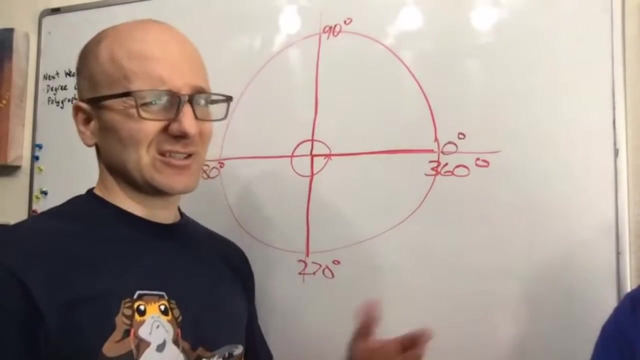 So often we just care about what direction we're pointed, but other times we literally care. Well, how far did we have to rotate? And so the angles are not actually equal angles, but they're co-terminal, And for many applications you just don't care the difference. 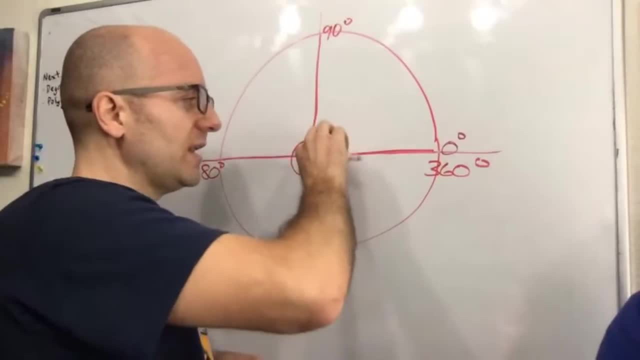 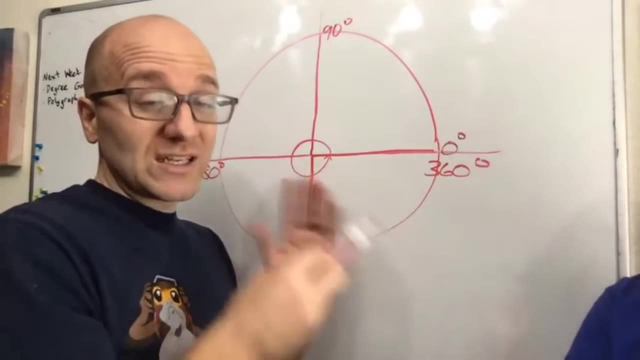 I don't care whether I go positive 180 degrees or negative 180 degrees. Most of the time either one would work. But there are cases where we would want to distinguish between those And in that case it wouldn't make much sense. 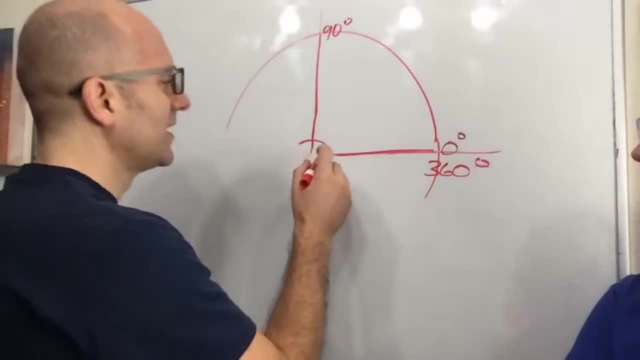 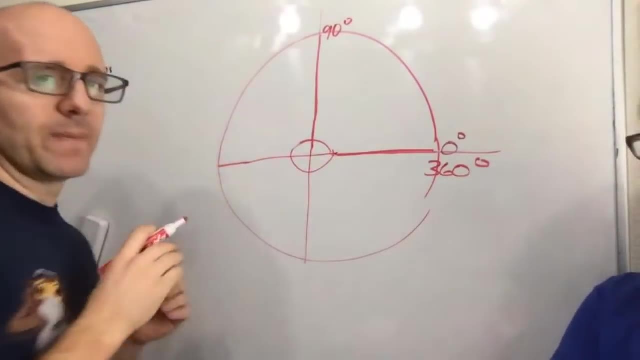 OK, so what are the other things? Oh, sorry, Sorry, I didn't mean to erase that yet Real quick. So what if I were to ask Science Mom for where is a 200 degree angle? Where is a 200 degree angle? 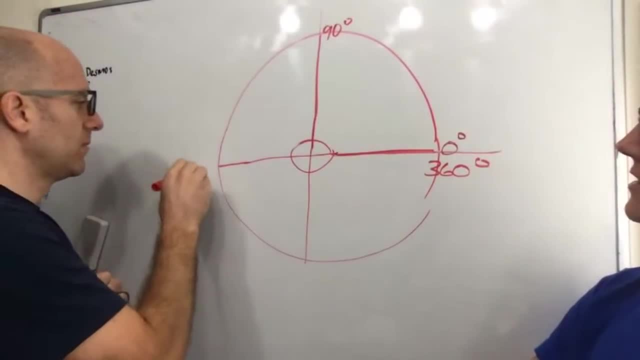 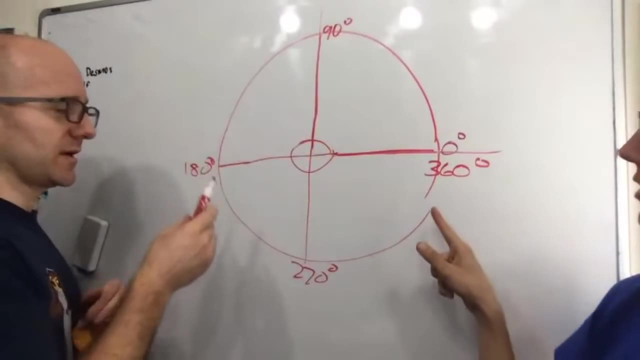 Yeah, Oh, dang, Let's see. So I'm starting here and I'm going this way. That's correct, All right. So here we go: 90 degrees, 180 degrees, 200 is going to be like here-ish. 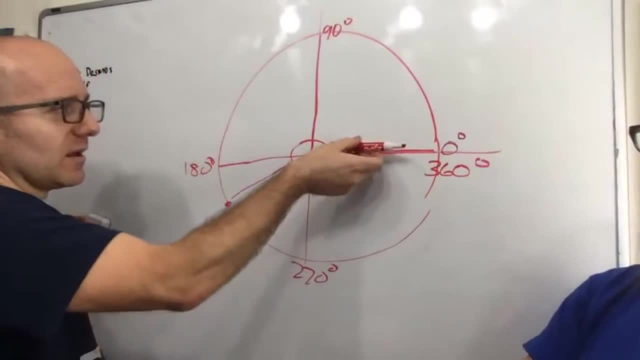 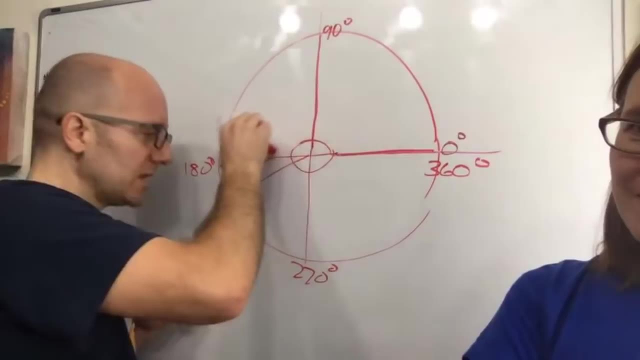 Yeah, probably something like this. So, yeah, I mean, every 10 degrees you're making these steps. Each quadrant gets you, chop it up into 10 degree angles And yeah, so somewhere it's bigger than 180 degrees. 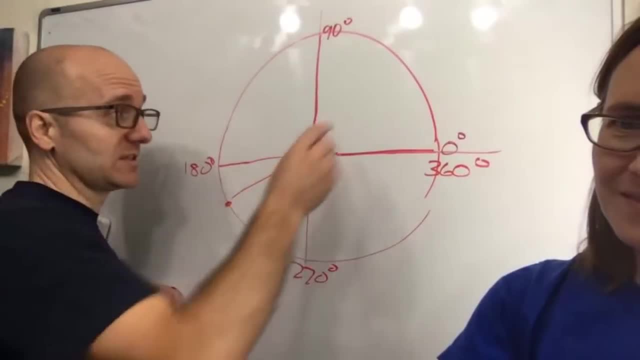 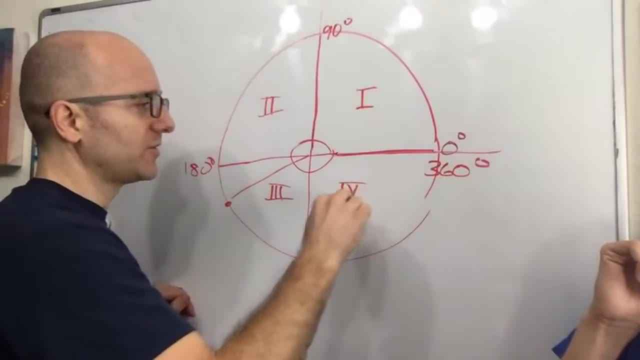 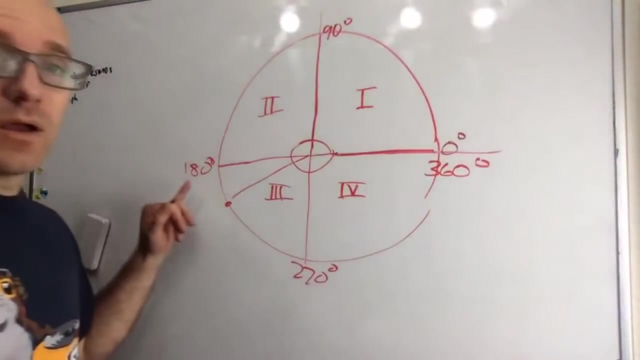 It's less than 270 degrees, So we actually even had a name for this. Here is quadrant one, quadrant two, quadrant three and quadrant four, And yeah, we always use Roman numerals for this. I don't know why, But yeah, so a 200 degree angle ends up in quadrant three. 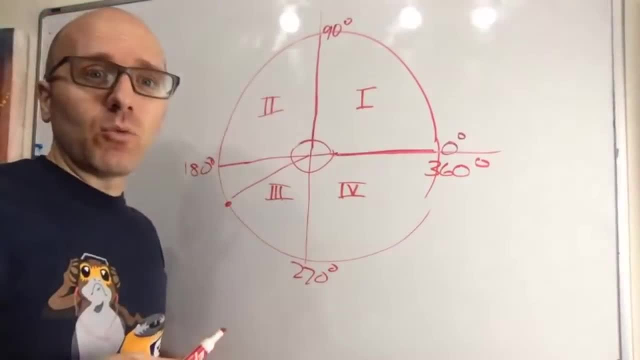 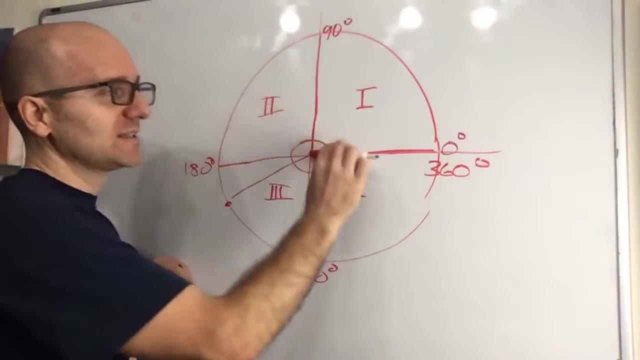 And I could name any angle. I could name. what about a thousand degree angle? Where's the 1,000 degree angle? Oh so in that case, well, you could go 360.. You could go 360 more, So you're up at 720.. 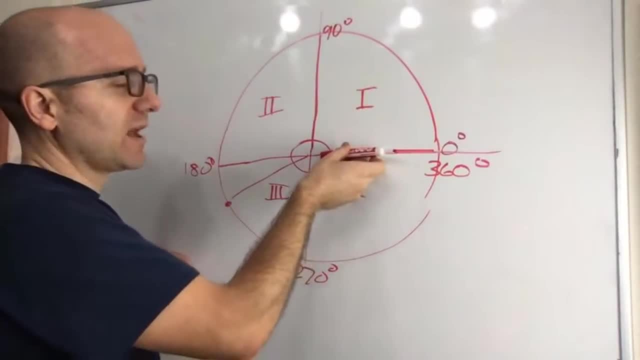 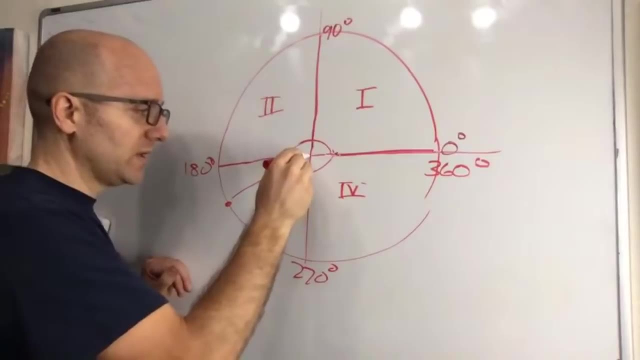 And then we probably need to slow down because if we went around again, that would actually be 1080.. So it turns out a 1,000 degree angle is going to be pointed down here-ish. So did I get that right? Let me just double check. 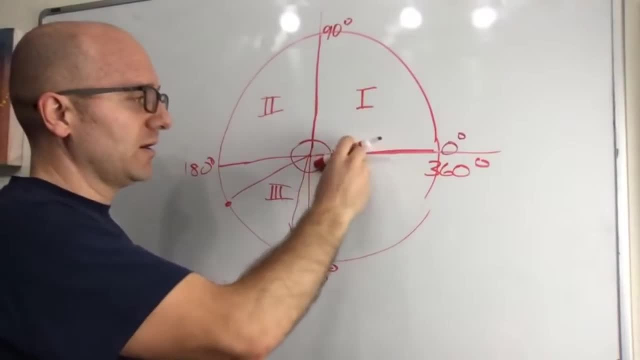 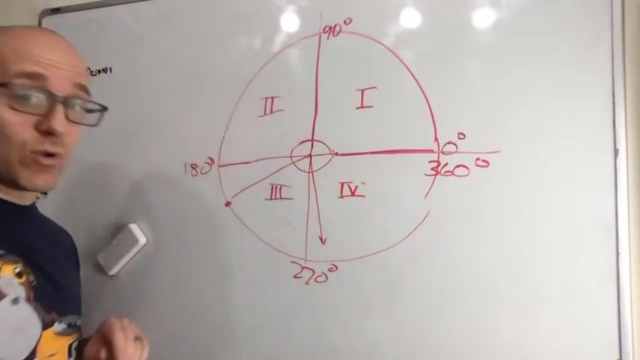 Yeah, So yeah, 1080, three times around- would be here, So I need to subtract. Oh, I needed to subtract 80 degrees. I did get it wrong, So it's pointed somewhere down here So we could wrap around and around and around. 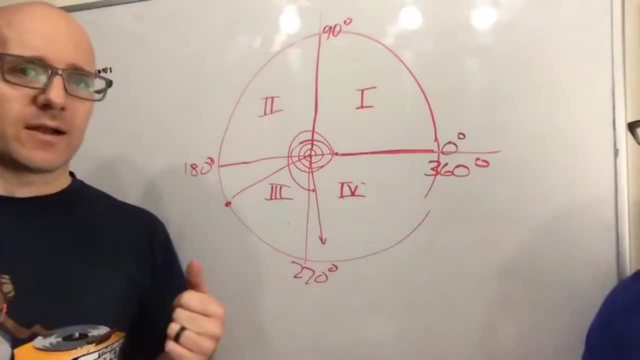 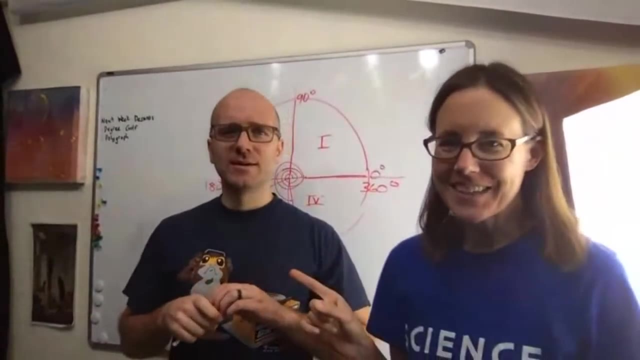 And there is our 1,000 degree angle. I don't know if you can see it. I don't know if you guys have tried this before. if you jump up- So Math Dad has contests with the kids all the time- Be like who can jump and rotate the farthest. 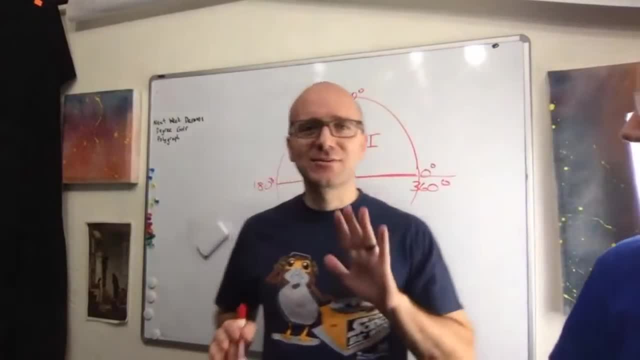 Which is: be careful, don't twist your ankle. No, no, I'm just going to do the 360 here, So I mean, so, 180 like this, I think all of us can handle that, But can you handle a 360?? 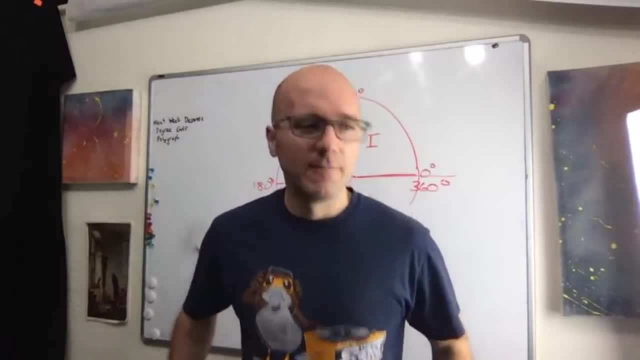 So you're looking, I'll look this way. So you need to jump up and get back to the same position. Yeah, All right, Math Dad, do it again, And then, if you can't do it, you can't do it. 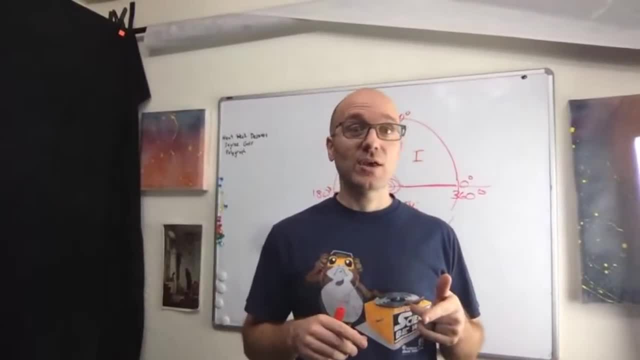 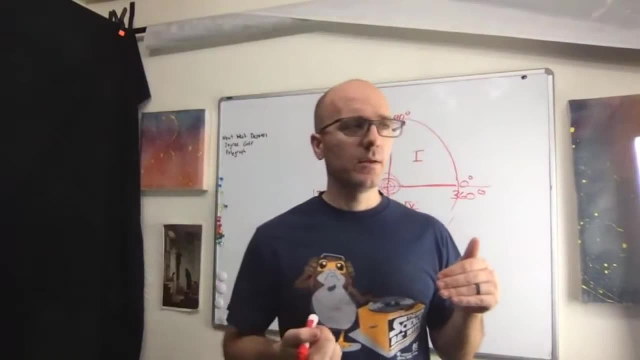 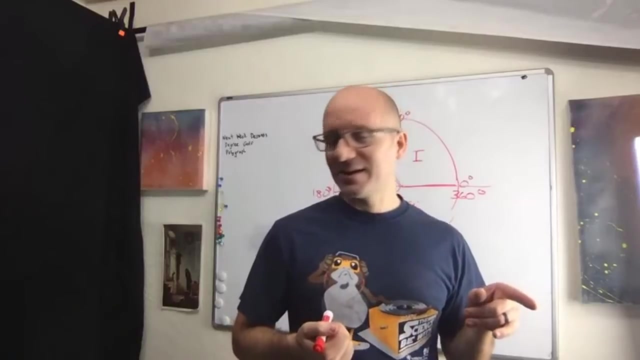 And if you can do a 360, then you want to see: oh, can I go even further? And then try to measure how far it is that you've gone. All right, what's the farthest you can go? Oh, I can almost do a 720,, although I'm totally not trying that here. 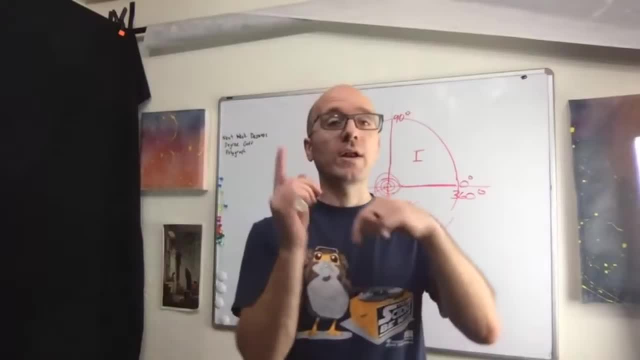 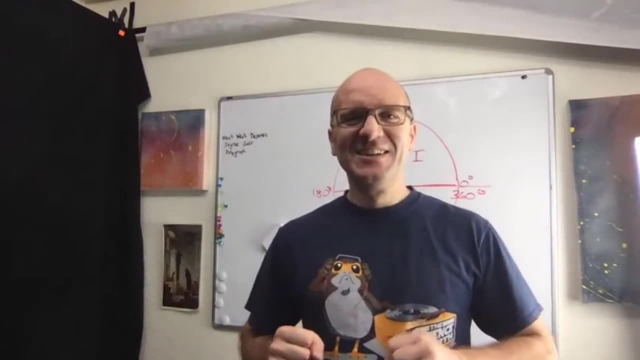 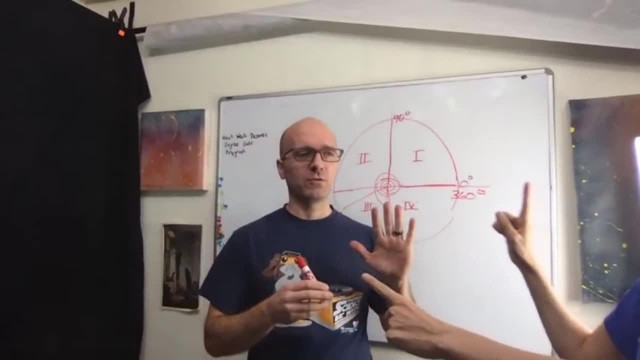 All right, Whoa, whoa, whoa, Yeah, almost, Almost, Almost, facing the opposite direction, which would have been a perfect 540.. So if you jump and you're facing where you were, that's 360.. Yep, 360 would be one time. 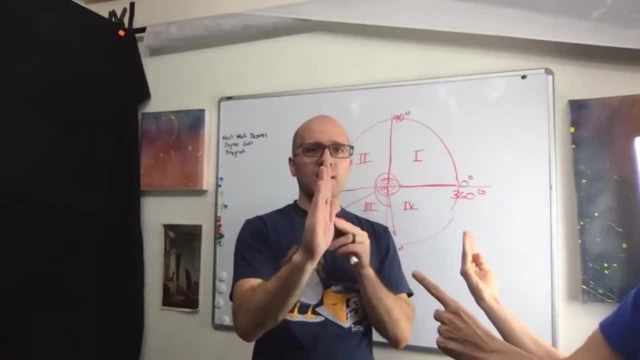 And then if you add 180 degrees on that, Then you're at 540. So I'd be facing away from you, The opposite direction. Yep, Pretty cool, But yeah, we don't have a lot of room in here. Kick this table too many times. 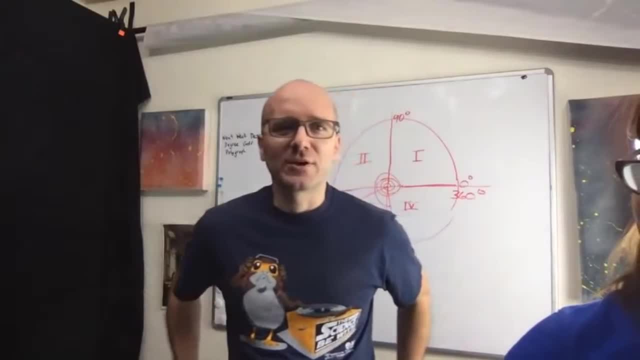 And Unplanetistic says: do a 1080.. That would be like a lot of room in here. Yeah, I mean, I don't have a lot of room in here. I don't have a lot of room, Something's going to work. 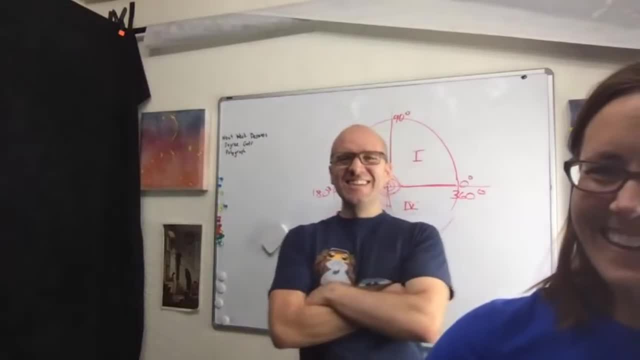 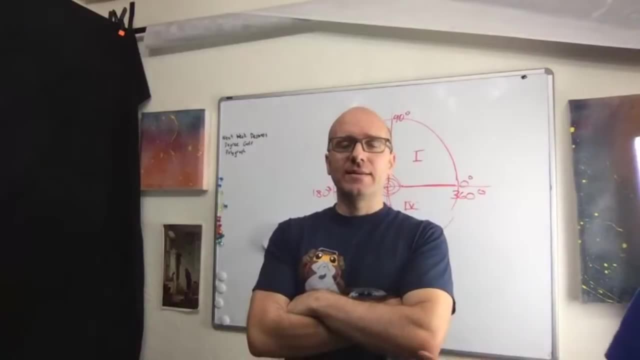 A lot of time And Unplanetistic says: do a 1080.. That would be like Olympic level of athleticism, right there, right Yeah, I wouldn't be surprised if there were. Maybe if you're on ice skates, Yeah. 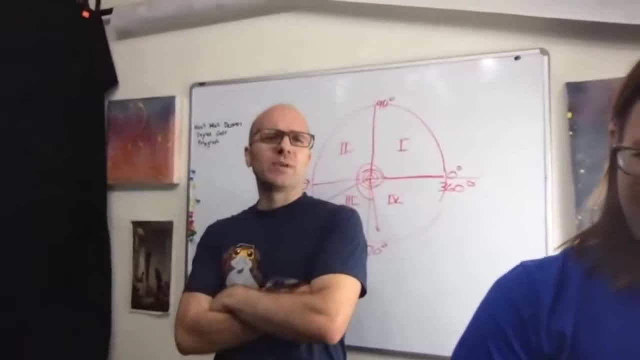 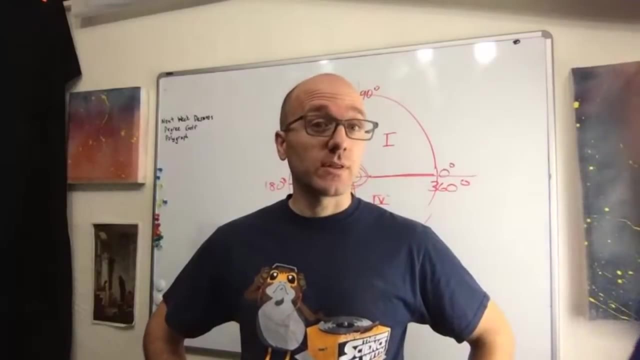 Oh yeah, yeah, Ice skaters can do it. Yeah, Olympic gymnasts maybe get a bunch of momentum, Maybe they can pull off something like that. But 720, there are people that can do two full circles, So yeah. 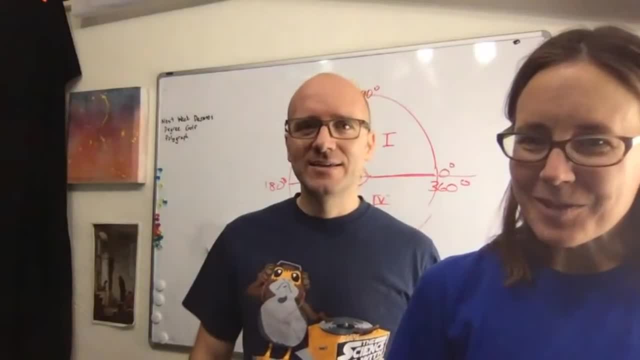 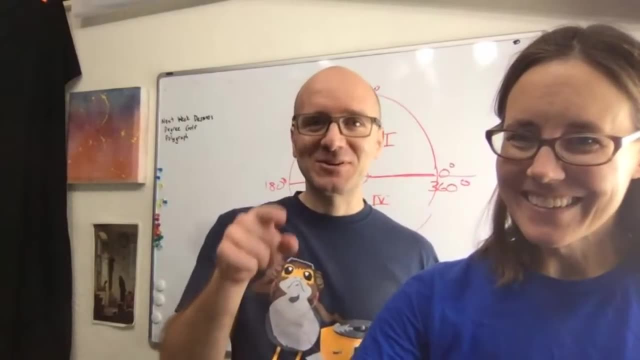 Give yourself a little bit of space if you're going to try this. Yeah suggests on the trampoline, or king husky suggests on the trampoline. that's a good idea. they're trying to get me injured. this is what they're trying. we do not have a pool or a trampoline. 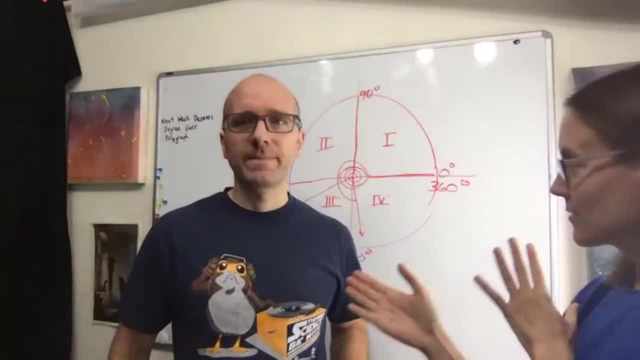 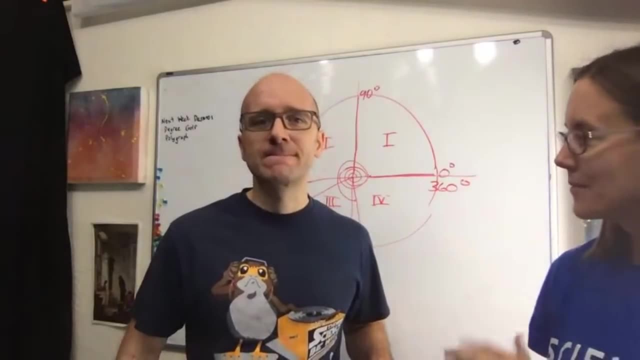 no, all right, are we? is the math lesson complete? anything else you wanted to say about? we got lots more to say about circles, but are we have time? we, we have about 10 minutes. so, no, we've got. we've got a bit. we're a little bit of time, okay, so just a few more. what are the? 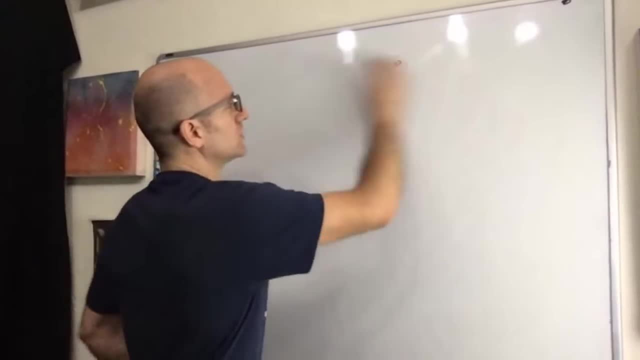 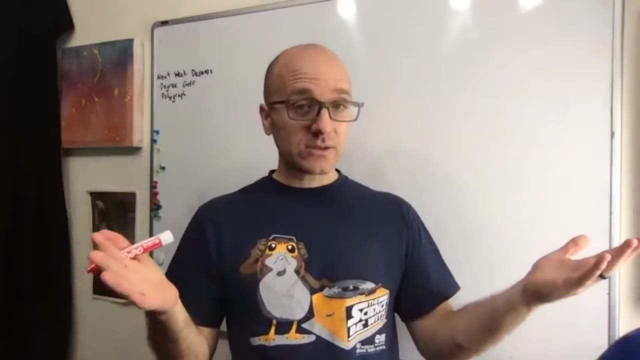 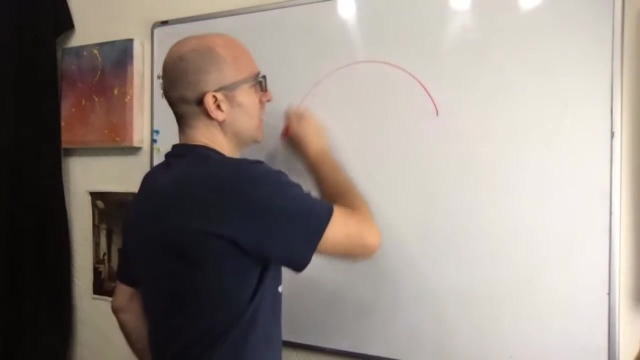 things that we are supposed to know about circles. well, it turns out, and as you get to junior high and then into high school, you're going to learn more about circles, and i wanted to give you a few of those formulas that you're going to encounter along the way. so, first of all, sophie, age 11, can 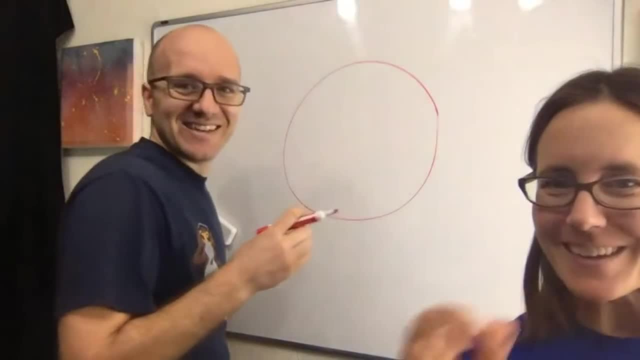 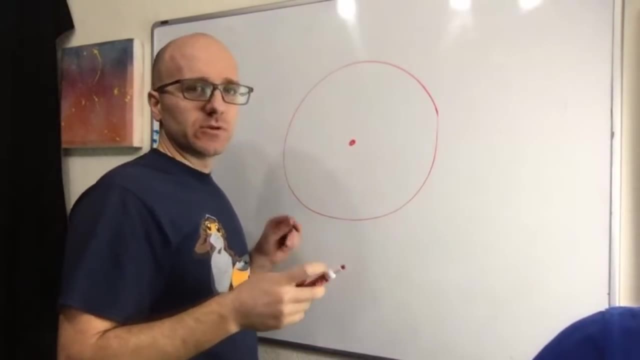 do a 360. sorry i'm. i'm just really entertained by seeing all of the comments about jumping in the chat and who can rotate so far. so, first of all, how does one draw a perfect circle? well, there's this tool called the compass, where one end stays at the center and then the other end rotates around. 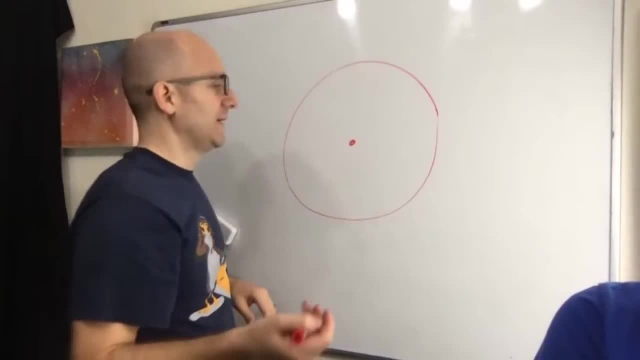 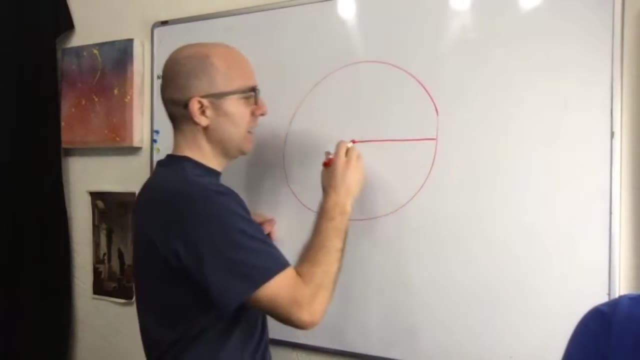 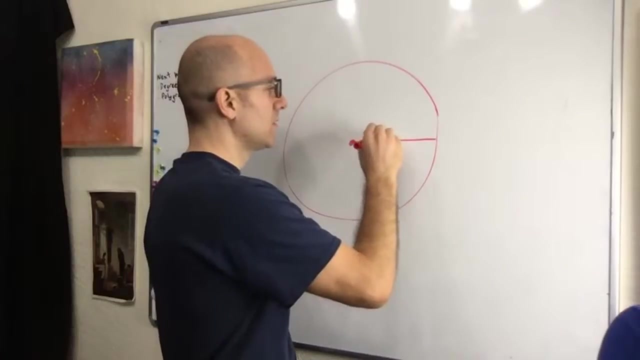 that center point and you can actually draw a perfect circle, and it's kind of satisfying to see it look so nice. okay, so what are the pieces of a circle? well, if i draw a line from the center to the edge, that distance is called the radius. if i draw a line from one end through the center, 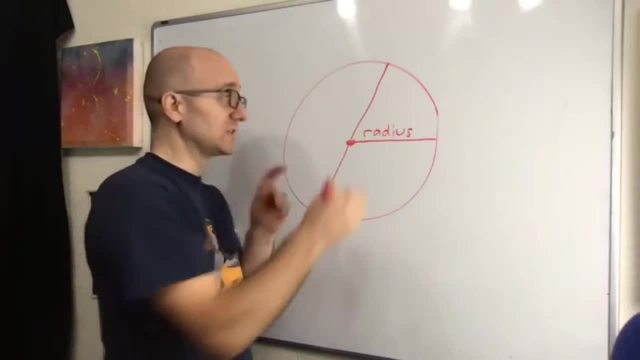 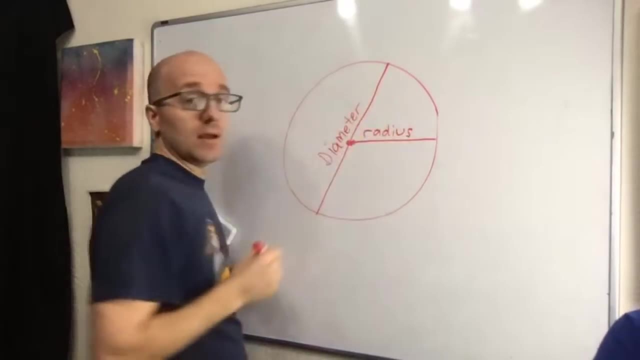 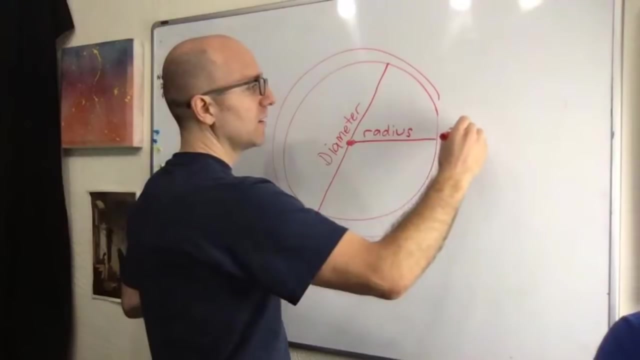 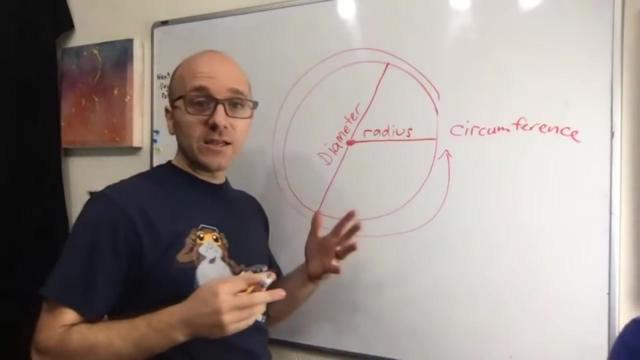 point to the far end. so that's twice as big as the radius. that one we call the diameter, and if we're talking about the distance around a circle, we call that the circumference. there's just just some handy words that we need to know and there are some formulas that relate 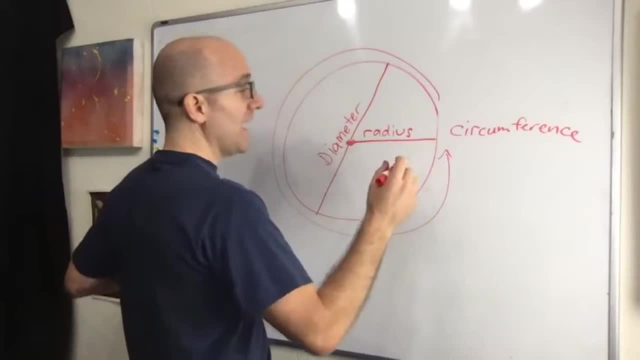 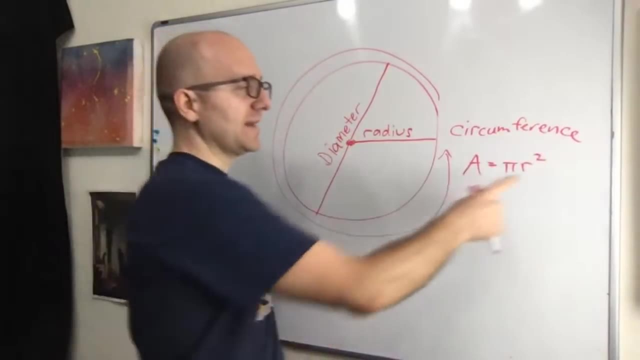 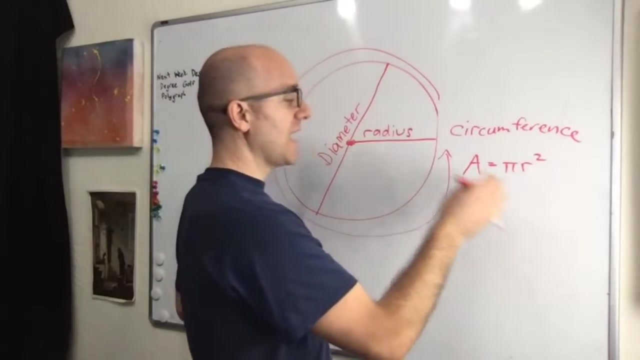 those. so in this case we're going to call it the circumference and then we're going to call it the radius. so in this case the area of a circle is equal to pi r squared. so pi times radius, times radius, and the circumference of a circle is the diameter times pi, or often we'll just write that as: 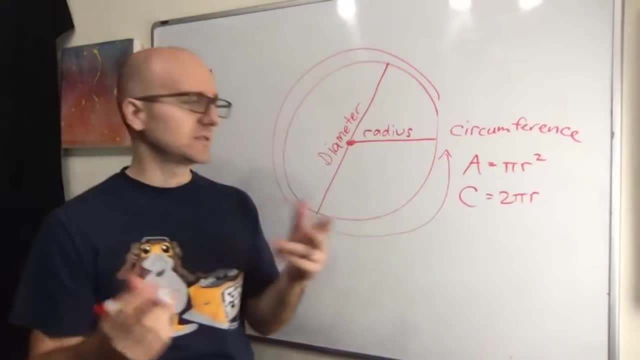 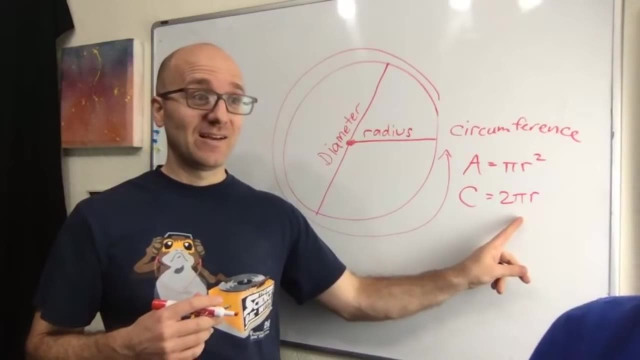 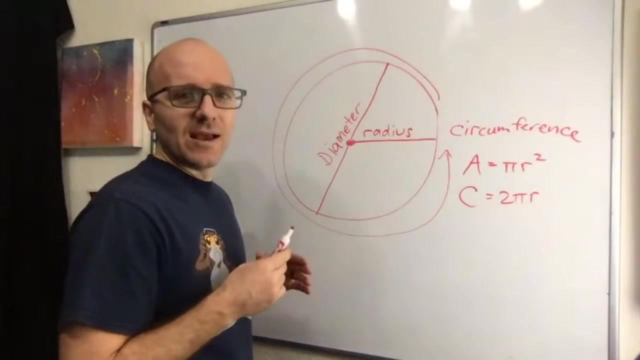 two pi times the radius, because two radiuses will be the diameter. now, what is this pi that i'm talking about right here? hmm, yes, this is a mathematical constant. i think we've brought it up before on the show. but where does it come from? well, it's what you get if you take the distance around a circle, so the 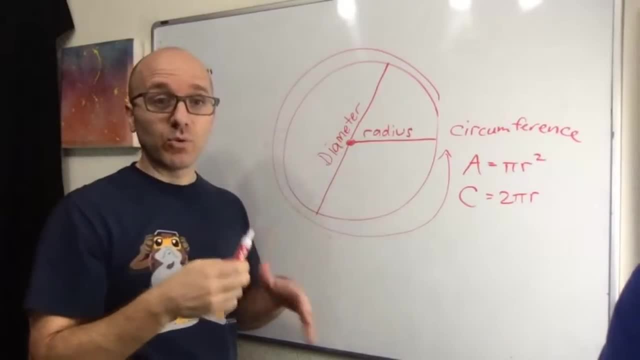 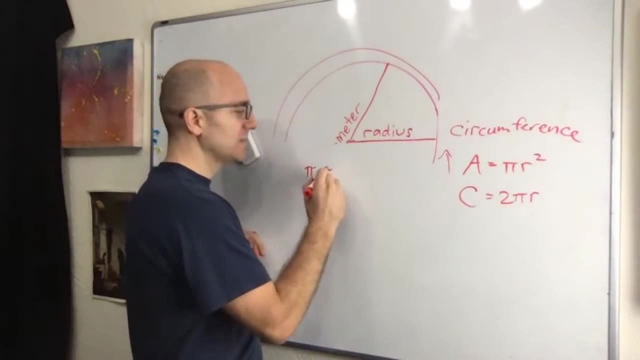 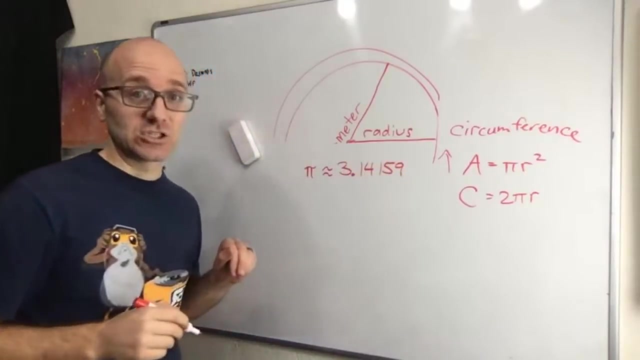 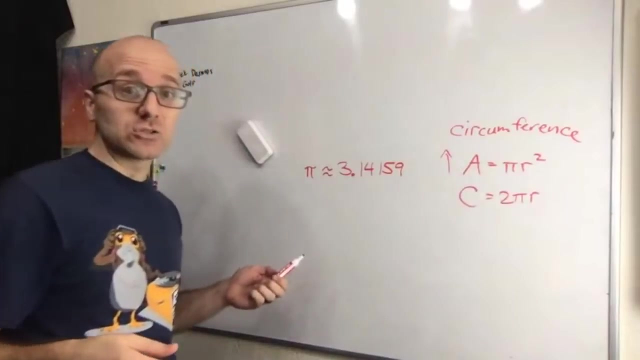 circumference and you divide it by the diameter, you always end up with pi and it works out. if you calculate this, pi is approximately three point one, four, one, five, nine ish. but those decimals are actually go forever and ever. they never repeat. this is what we call an irrational number. 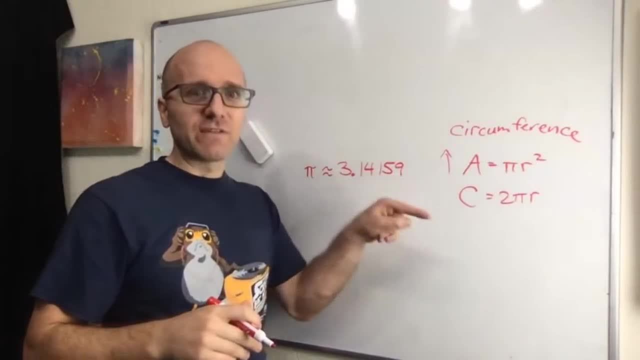 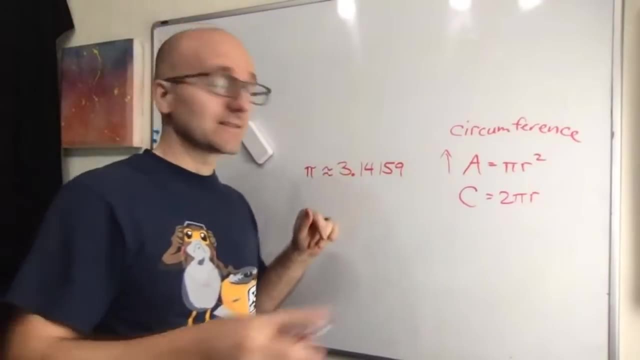 so pi is three point one, four, one, five, nine, two, six, five, three, five, eight, nine, seven, nine, three, two, three, eight, four, six, two, six, four, three. uh, that's about as far as i've got it. but yeah, thanks, but yeah, um, you can never get that all the way, and there are people who have actually 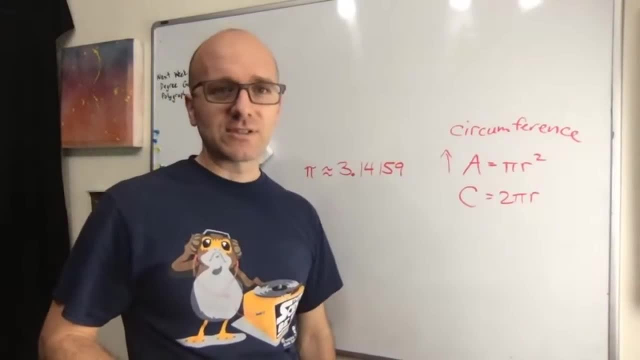 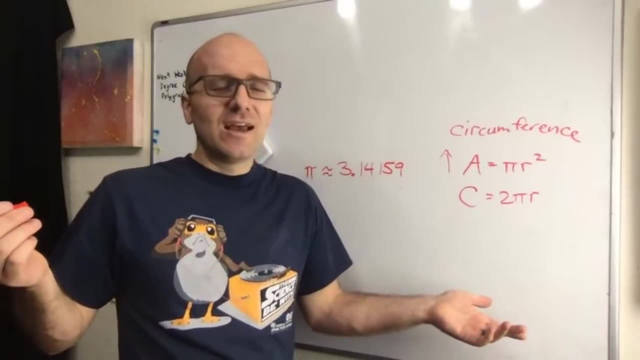 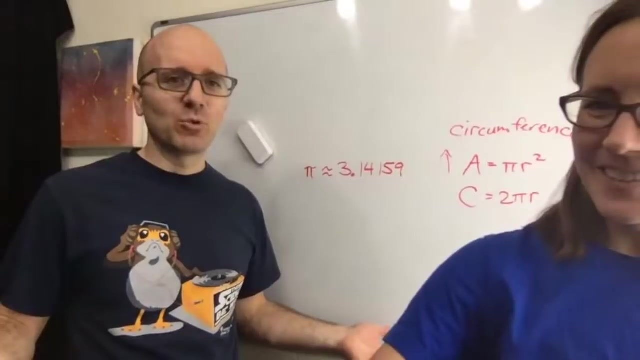 memorized 50 000 digits of pi before, which is insane for on multiple levels, just that they're able to do it, but also that they chose to do it, because once you have the first 20 decimals or so that there's no calculation you would make where you need more decimal places than that for pi. i. 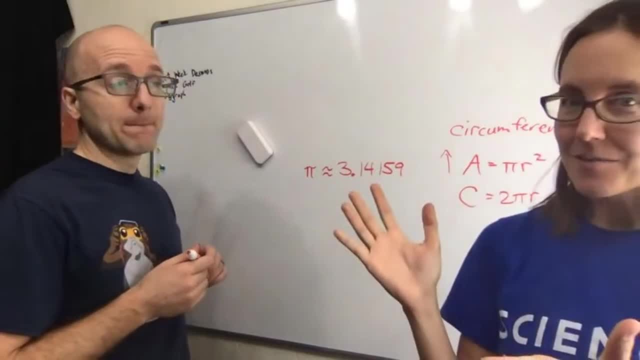 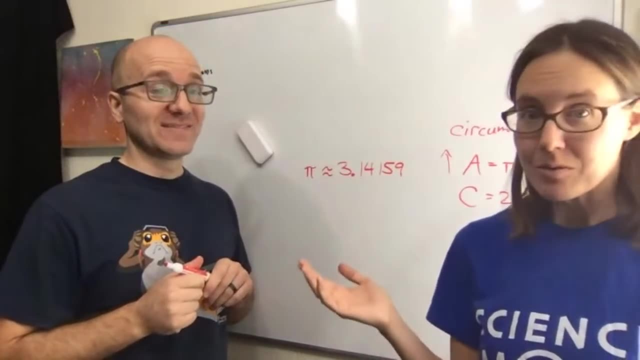 have a quick question for you about circles. yeah, what if, instead of dividing them into 360, what if we picked different numbers? because you could divide a circle equally into 12 degrees instead of 360 degrees, absolutely. and so so why why 360? why 360? so this goes back to the ancient. 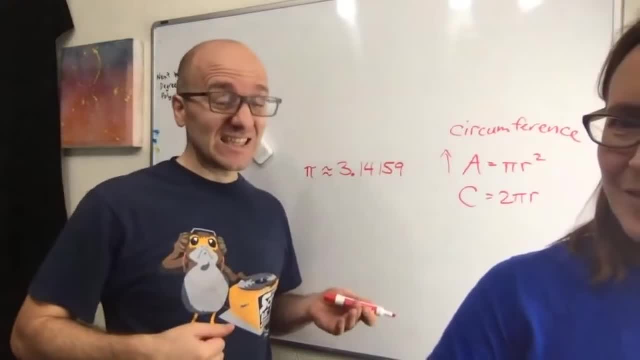 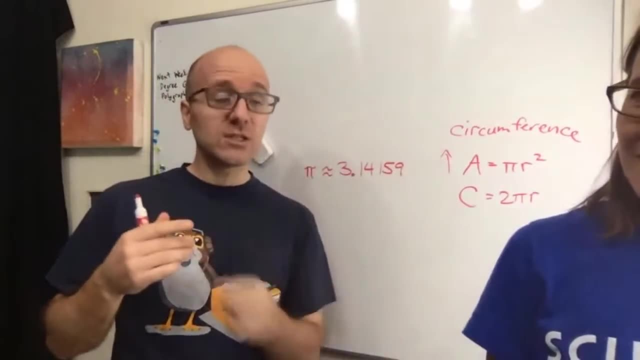 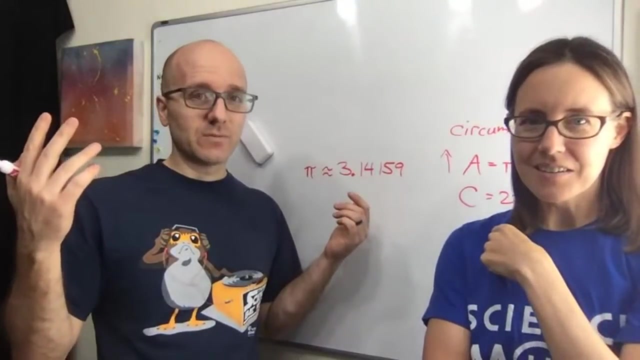 babylonians. they used the number system, base 60, which is also kind of interesting. so we use base 10. every time we get to a 10, we move out a new digit. well, they used base 60, so does that mean they had 59 different digits? um, yeah, 60, 60 digits, yeah, the zero, and i actually don't know a ton about. 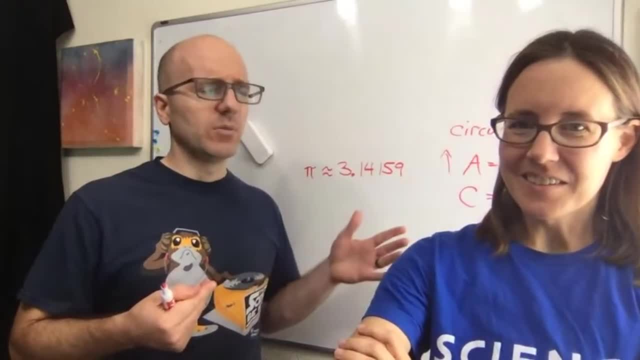 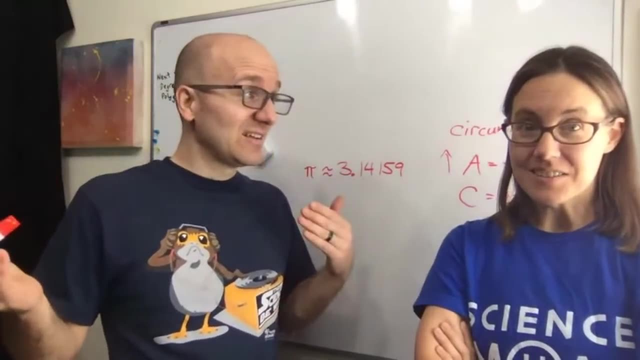 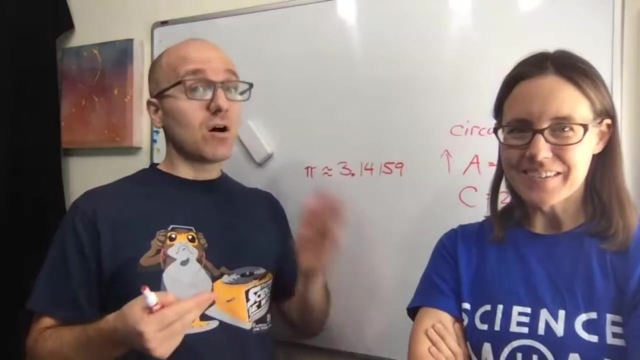 their mathematics or why they did things certain ways, but yeah, that fundamentally they use base 60. well, and guess what? how many minutes are in an hour? 60, 60 minutes? and that's where that comes from. that's where that comes from, yeah. how many seconds in a minute? 60 seconds. yeah, this base 60 is all over. 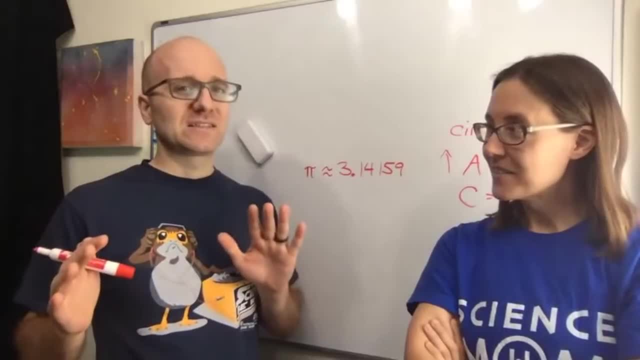 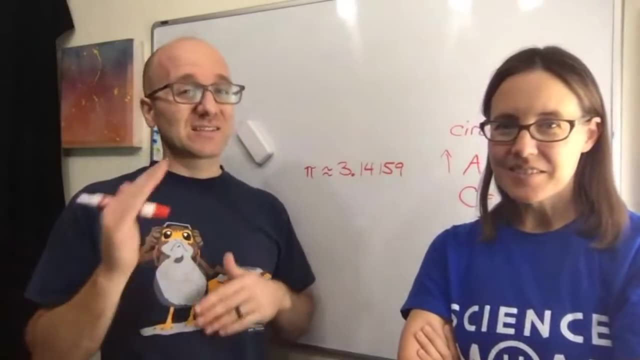 the place. now it turns out that mathematicians actually use a different measurement for angles rather than degrees. i mean, we can use degrees if we want, but it's kind of like the celsius versus fahrenheit. like, if you want to, the one that makes more sense is actually celsius. it's based off of. 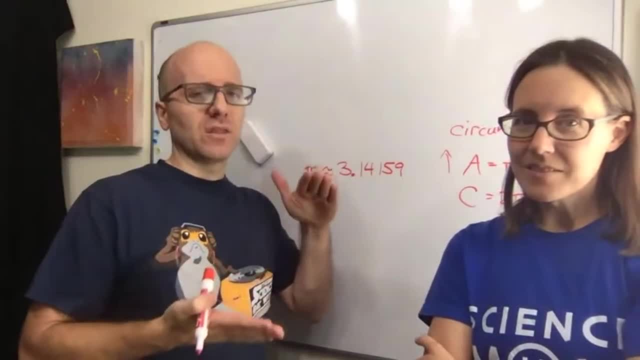 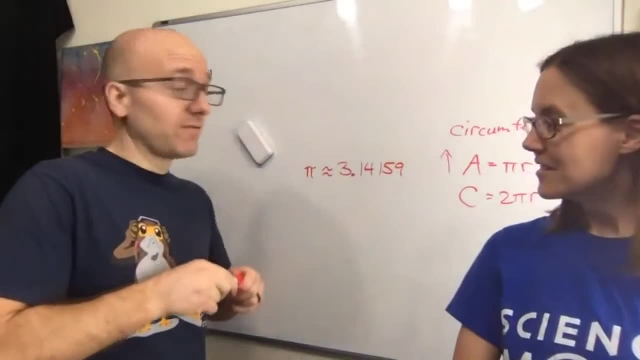 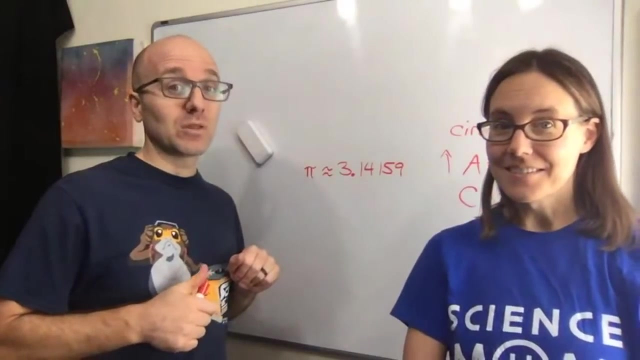 something and it's more uniform measure. that, yeah, it carries a little more meaning. well, mathematicians do something called radians, so we could even talk further about circles, talk about how do you get their equation in the plane. we're gonna skip that, but i'll just let you know it has to do with pythagorean theorem. 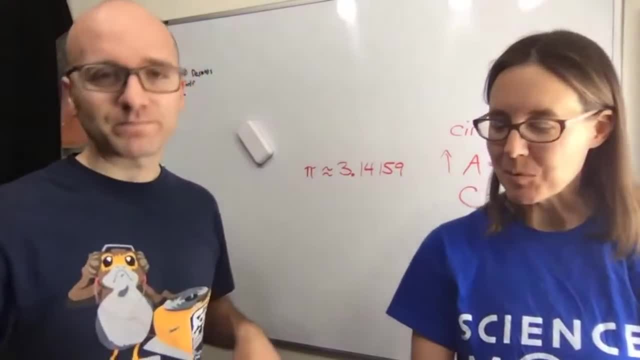 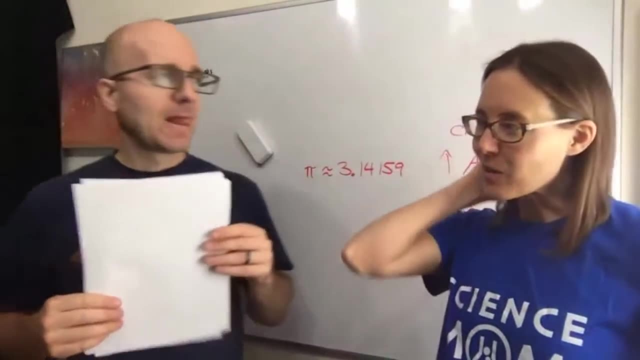 and yeah, kind of kind of fun. we'll save that for another time, but it's time for what's in the bag now. all right, what did you? so math dad came up with our riddle. so i gotta ask: did you actually put something in a bag? i, i didn't, because 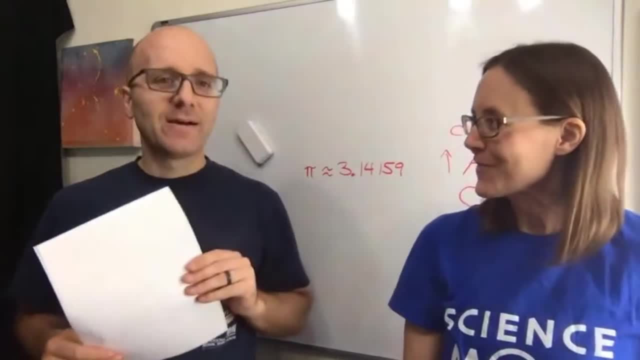 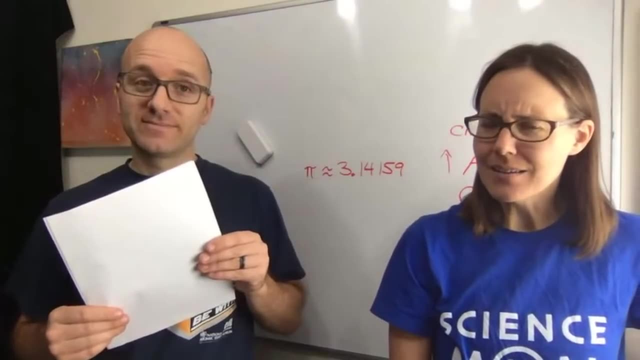 yeah, because you didn't put stuff in bags. yeah, i usually forget to. all right, all right. so the more i dry the wetter i get, the more i dry the wetter i get, huh, all right, give me a little more. i'm a little, i'm stumped. you use me every day. 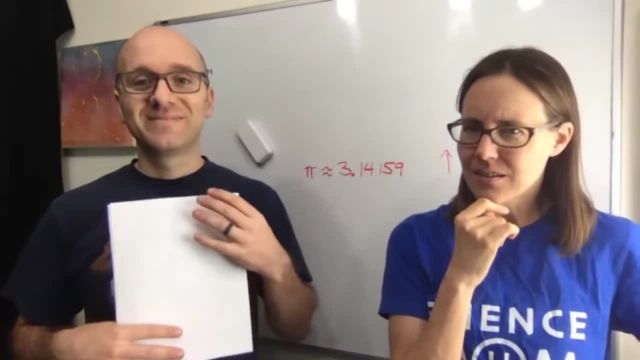 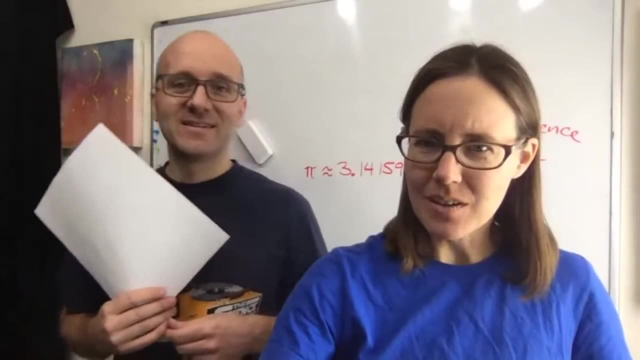 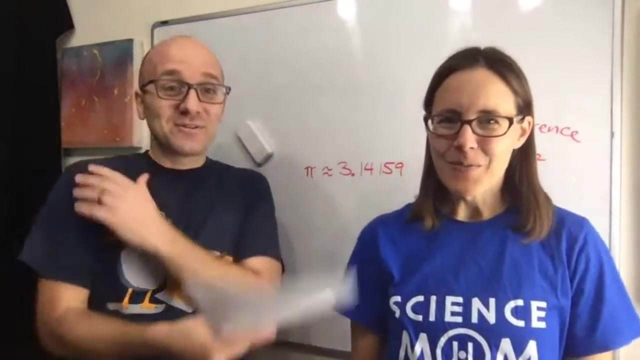 the more i dry the wetter, i get all right. what. what gets wetter when it dries out? i am, oh g man, a towel, larissa. a towel, that's totally it, because it's a towel. though the more the towel dries you off, the wetter it gets. yep, was there another part of the clue, or no? just that you use me every day. 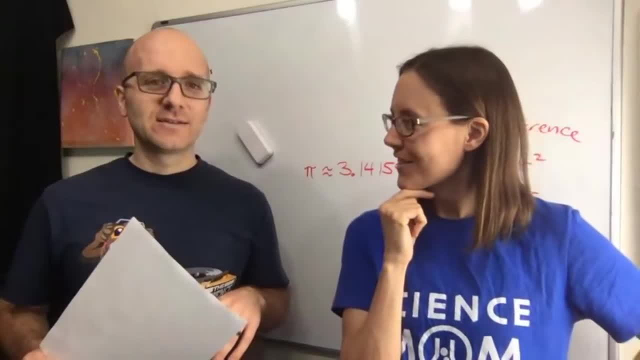 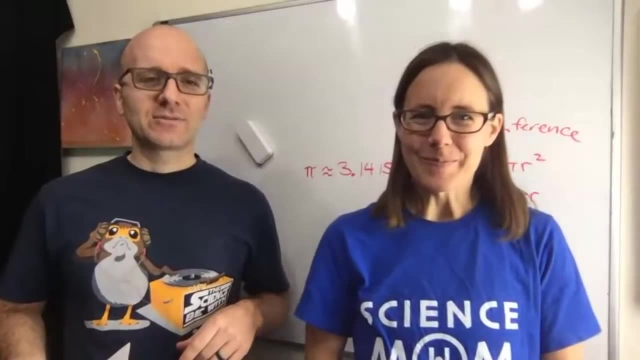 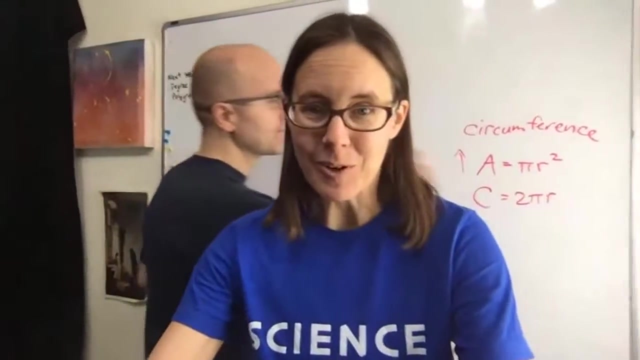 use your every day, unless you don't shower every day, and then you don't. you wash your hands, right? yes, okay, use a towel when you wash your hands. awesome, that's a great one. yeah, i was pretty stumped when i saw it, so i was: oh, yeah, that's a good one. i like it now real quick, before i. 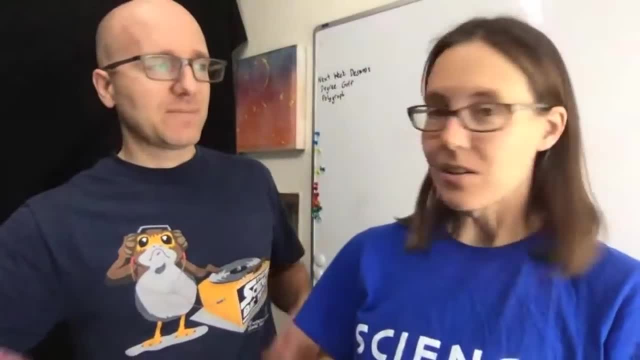 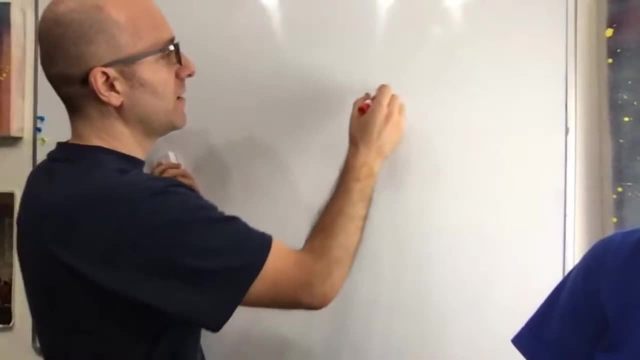 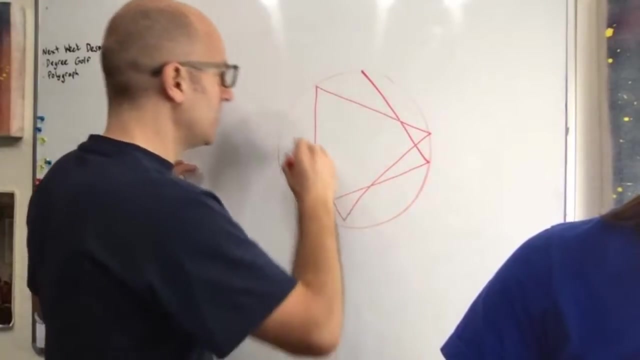 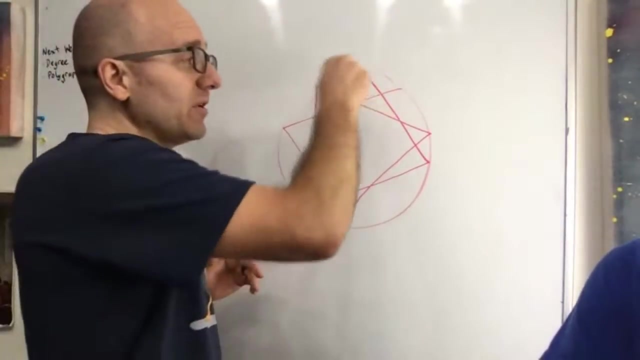 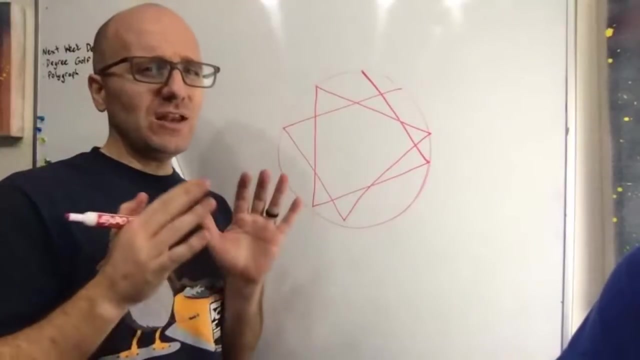 show you the engineering challenge, okay. so last time our math mystery involved a laser beam that was bouncing around the inside of a clock or whatever shape we were looking at, and it depended on the number of numbers and how far it was jumping each time. and the question was: how do we know when we're jumping? 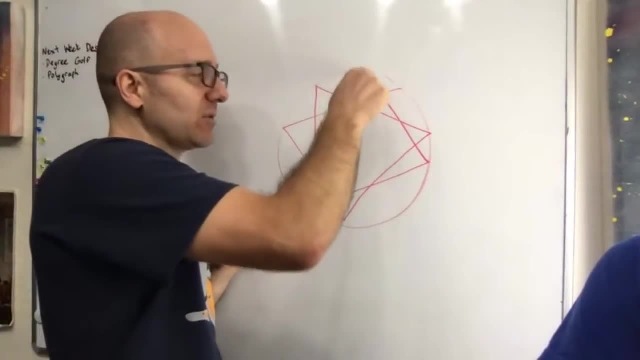 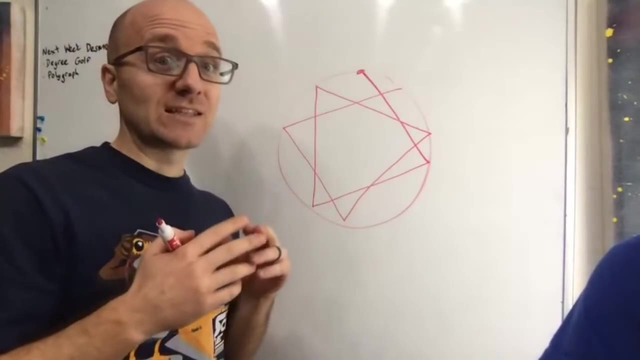 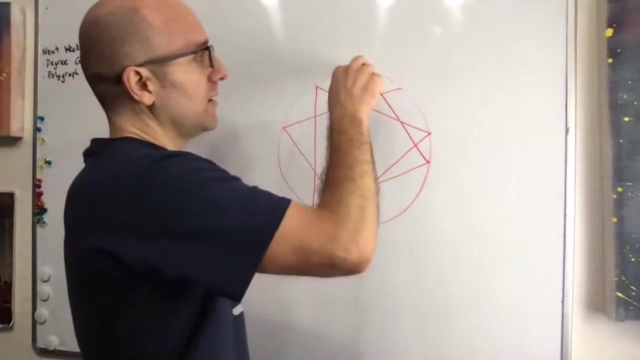 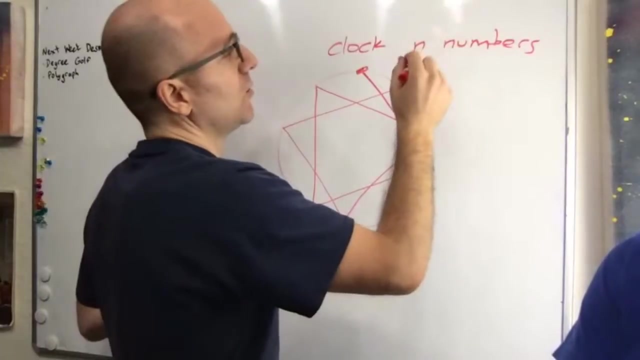 know when this laser beam will actually hit every single number on our clock. And I even made a little Desmos activity where you could play around and I saw that some people had actually figured it out. So the secret is you? so if the clock has N numbers and we always jump by K numbers, 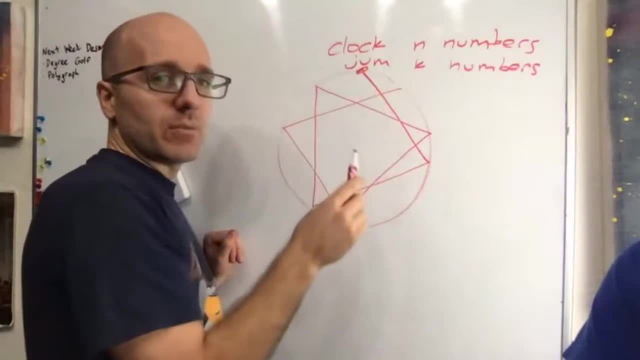 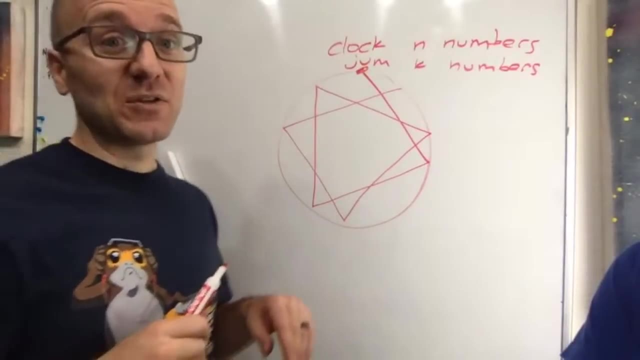 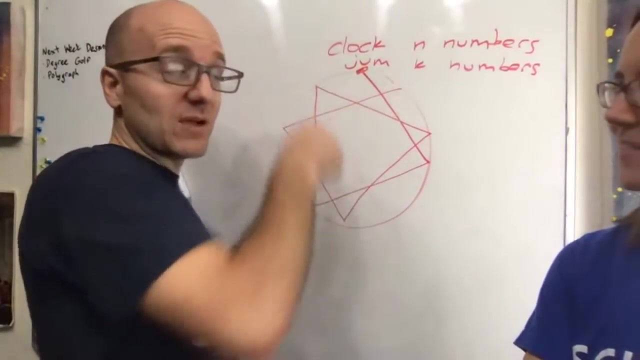 then we will hit every single number if, and only if, N and K have no common factors greater than one. So if their greatest common factor is one, then that's enough to guarantee that when this bounces around, it will hit every single number. It's kind of like the opposite of the answer to. 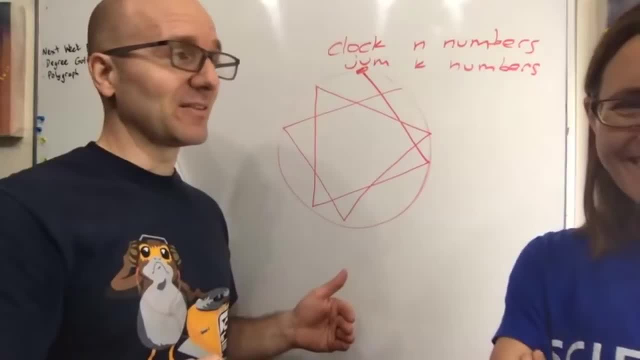 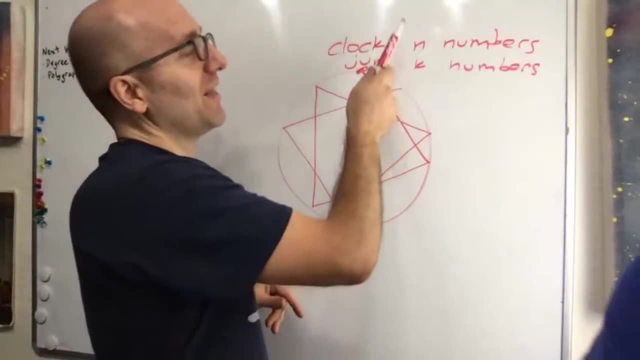 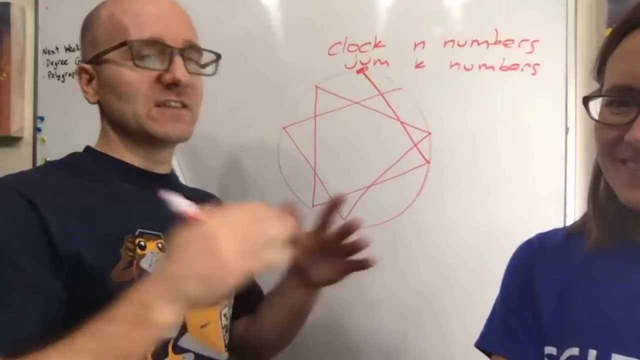 the previous math mystery about the king. That's right. The numbers that were visible to the king were exactly the same: The pairs of numbers where the two coordinates didn't have any common factors other than one. but the ones that were invisible to the king were the ones that shared common factors. That's right. 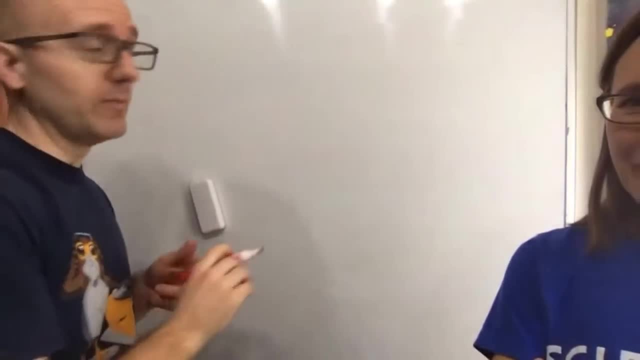 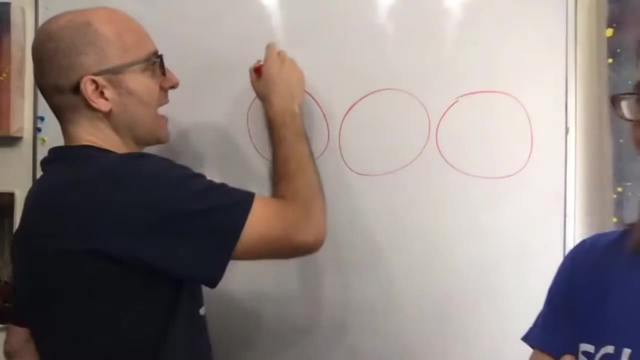 Yeah, Okay. So today's problem is also a clock problem, but this one's going to be a simultaneous clock problem. So in this case I've got three different clocks. I have an eight hour clock, a 10 hour clock. 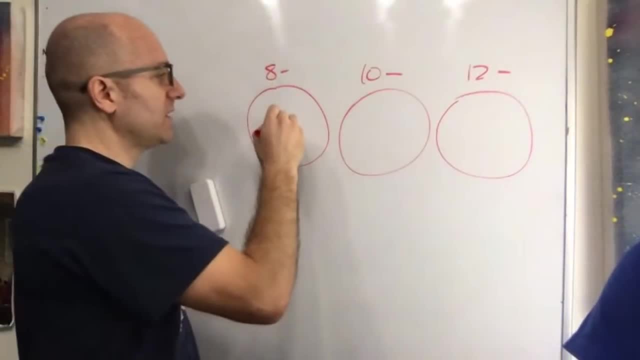 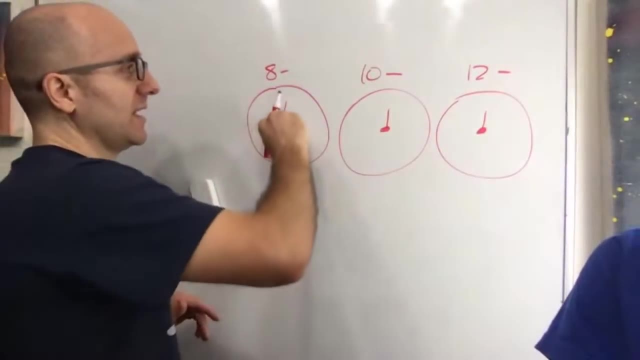 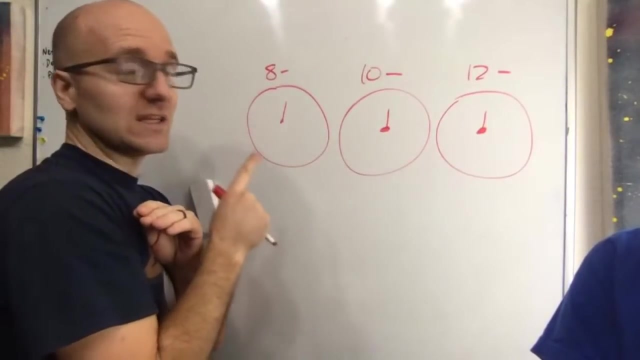 and a 12 hour clock, And all three of these are going to start pointed upwards at the same time. But and so we say: go, all three clocks start. And my question is: how long will it take before these three clocks all are pointing back up at the 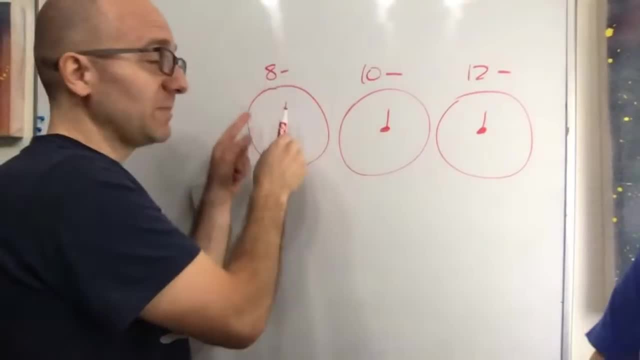 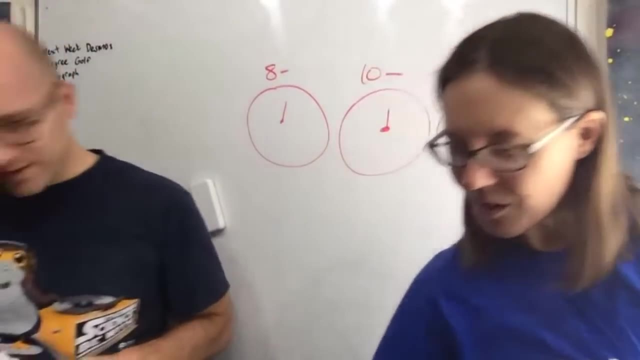 same time again, But they're going at different speeds. This one goes around every eight hours, So let's just draw. Do you have another marker? No, I lost the markers. All right, here we go. So in eight hours, this one will go all the way around and it will be pointing. 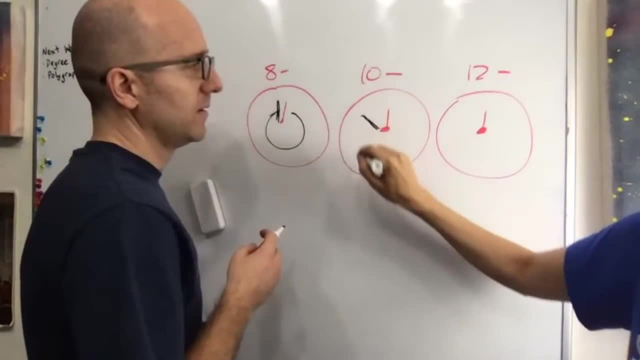 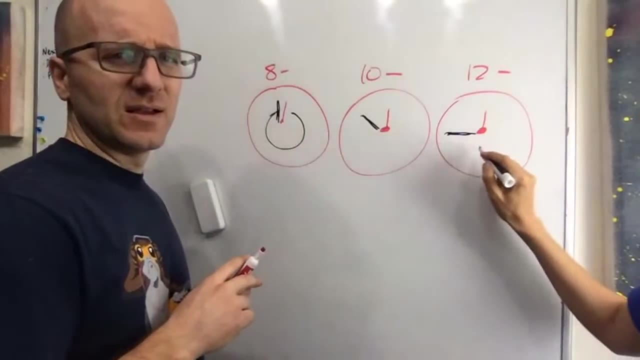 straight up again, But this one is only going to. it's going to be two hours away And this one is going to be four hours away. So in eight hours they're not lined up. How many hours until they all line up again? 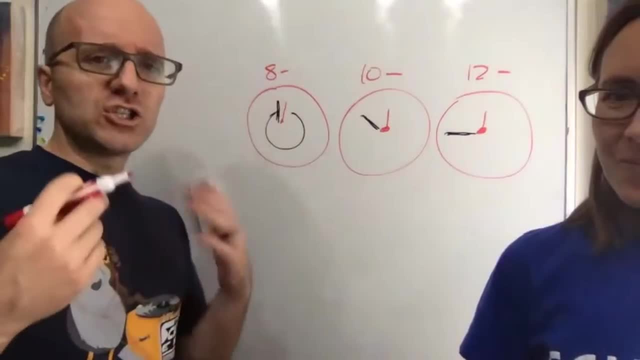 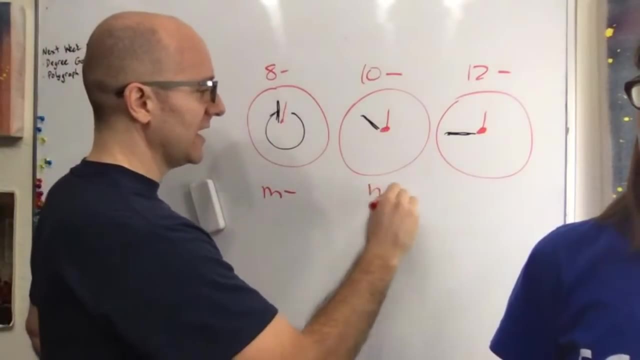 Yep, But that's exactly the question. And then, of course, the more general question is: well, what if this one had I don't know M hours? this one M hour clock, this one was an N hour clock, this one was a P hour clock. In that case, 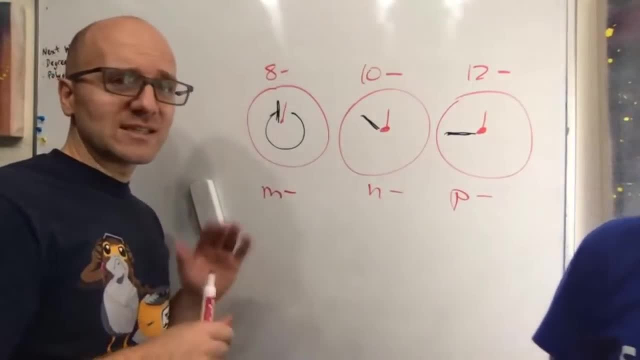 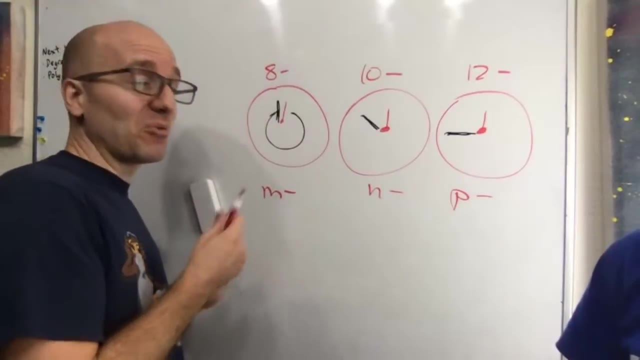 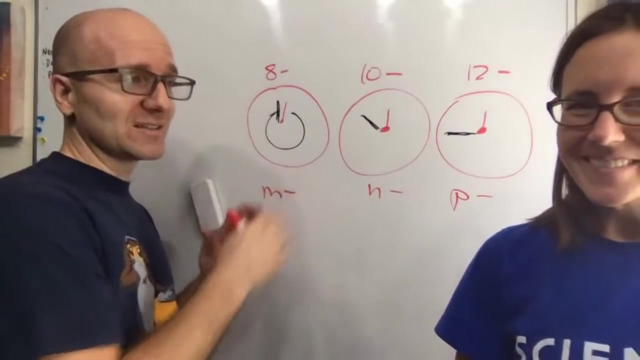 how do we actually figure this out in general? So it's not a question with an obvious answer. It's the type of problem that we need to experiment with and see if we can come up with some reasoning behind what's going on. There's definitely some order to this. So there's our math mystery, for 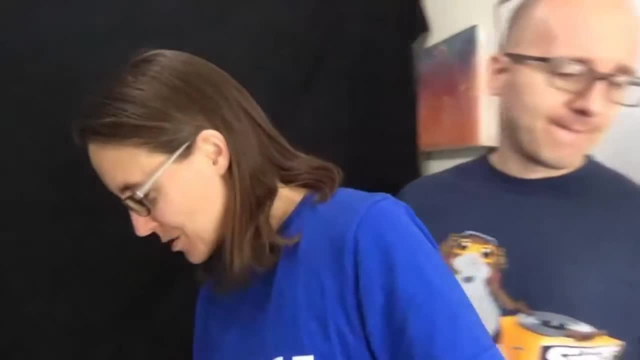 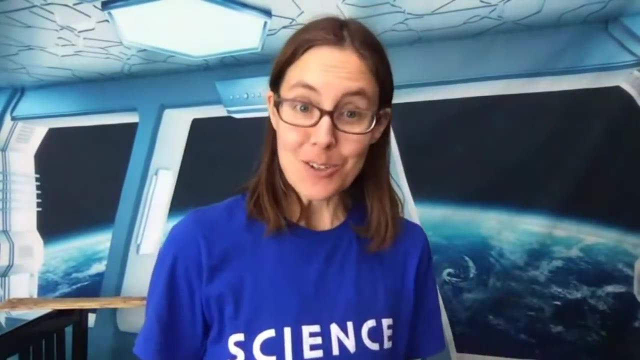 tomorrow- Awesome. Thank you, Math Dad. And then let me turn this around real quick. I want to tell you guys something real fast, and then I'm going to show you some awesome pictures of real life use of block and tackle or pulleys- So quick. 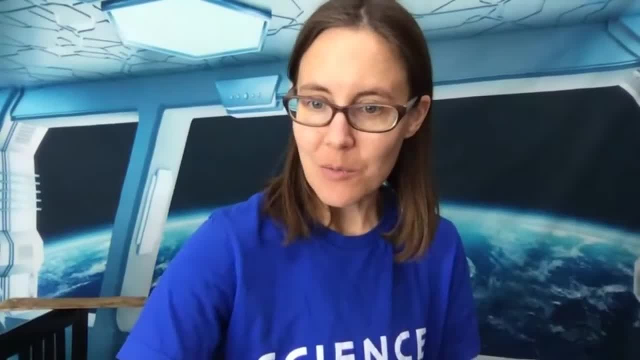 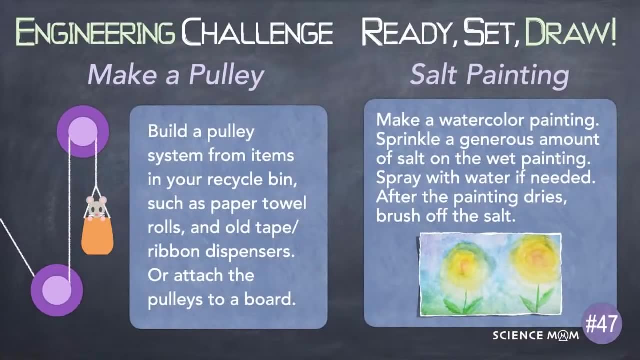 reminder that our art prompt for today. oh, my goodness, and we are, we're kind of running out of time. That's okay. We have the art showcase too. So real quick, make a pulley and a salt painting. That is the art. 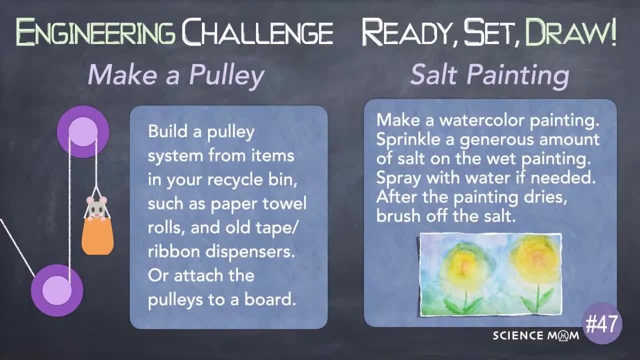 prompt for today? Whoa, a salt painting. Yes, So you just do a watercolor painting, but then sprinkle a bunch of salt. Yes, Sprinkled a bunch of salt on it. Salt on it. Spray it with water if you need, And then, after the painting dries, brush off the salt. 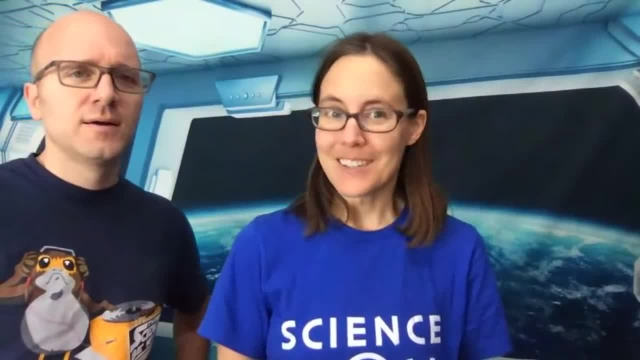 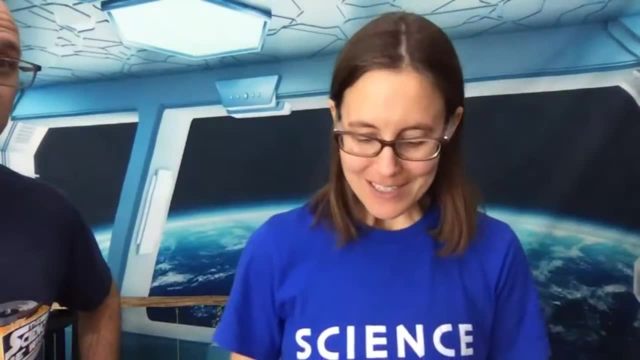 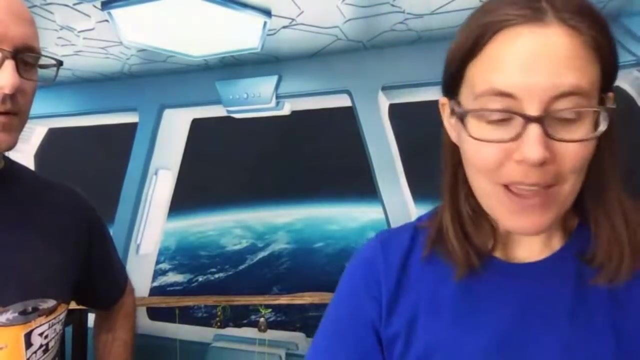 The salt is going to create really cool patterns with the watercolors. That's a real, that's a real fun one to do. And then let me show you some real life examples of block and tackle. So when I worked for the Forest Service- which was one of the best jobs ever- we would make these. 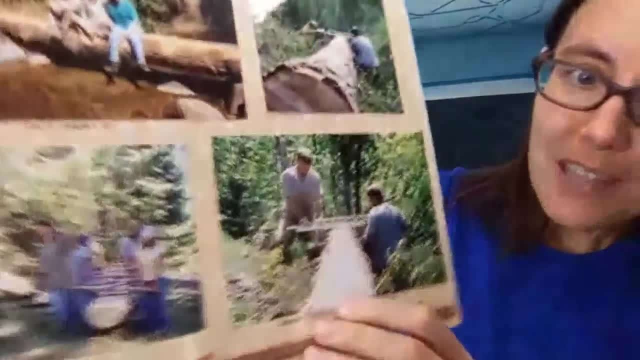 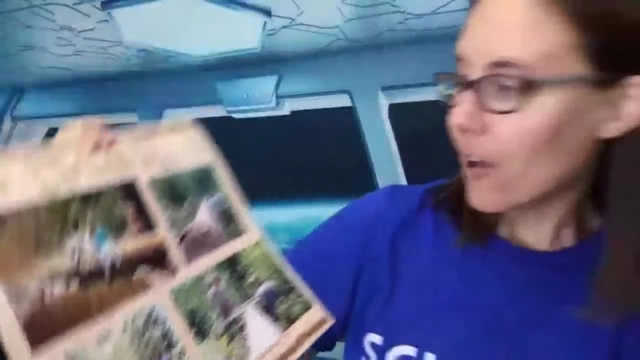 bridges- And they're not technically a bridge because they're not engineered- but we would take a log and then we would saw off And then we would carry it and place it across a river so that then you could have a stream crossing where people could go across the stream and not get wet. 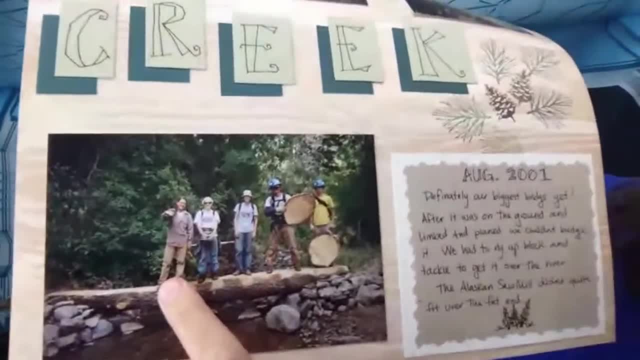 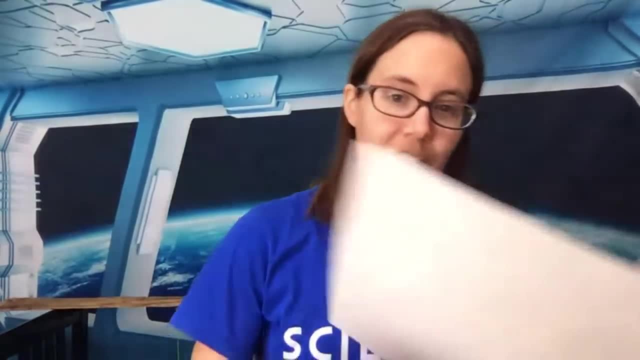 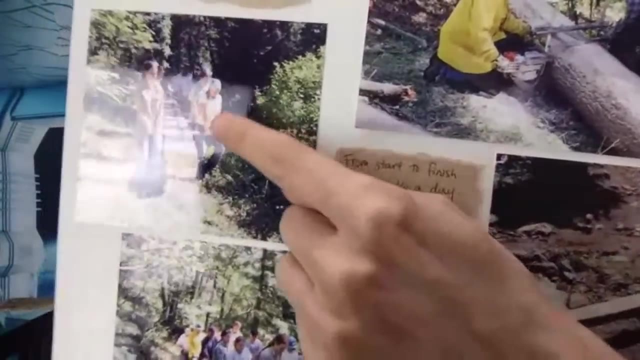 So there is. can you guess which one is Science Mom? That's me right there holding the chainsaw, And this is one of the bridges we made. Well, this bridge was so big that we actually could not carry it like this. So even with the whole entire crew, you know 12 people and all of these log carriers here the bridge was. 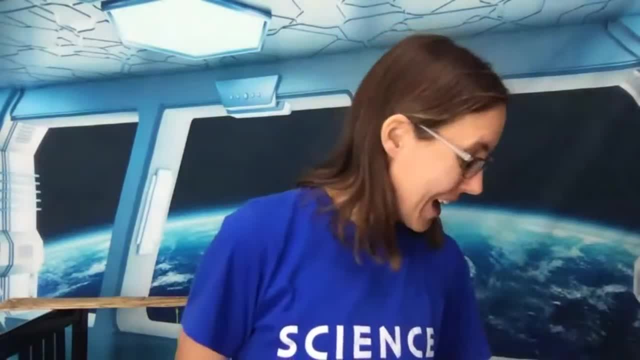 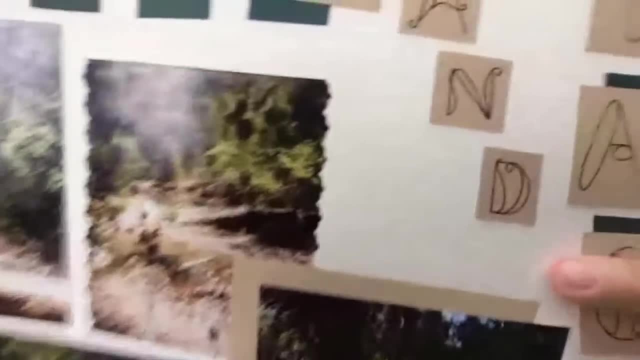 too heavy to carry. So what were we going to do? How are we going to get it across the creek? Well, we had to use block and tackle. So here is- I'll get just a little bit closer so you can see the pulley. 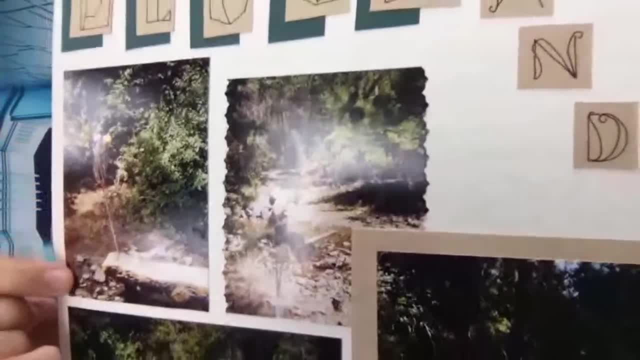 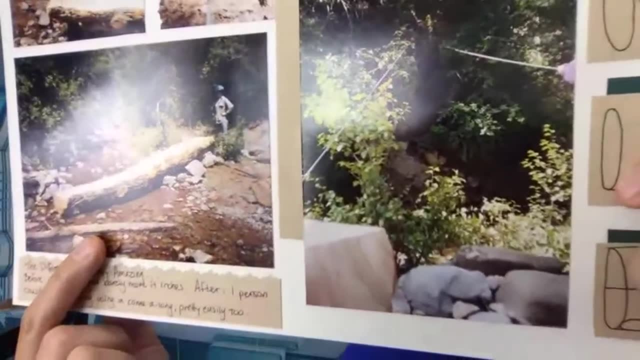 So here is the pulley here that you can see, set up tied to the bridge and using that block and tackle system, One person was able to move this entire bridge using a come along, whereas 10 people with log carriers couldn't lift it. 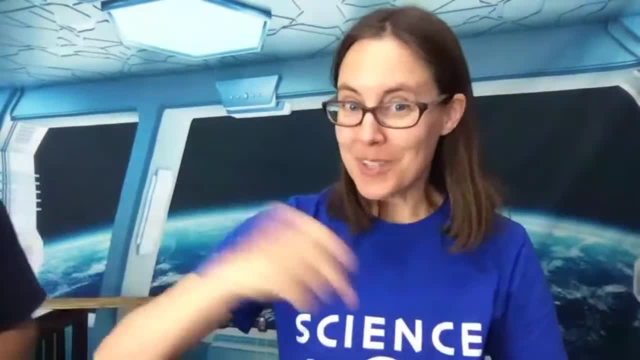 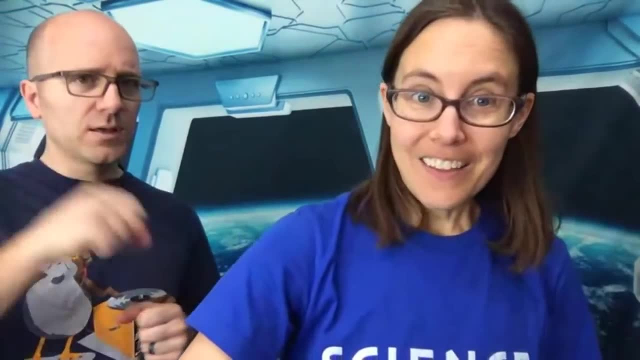 It was too heavy With block and tackle. one person just using a come along and a winch was able to move it And it was slow work. It was just like bit by bit, So that's a compound pulley, Yeah, yeah. 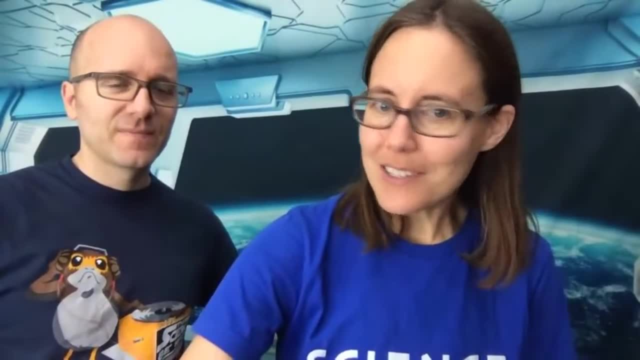 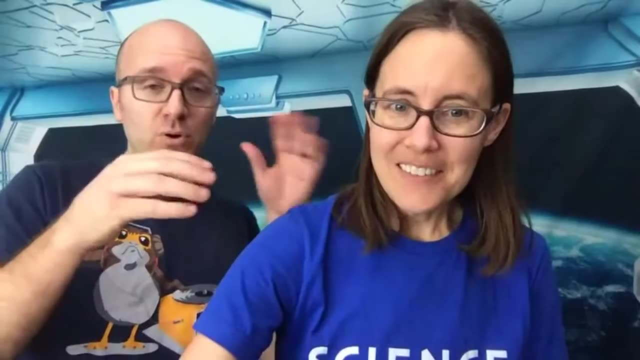 And, if no one's, maybe describe real quick what is a come along. for people who haven't seen a come along before, They're a really cool tool. Yeah well, so you've got this compound pulley, So it's wrapped around multiple times, which means, of course, that you're going to get a huge mechanical 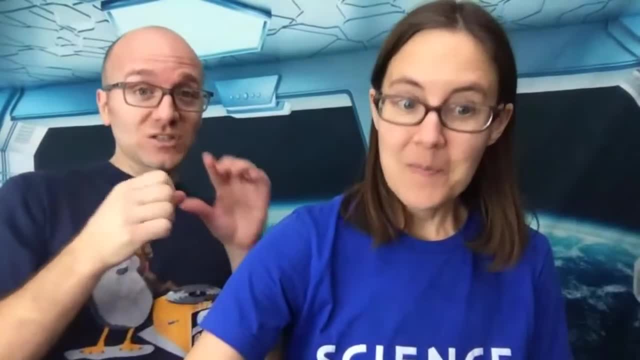 advantage. But you're going to have to pull the string a long ways to get you to the top of the bridge. So you're going to have to pull the string a long ways to get you to the top of the bridge. So it's just a little bit of actual motion, but you're actually even able to use a crank. 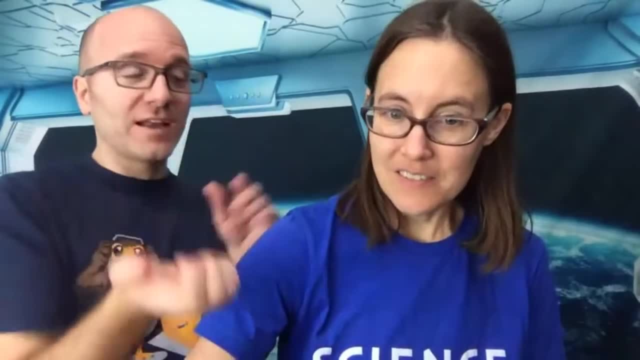 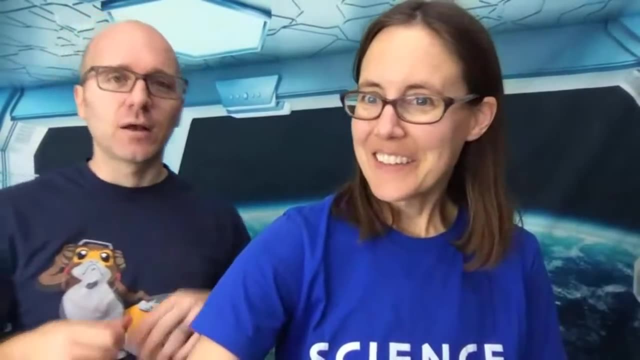 So you've got kind of this lever part mechanical advantage that's allowing you to pull the rope, which is giving you additional mechanical advantage through the pulley. So it's a complex machine because it's combining multiple simple machines. It's really cool. 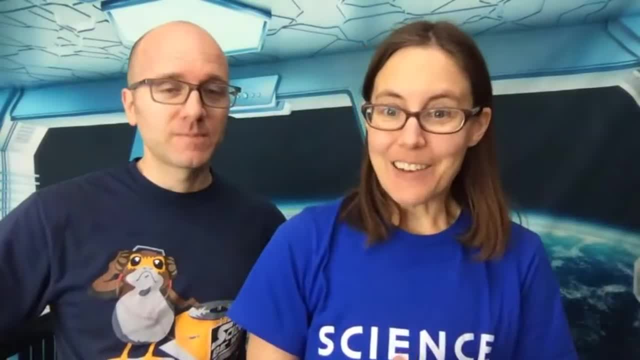 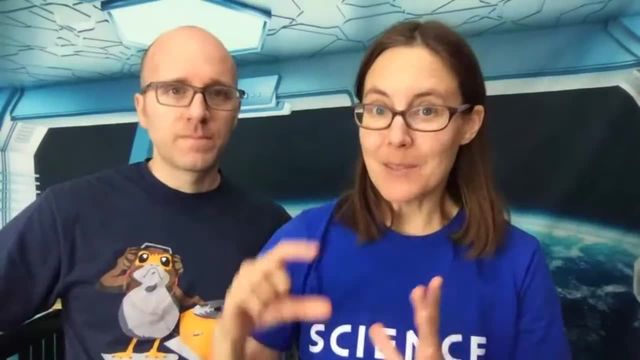 And now we're ready for our art showcase. And if you are new to our show and not sure about where to submit art, post it on Facebook Or on Instagram. we have an album that's pinned to the top of the page or you can email it to art at science dot mom. 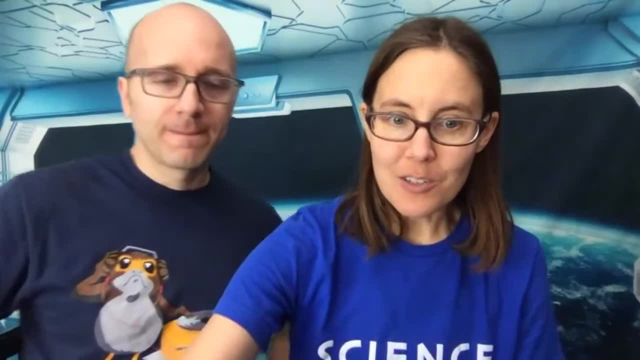 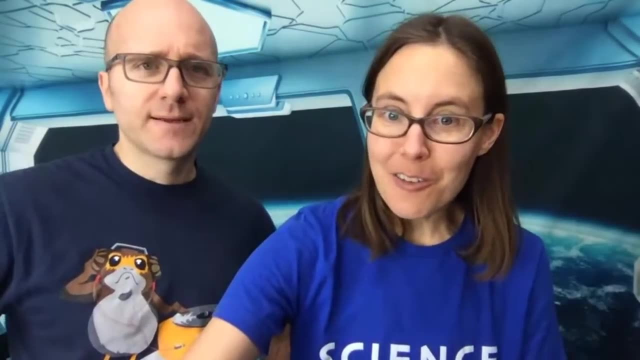 But posting it on Facebook is the best, best way to get your art featured. So I'm going to share the screen, because yesterday's art prompt was pointillism, which is kind of a style of modern art where you take dots and you arrange the dots to create a picture. 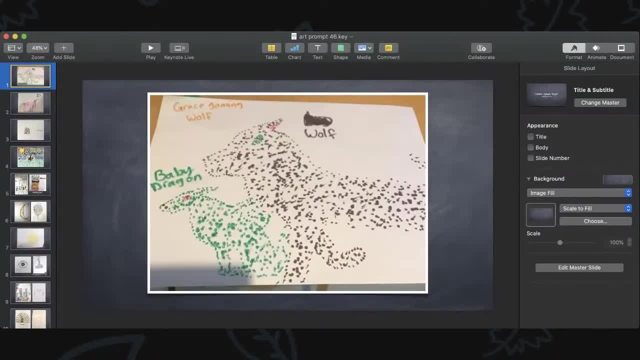 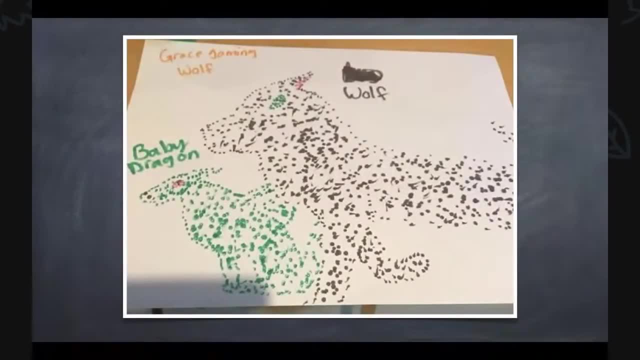 This sounded like a really hard prompt, So it's it's. it's quite a bit of fun and you can use any type of medium. So from Grace Gaming Wolf, we have a wolf and a baby dragon. I love it. Kathy did a unicorn. 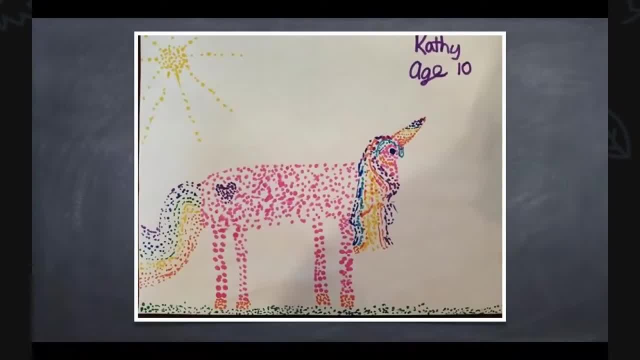 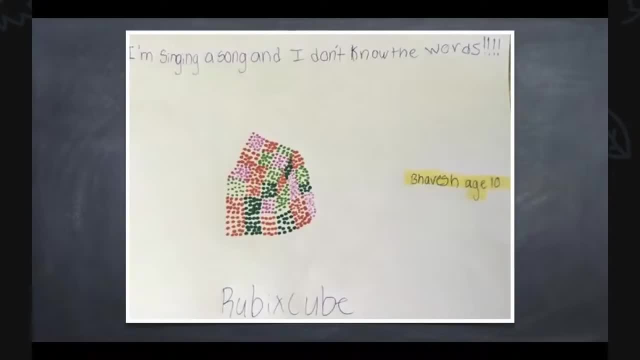 That's fantastic And you see, it's just dots arranged so that you get a picture. Yeah, yeah, The sun singing a song, The cool Rubik's Cube I love like you could actually see the 3D shape. That's not easy. 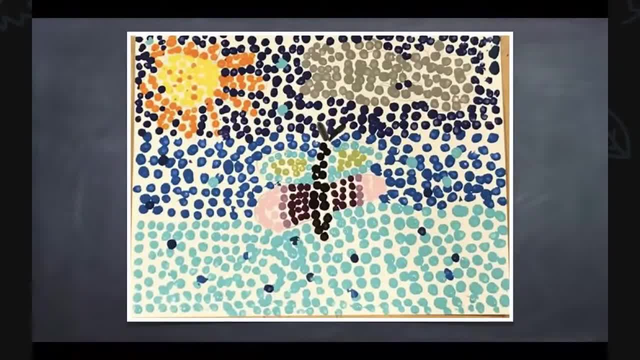 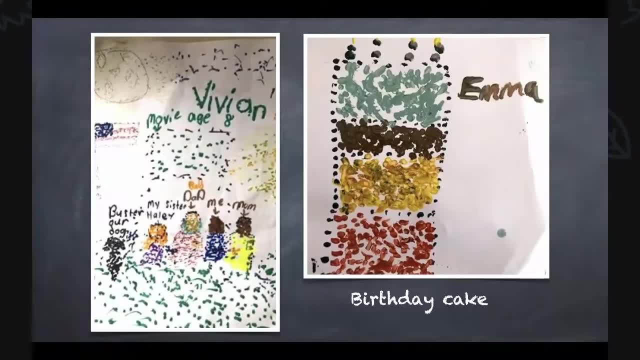 And then this one with paints: beautiful butterfly and a sun and a cloud and a scene. I like that. That's something really satisfying about It is the dots. Yeah, Seeing a picture emerge just from dots, Oh, great work. Vivian, portrait of her family and watching a movie. 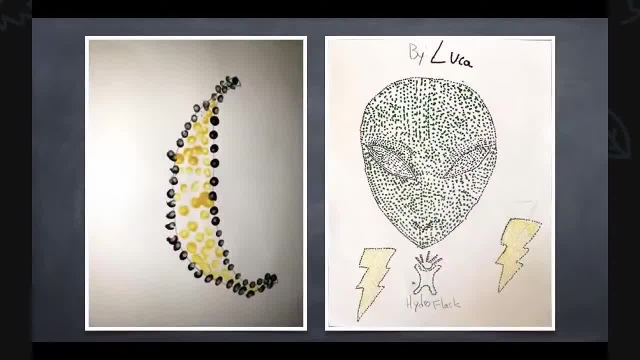 Emma drew a birthday cake. Ooh, Luca did this. cool. What is that? That was superheroes. That is that a superhero? I was going to say it was an alien, but awesome, And we've got a moon here. Well, the banana Jameson, Jameson. 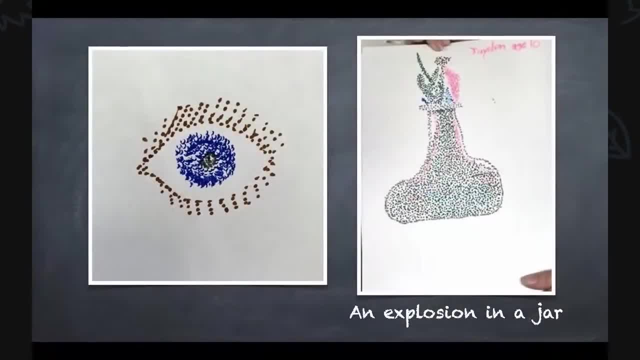 Yeah, nice great image of the sun. Ooh And I. is this how newspapers do their work? Little little tiny points of ink. You know it kind of is. Yeah Well, when you see, when you see a newspaper, if you get a magnifying glass and zoom in on a picture on the newspaper, you'll get down to just dots. 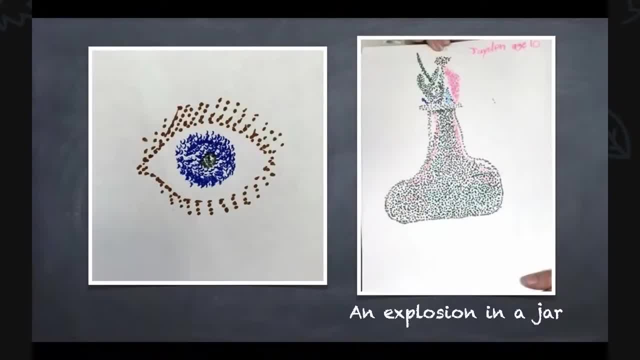 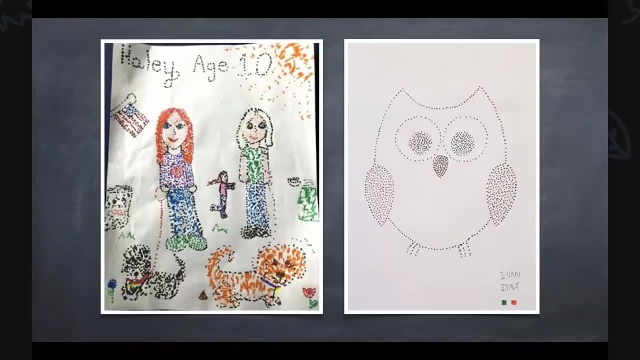 So in images you know pixels. That's really what pixels are. Pixels are dots. So great work, Jalynn. Explosion in a jar Haley- Oh nice work, I love it. And then look at, look at, the cute owl. 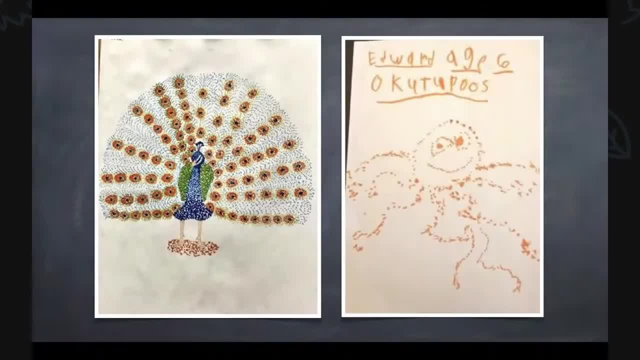 Oh yeah, good job, Ivan, Great job. The peacock is beautiful, Nicely done. Oh, and Edward, I love the octopus. It's fantastic. I couldn't draw this stuff with without using just points. You guys are doing a good job. Oh, and those are fun. So for people who haven't seen those, they're like a little like little plastic dots that you can put together and then you iron them and then they like merge together to create a painting And that's. that's exactly what this is. 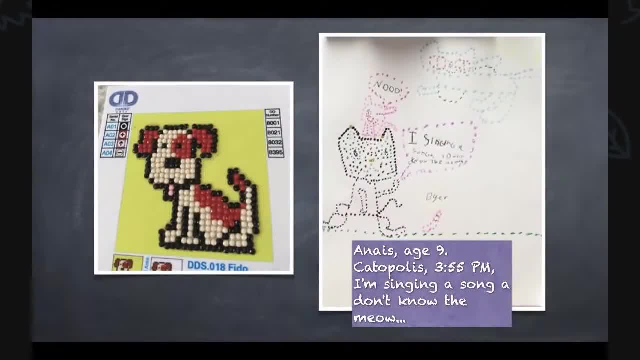 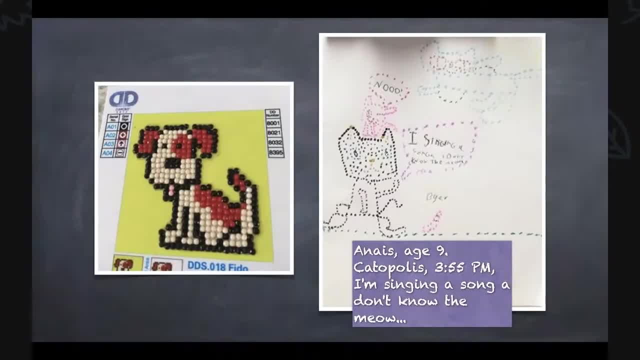 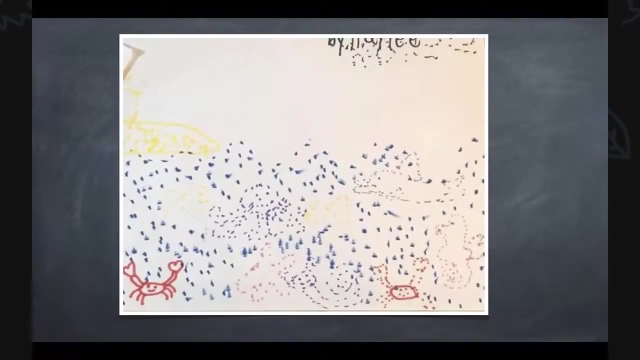 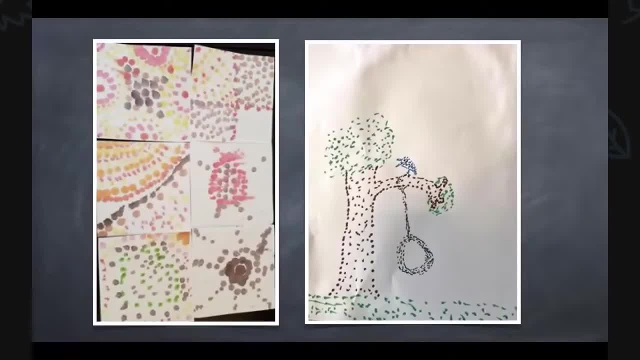 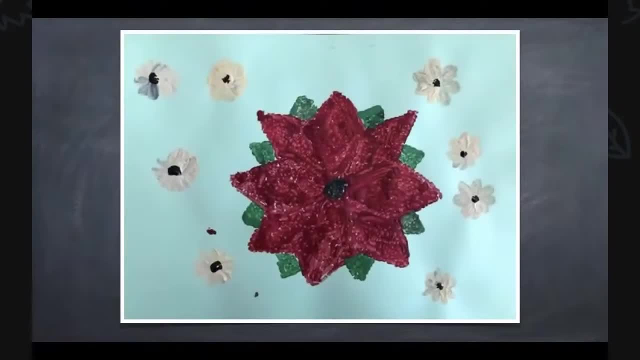 Is that Haley? I believe it's Haley- A little crab. They're super cute And we've got a bird and a tire swing. It's really fun to see the variety. Great job, you guys, with this art prompt. Ooh, a poinsettia and flowers. 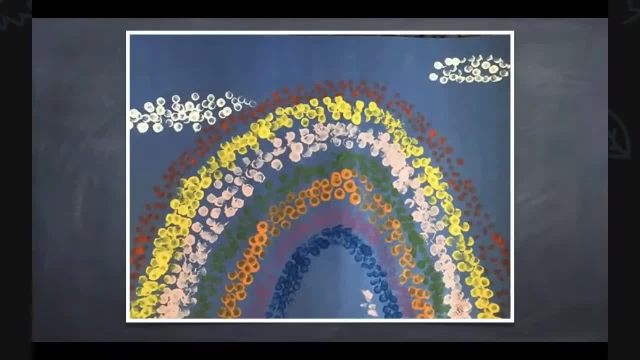 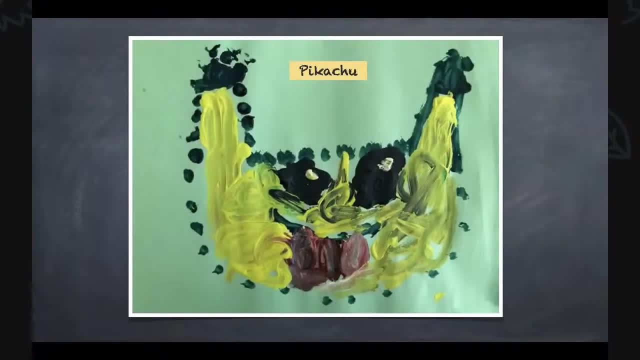 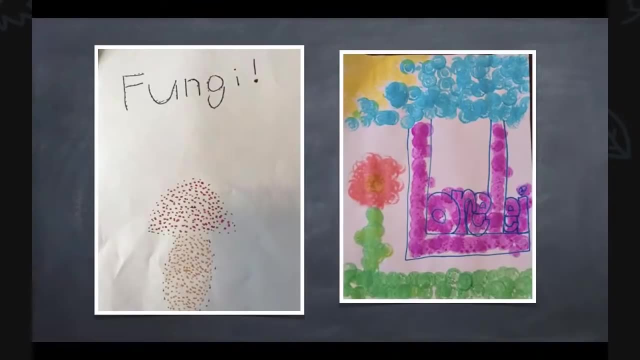 And we'll do three more. We've got a rainbow. Oh yeah, Lovely job. Oh, and a turtle Cute An ice cream cone, Popsicle pikachu, very nice, all right. and some fungi. and what's your name? yeah, very nice, you guys. 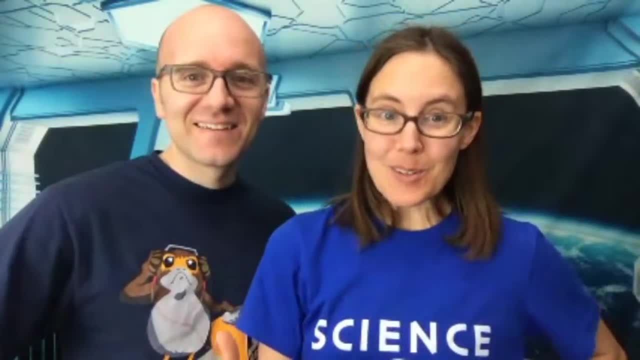 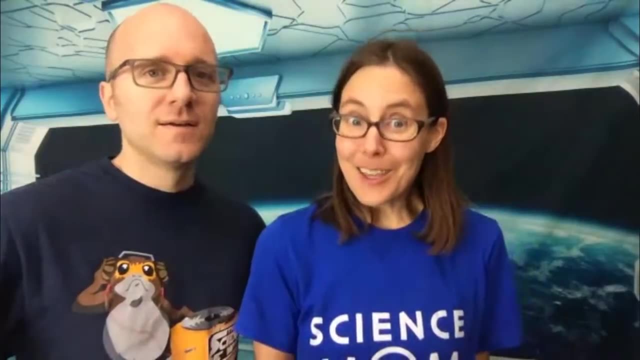 so thank you for everyone who sent in pictures with this pointillism art prompt. this was really a fun, fun activity, and if you're watching the replay and haven't had a chance to try it yet, give it a try and then share your art with us online so that we can see what you come up with. 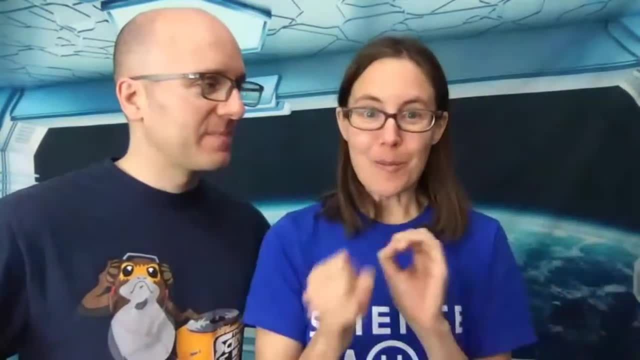 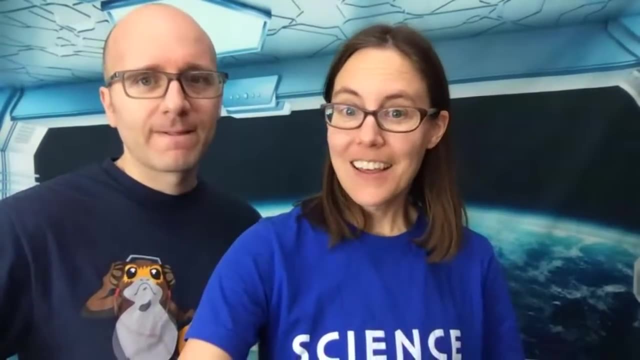 it's amazing to see, uh, an image emerge from just a collection of dots. i already forgot what's the art prompt for tomorrow: salt art, salt art, yes, salt art. so to create a salt painting with watercolor. and if you don't have watercolors, you can use. 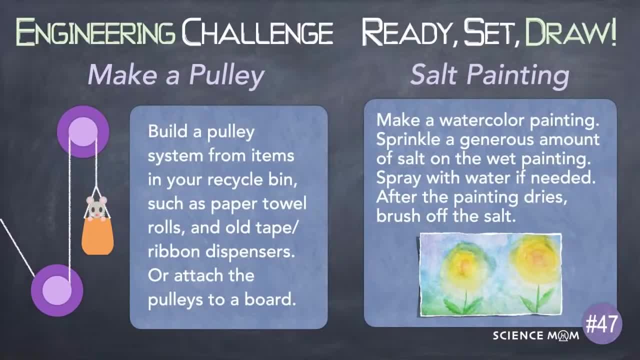 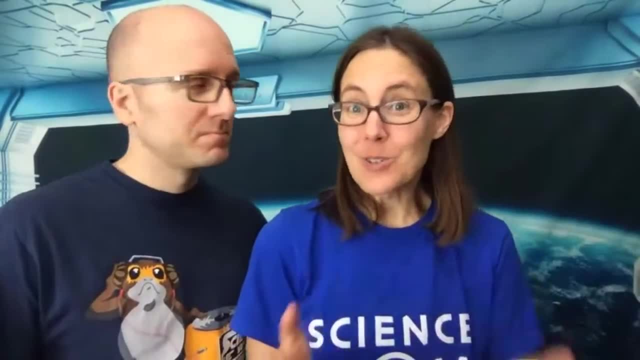 markers, and as long as the markers are washable markers, then when you spray them with water and salt, it'll work just the same way. so that's a that's a good little life hack. if you ever want to do watercolors and you don't have watercolors, just take washable markers, color and then a squirt. 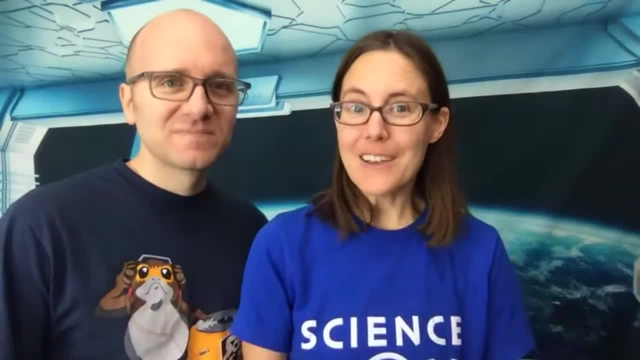 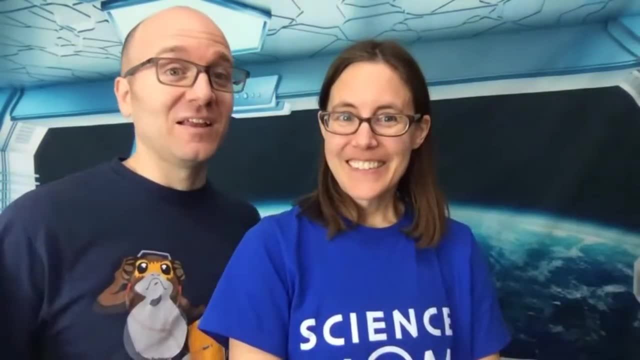 bottle or you know, maybe just mist with like flicking water on it and add, install. it'll work much the same way. cool, all right. thank you so much for tuning in today and in having fun with us playing with some levers and pulleys, these simple machines, mechanical. 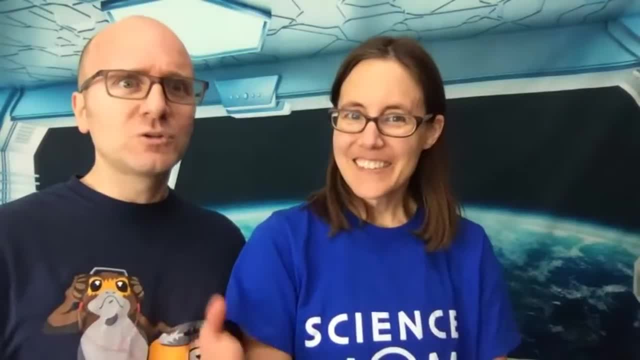 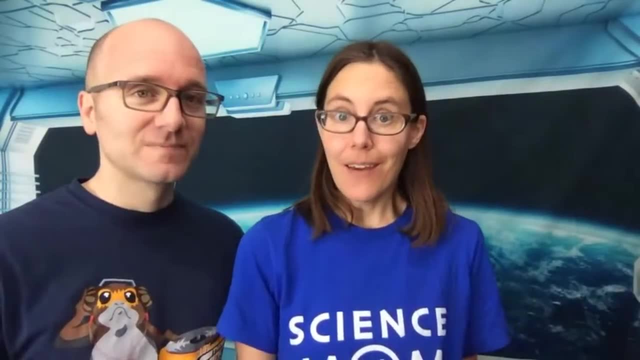 advantage are absolutely fascinating and a huge part of our lives, even though we might not realize it. yes, and tomorrow we're going to be learning all about indoor plumbing and water. how do we get clean water and, maybe more importantly, where does all the stuff we flush down the toilet go?